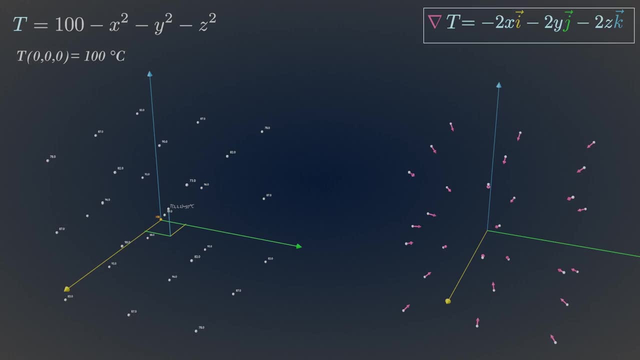 If you remember from calculus 2,, a gradient vector always has a vector function. This vector points towards maximum increase or decrease of a function. Looking at this gradient field at each point in the region, it gives the direction for which the increase in temperature is greatest. 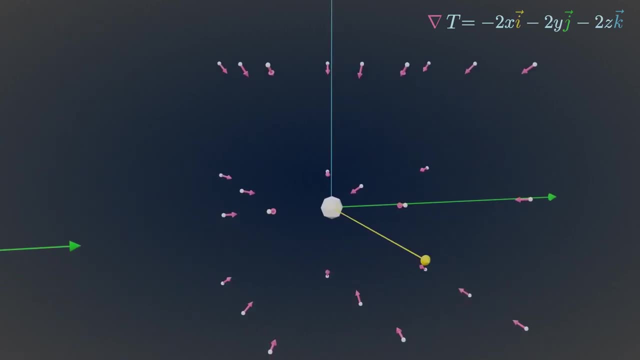 In this case the vectors are pointing towards origin. If you notice, only on origin the temperature is maximum, So the temperature gradient at origin is zero. you can verify this by looking at the scalar field. before we move more intuitive meaning towards gradients, notice the difference between scalar and vector field we would encounter. 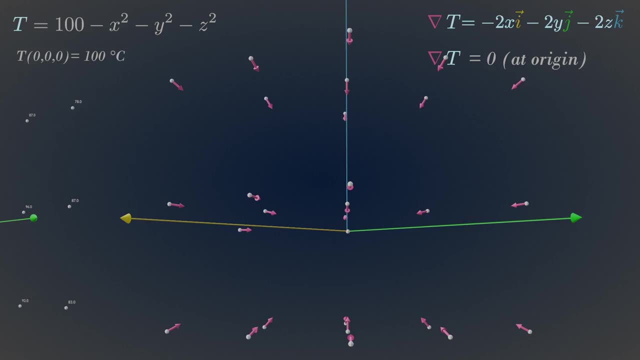 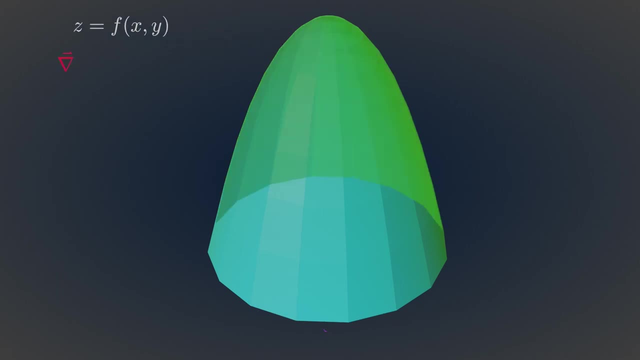 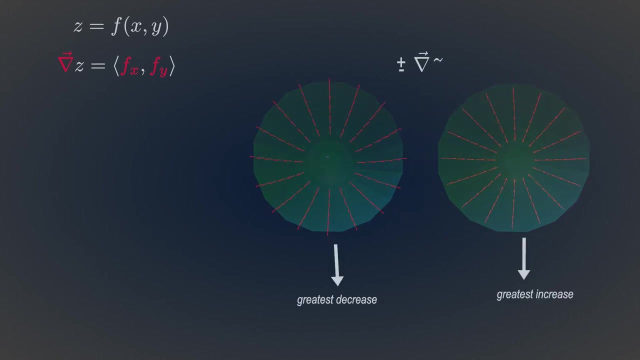 a lot of vector fields in this course. here i have plotted a scalar function in space. gradient of a scalar function is a vector that always points in the direction of greatest increase or decrease of the function at a point. the gradient operator here captures all the partial derivative information of a function. 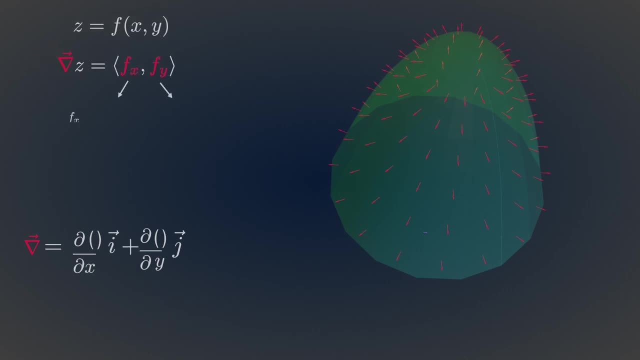 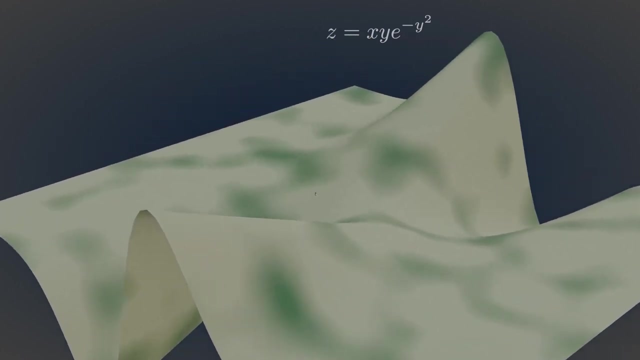 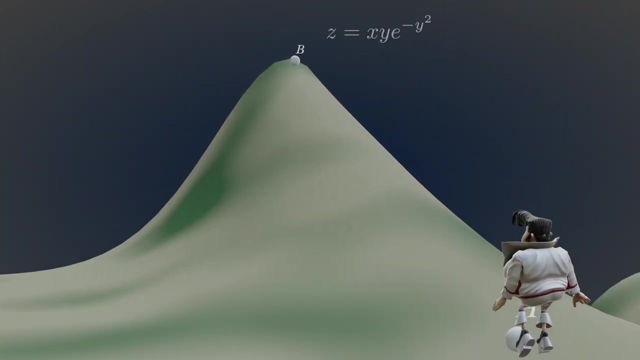 adds them and makes them a vector. let's get in depth of it. let's get in depth of it. okay, here is a function of two variable which i have plotted. it creates a hill in 3d space. now here is a boy standing at point a. now he wants to climb the hill and move towards. 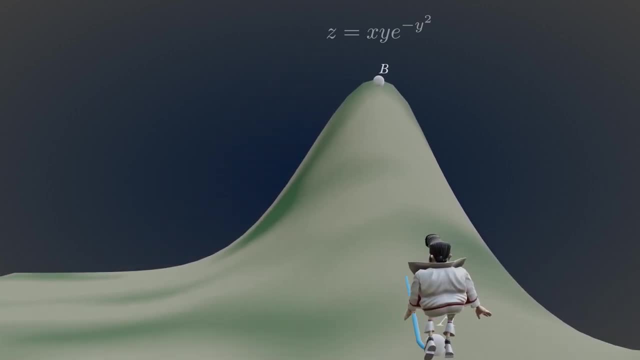 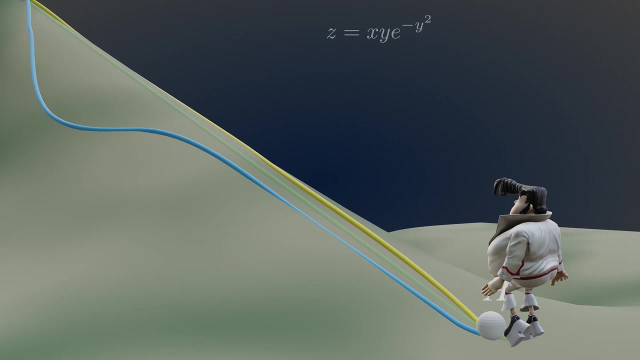 point b. he knows that he can climb the hill in many ways and can follow different curved path, but also he wanted to climb faster. so right now he is in search of a way to climb the hill, in search of the path that has the steepest ascent. 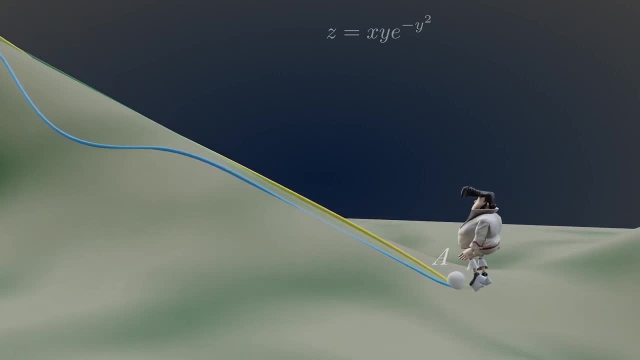 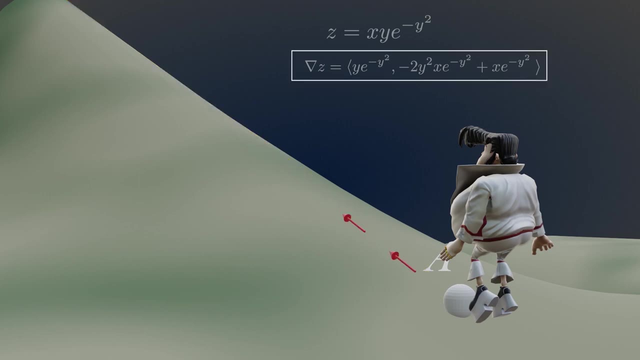 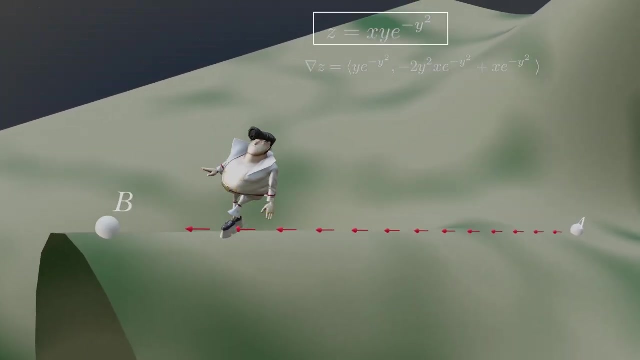 do you have any idea from a to b? how can he get the direction to steepest path? well, he can use gradient. it can shows him the path of steepest ascent of a hill. by using his position coordinates he can generate gradient vectors. the gradient of this to variable. 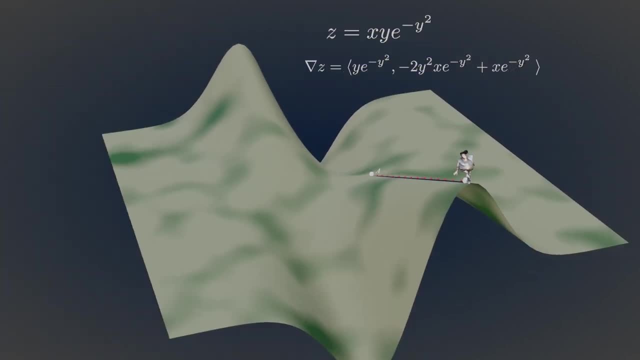 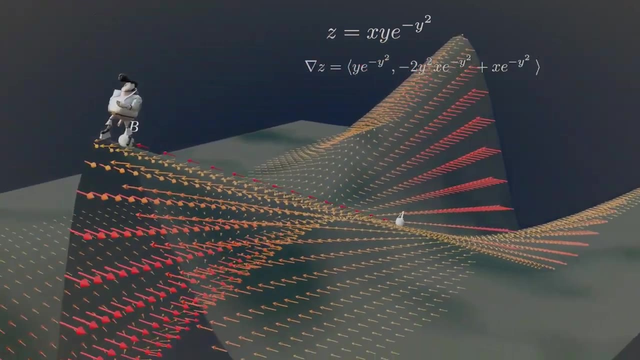 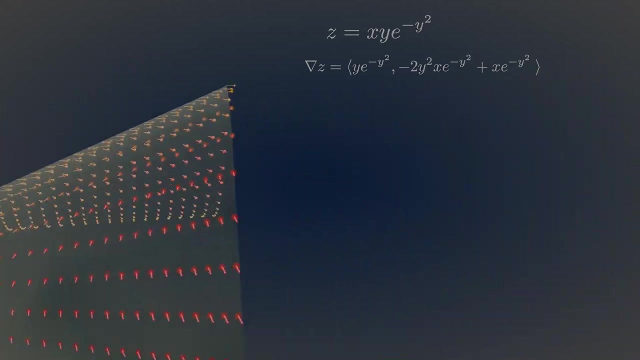 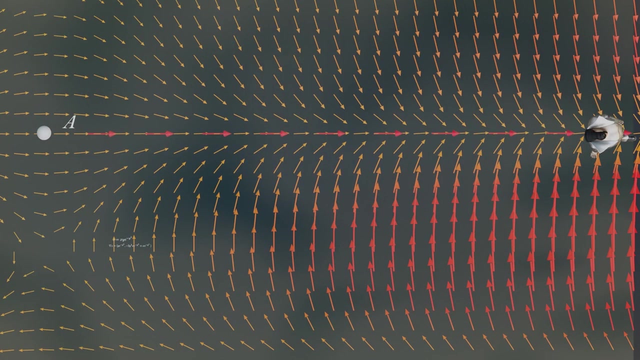 function is this to the vector field. the gradient of this to variable function is this to the vector field. for this we need to use gradient gradients to make a gradient. and since gradient gradients have been added on theác będziemy, let's plot this gradient field on every coordinates of our hills. these gradient vectors doesn't make any sense right now. well, these gradients vectors are second dimensional and makes much sense when you look them with the top view. this is the path taken by a boy looking at this field graph. you can see everywhere in hills coordinate. the gradient vector points to the hill. we see here are many gradients and we can see whole mountains. but heresi were next to the hill. we don't have many gradients and if we you forgot some graph, you'll not were where there are some Increvidae and another gradient field in the Nitrogen field. We'd looks like a bad cartoon. Don't forget that gradient vectors can be created manually. you only haven't enough time to understand the Australia low energy and water levels. 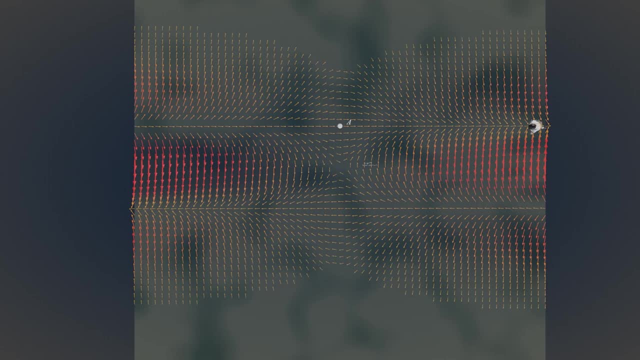 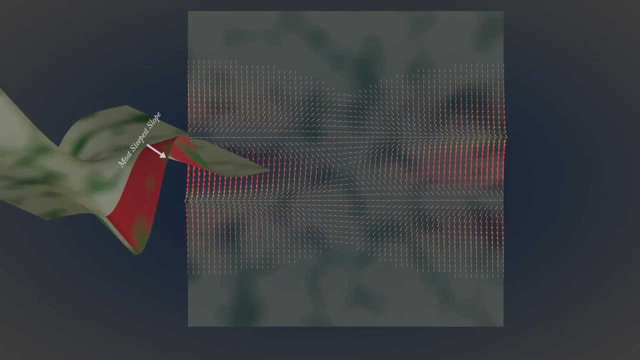 vector points towards the path of steepest ascent. Here the gradient arrows are red in color and have larger magnitude. It means that this area got the highest steepest slope. Also, notice: here is no gradient. the slope is zero, which means the ground is completely flat. 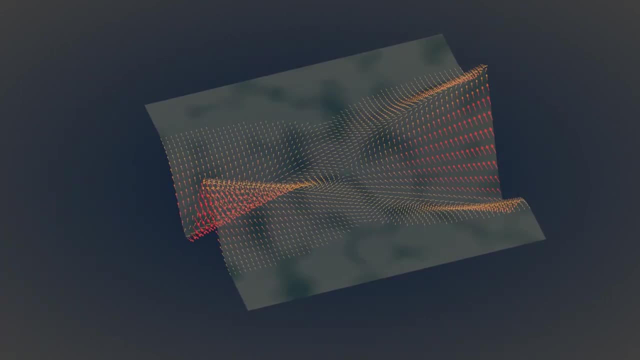 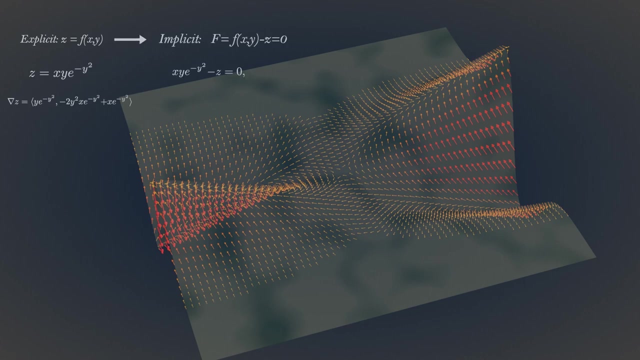 So we calculated gradient of this explicit function, But you can convert it to implicit function and calculate its gradient. This time it gives you gradient in three dimensions. If you plot this gradient, all you will get is a normal vectors of the surfaces. 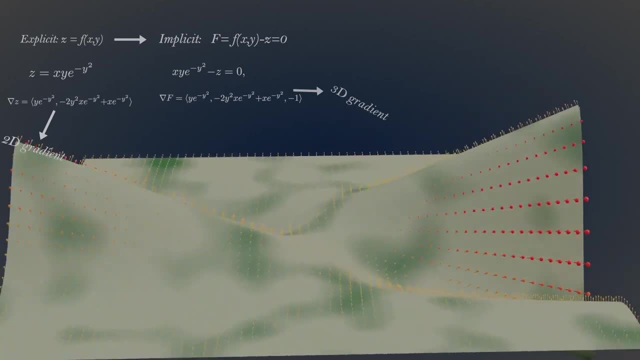 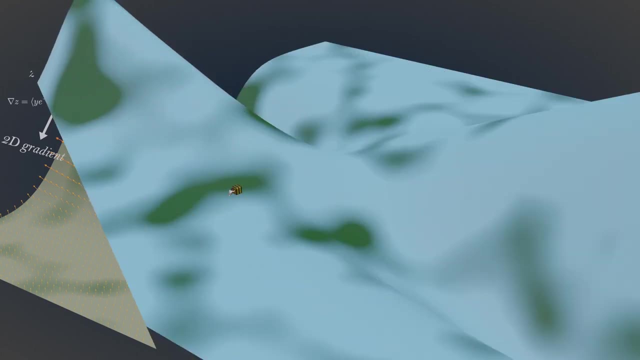 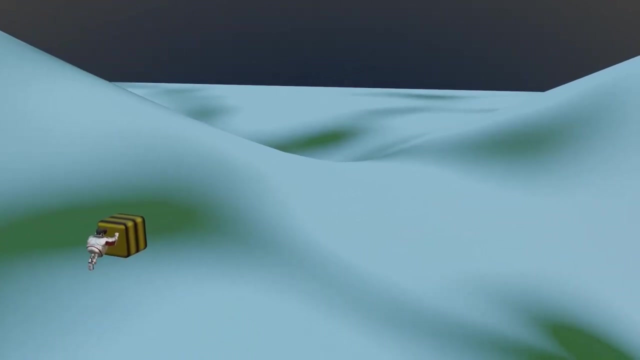 These vectors are important in surface parametrizations. We will talk more about this in the next video. We will talk more about it later in more detailed concept. Now let's get the idea of line integral of a vector field. Here you can see a boy is trying to push the block along the curve. 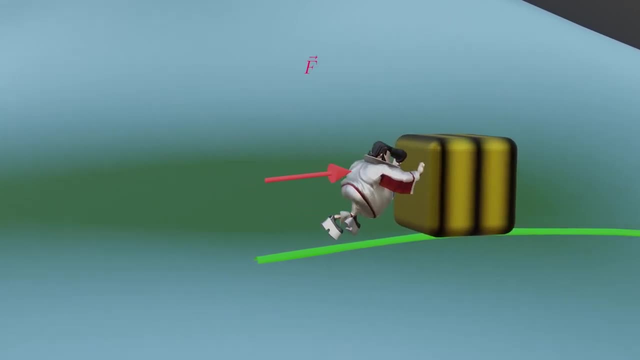 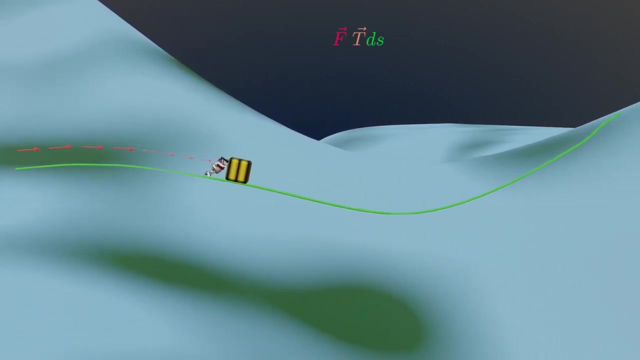 For that he needs to apply force and push it in certain direction. If you notice, this block will only move along the path of curve if he apply force tangent to curve direction. In some cases he needs to apply less force to push it, while in some cases he needs to apply more force. 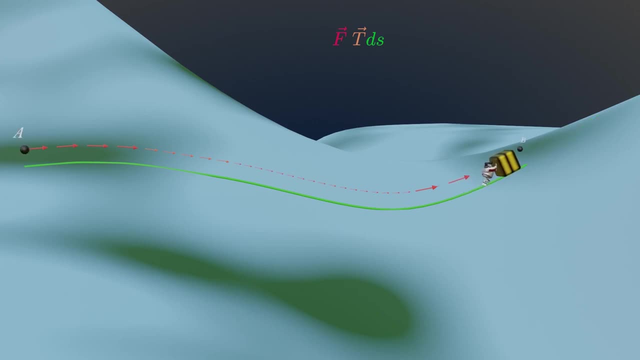 If he successfully move the block from point A to point B, then he has done work on it. This work done is calculated by summing up all the magnitude of tangent forces along the length of curve. This summation is done by line integral. 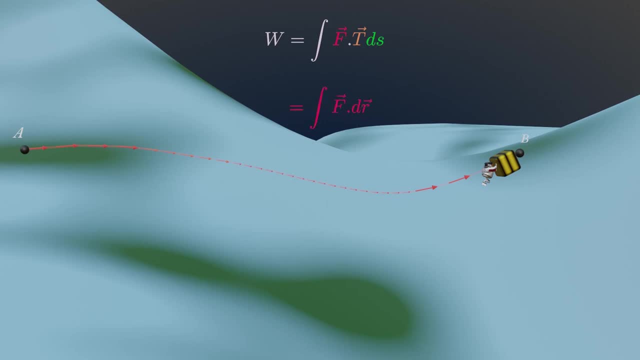 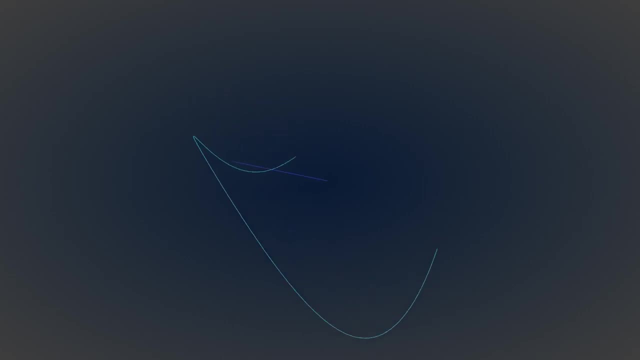 It can also be written in more standard form. As a particle moves along a smooth curve in space, the unit tangent vector turns as the curve bends. Its length remains constant and only its direction changes. The unit tangent vector is given by: 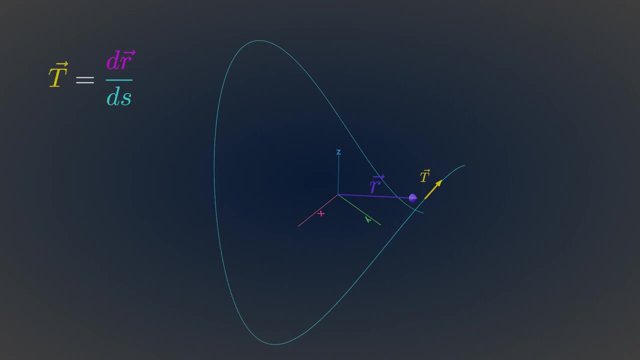 This can be simplified as: Therefore, the simple definition of work done is given by unit tangent vector. As a particle moves along a smooth curve in space, the unit tangent vector turns as the curve bends. The result is transformational. 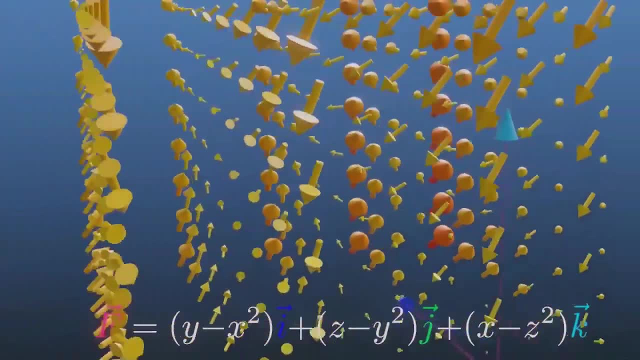 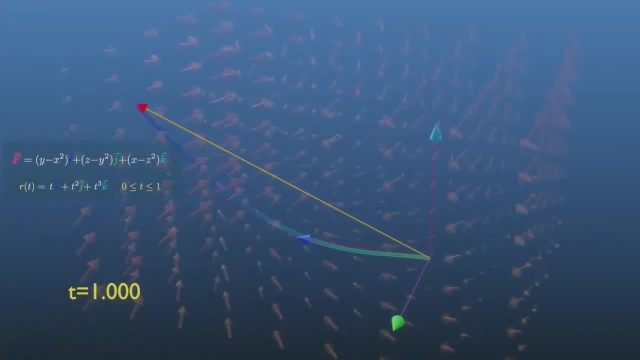 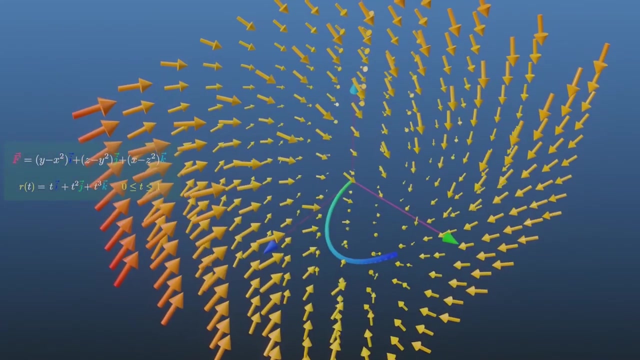 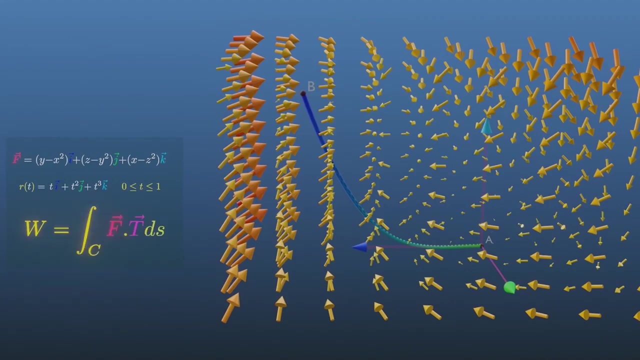 Okay, let's visualize work done by this force field on moving an object along the curve parametrized by this equation. The formula to calculate the total work done in moving an object from point A to point B is this line integral. Here, F is the force vector of the field, T is unit tangent. 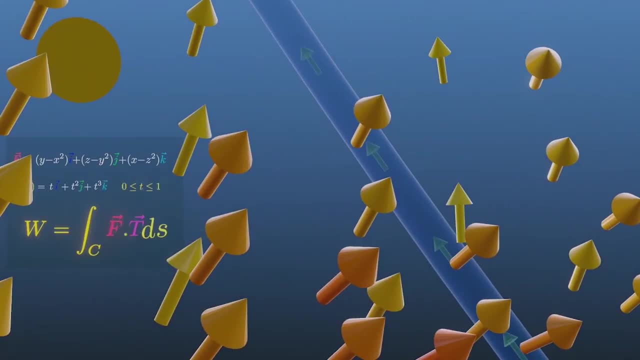 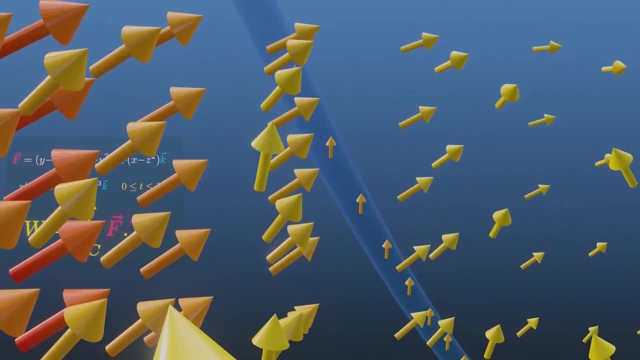 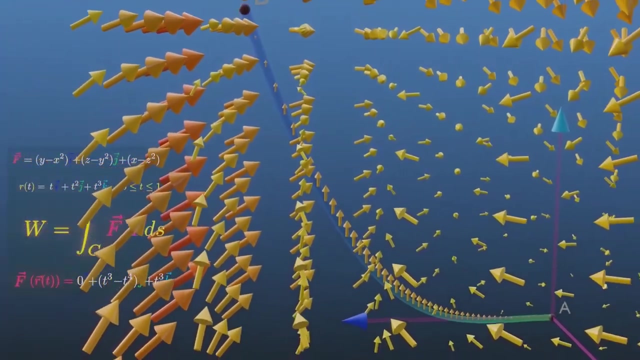 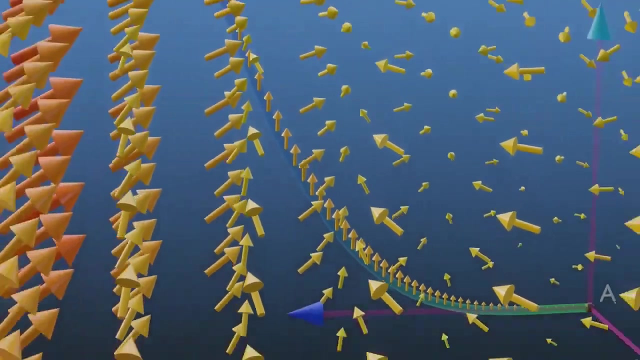 vector of curve and ds is arc length. Okay, now we need to calculate the force vectors acting on every point of the curve. So let's evaluate the force field only on curve. Notice how its magnitude is randomly distributed along the length of curve. 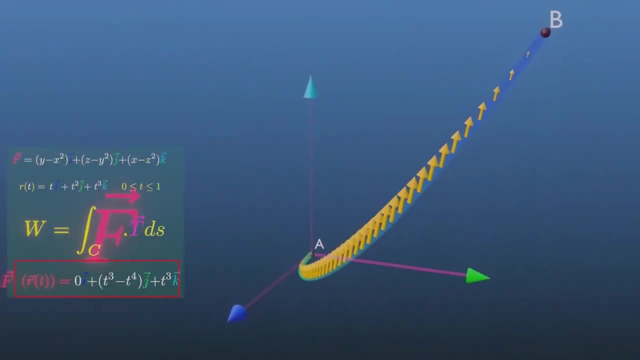 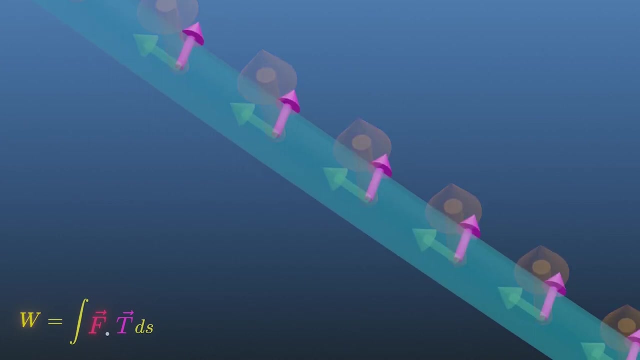 Right now. we don't want all the force field. Evaluating force field only on the curve points is enough. Every curve is oriented in space according to their unit's tangent vectors and normal vectors. To calculate work done, we only need tangential vectors of curve. 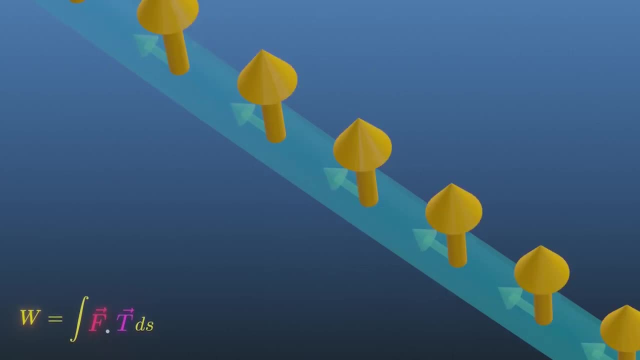 We can calculate in what direction those unit's tangent vectors are pointing just by differentiating this parametrized curve. This is simple dot product and it is scalar quantity. Here we are projecting every force vectors in the direction of unit's tangent vector of curve. 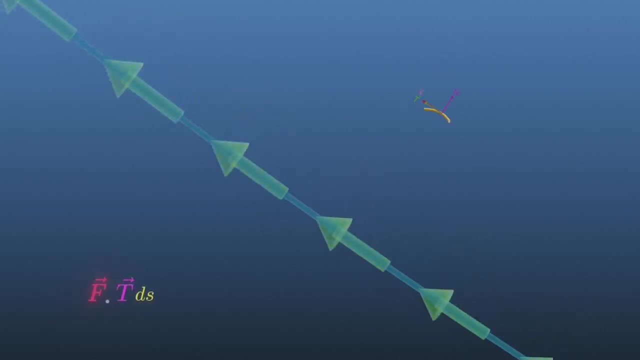 and multiplying the magnitude of this tangential component of force with the small arc length of curve, This gives small work done on infinitesimal arc length. To calculate the total work done, we need to sum up every tangential component of force field along the length of curve. 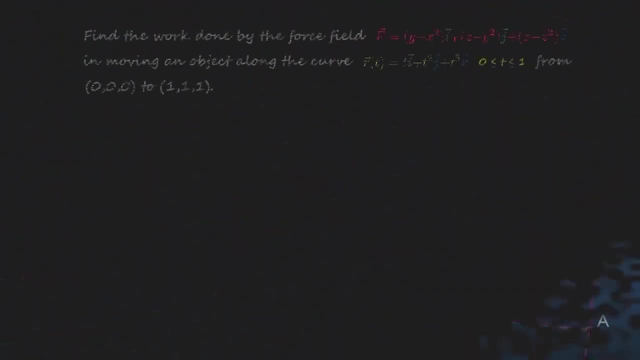 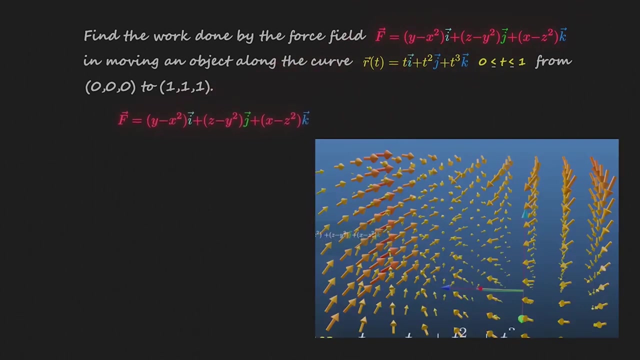 This is possible only by using integration. Okay, that's some intuitive definition of work done by force field. Now let's look at another example. First, let's get our vector field and parametrized curve, Calculate the force field acting only on curve. 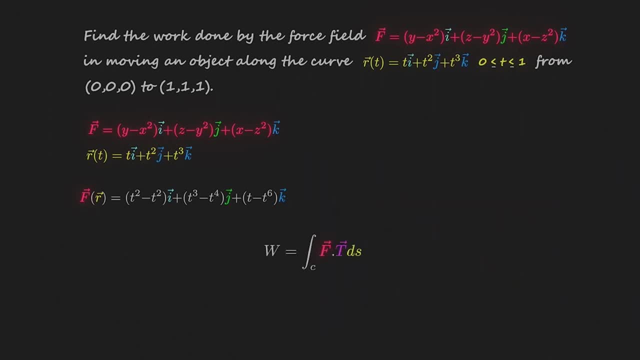 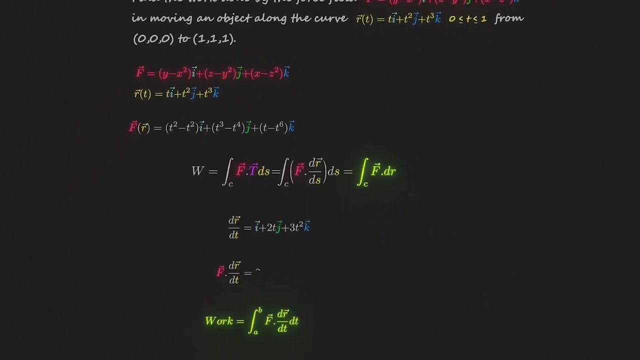 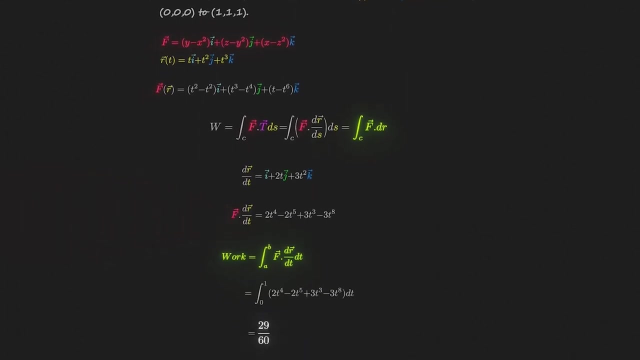 Now the definition of work done is: We can convert this equation into parametric vector form. I already told you the relation of these three parameters. Now you can easily calculate total work done by simply using this formula. Just calculate the dot product and integrate from: t equals 0 to 1.. 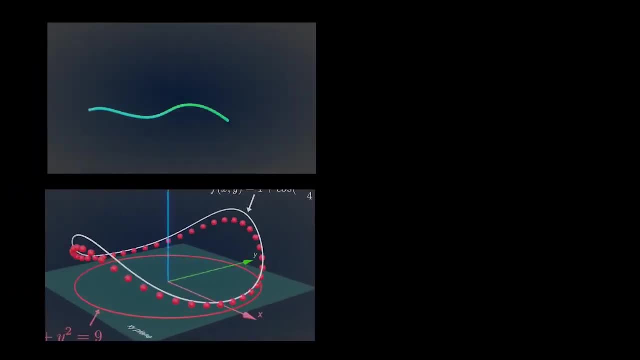 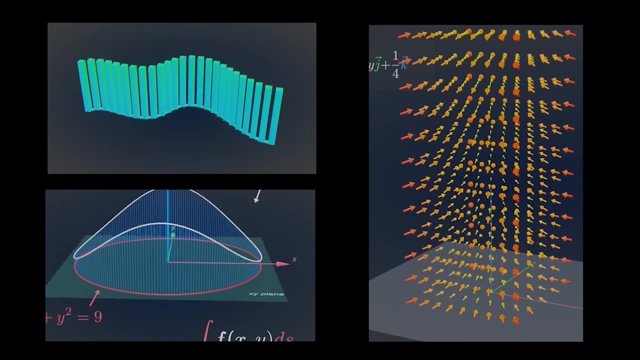 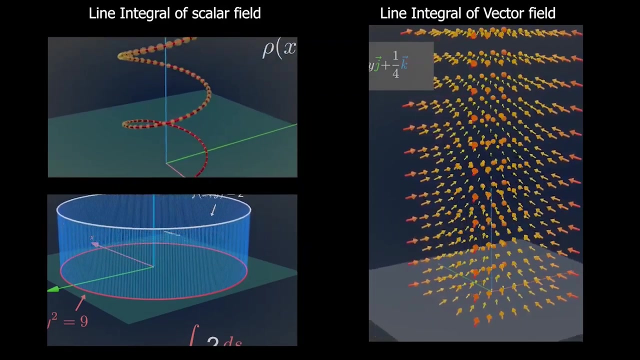 Okay, work done was an example of line integral of a vector field. Throughout this course, you would encounter two types of line integrals: Line integrals of scalar fields and line integrals of a vector field. Now let's take a look at the line integral of a scalar field. 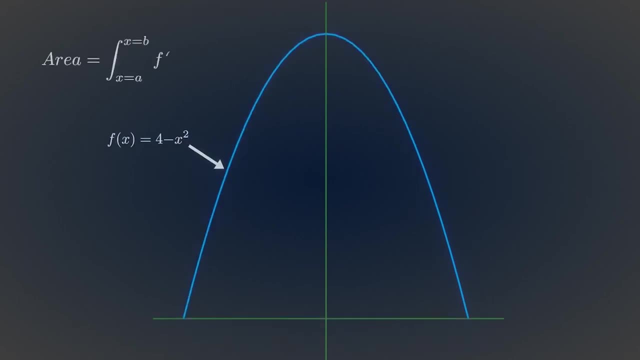 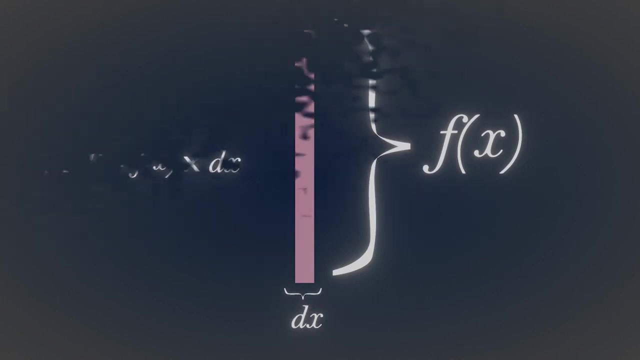 To understand line integral, let's understand the basic idea of simple integral first. For that I would use a rectangle that has an infinitesimal width and posses some height to get intuitive meaning of scalar line integral. Consider an equation of a curve: The integral of this curve with respect to x-axis. 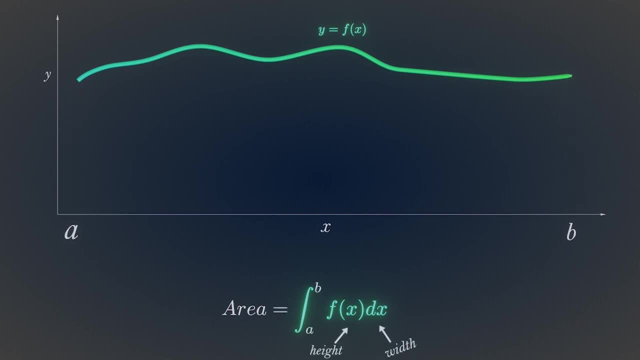 is given by this formula. It got variable height and infinitesimal width of a small rectangle. Let's call it a stick. Right now we only got four stick. Let's keep on adding them. If you do so, you approximate the area under this curve. 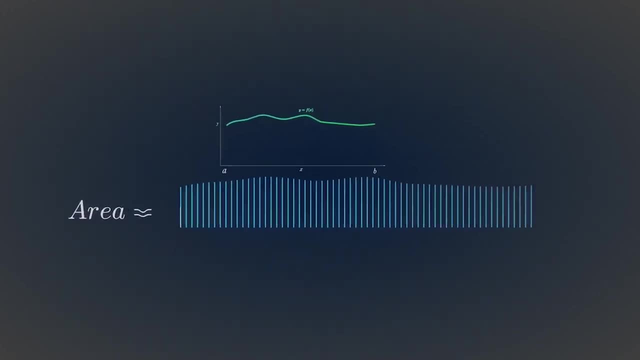 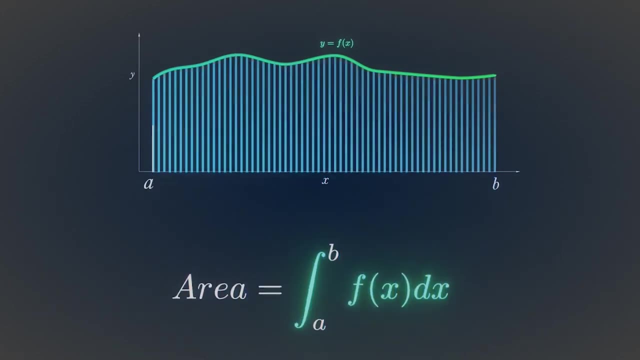 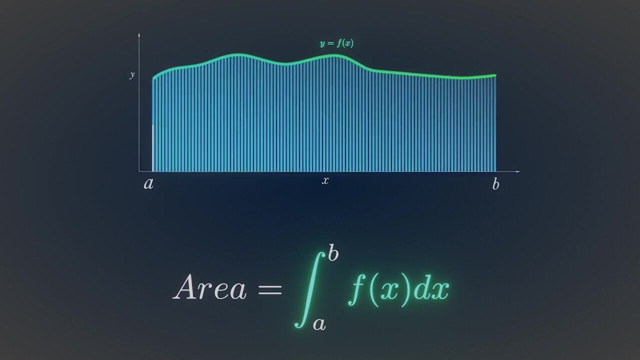 Just by using 63 sticks you can easily approximate the area. The area would be more precise if our stick possesses infinitesimal width and we increase the number of sticks. This is also one kind of line integral. Here we integrate the curve with respect to x-axis. 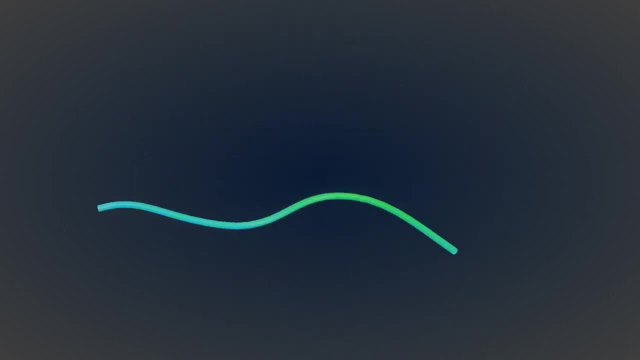 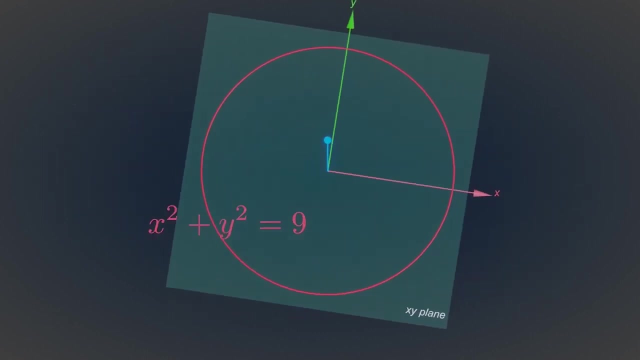 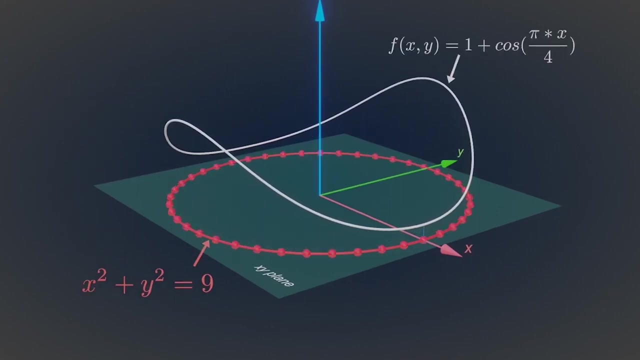 Now let's try to add those sticks on a 2D curve and try to integrate them. Here is a parametrized equation of a circle in x-y plane. Now let's plot another curve orthogonal to this circle. Here every point of this circle is projected upward, which builds this beautiful function. 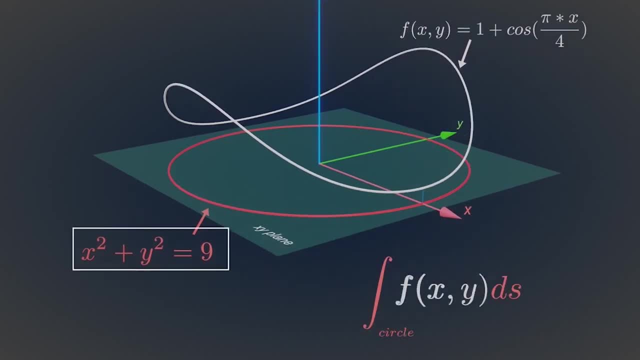 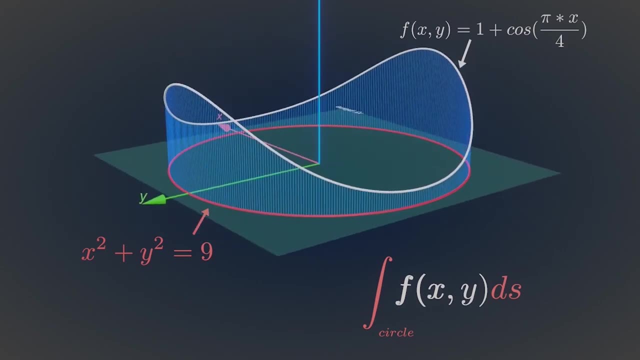 The line integral of this function along the curve gives the area of this blue surface. Just imagine adding those tiny stick along the path of a circle. Now here is an interesting thing: Decent value If you change this formula's height function to some constant value. let's make it 1,. 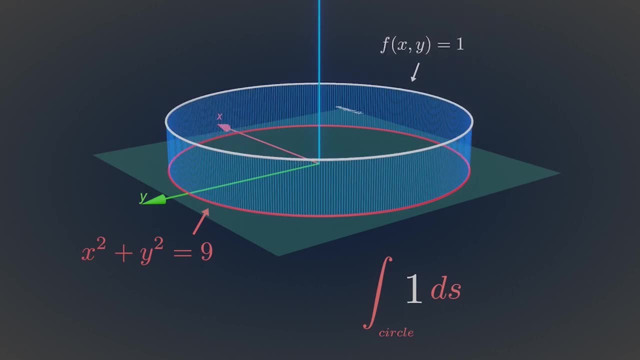 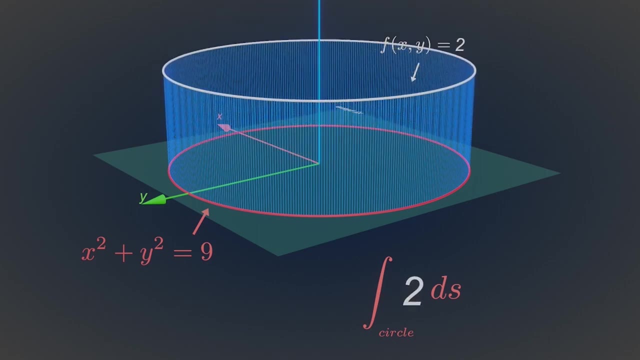 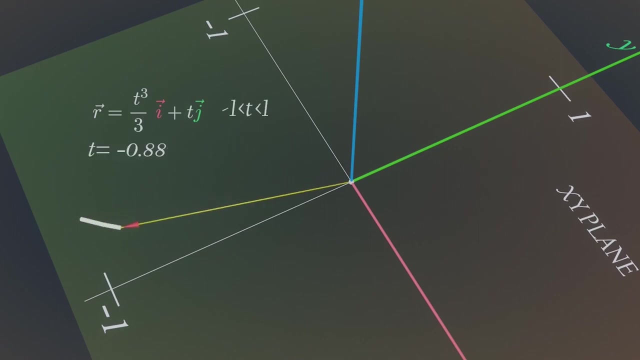 then you will get the Area of this cylinder. In this case every stick got the height one. Its height is directly proportional to the magnitude of this constant. Okay, here is another curve parametrized in x-y plane. So here in a circle we have a til QUEEN weaving arrangement in x-lineatur, root of x-hao condition. 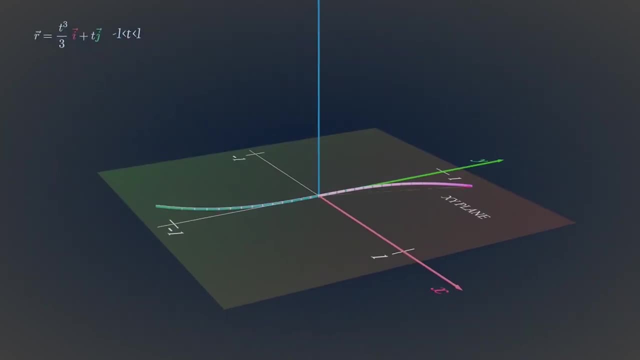 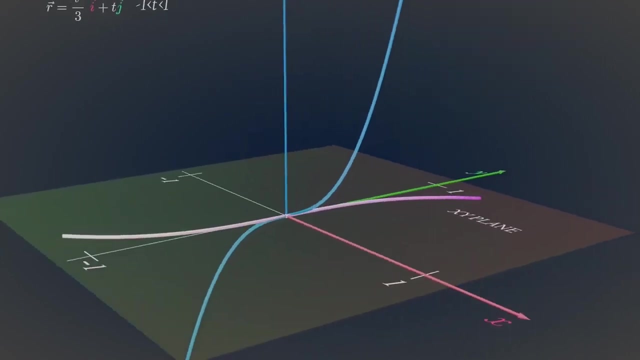 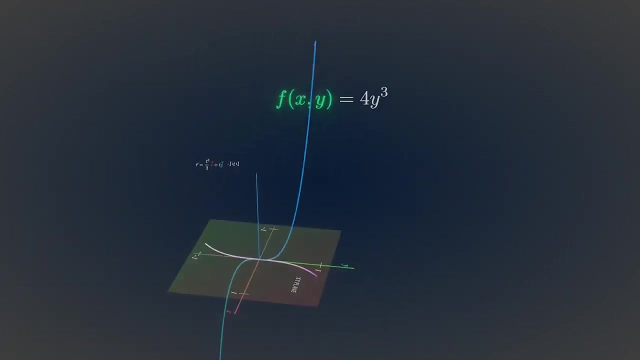 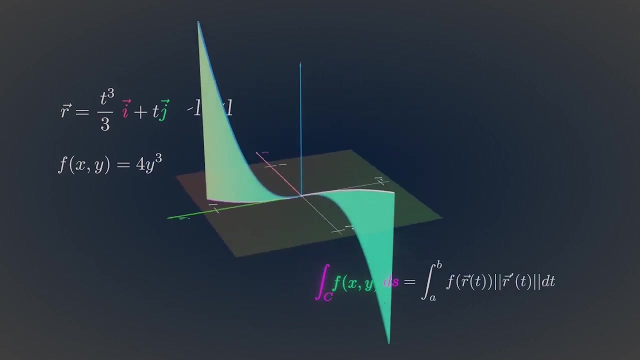 Now here is an interesting thing Again. let's draw another curve orthogonal to this parametrized curve. See how this curve is parametrized. The line integral of this function, where we add tiny sticks along the parametrized curve in x-y plane, gives the area of this surface. 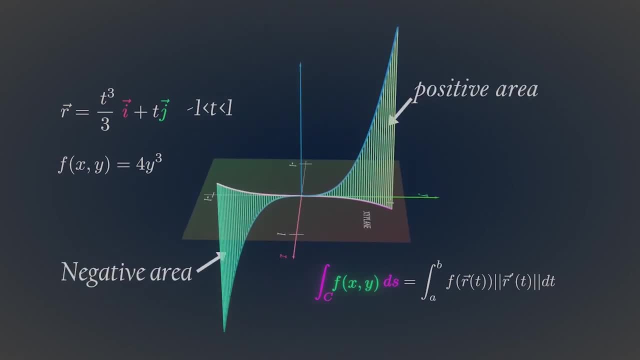 Please be careful with the negative area. From the illustration we see that the graph dips below the x-y plane. There is technique to calculate area back in single variable calculus to handle this type of negative and positive function. Now here is an another example: a parametrized ellipse in x-y plane. 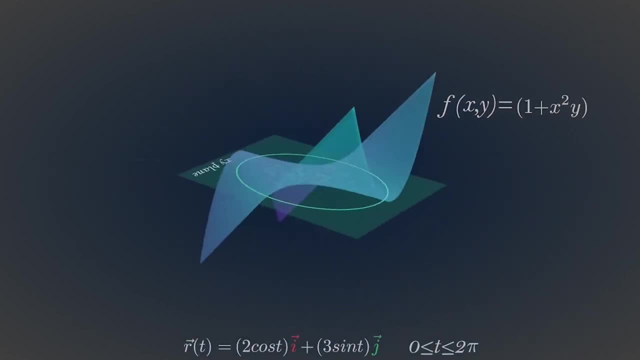 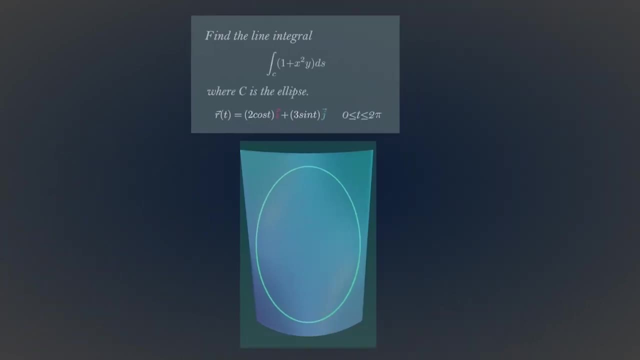 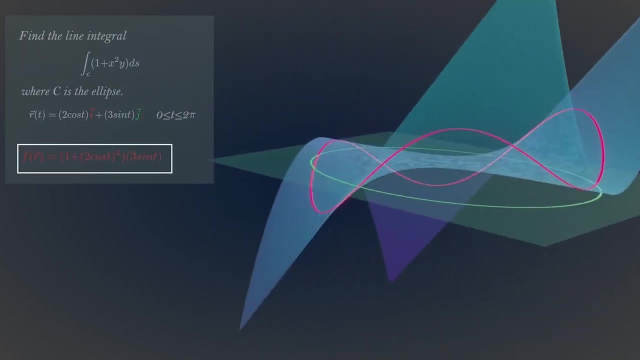 This time let's draw a surface that surrounds this ellipse. As you can see, this surface surrounds our ellipse in all way. Let's try to solve this line integral problem. First, we need to project our ellipse over the surface. Now the height of stick is given by this parametrized function. 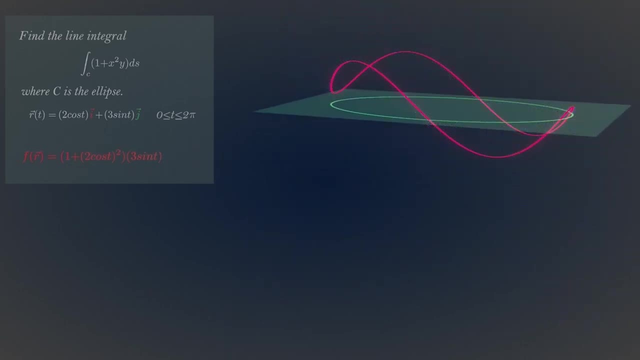 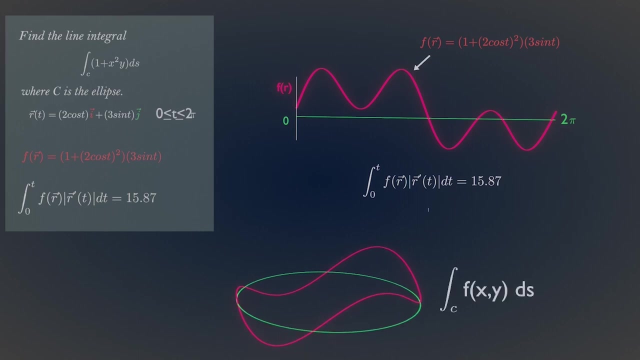 Now we don't want the surface, Let's remove it. Evaluating this line integral is like adding stick along the path of ellipse that has height generated by this parametrized function. You can convert this problem into this: Did you notice how important parametrizing a curve is? 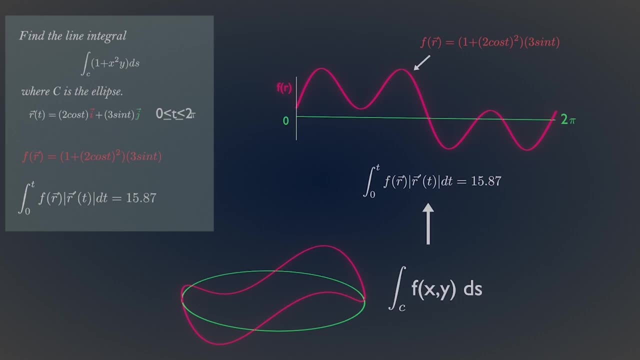 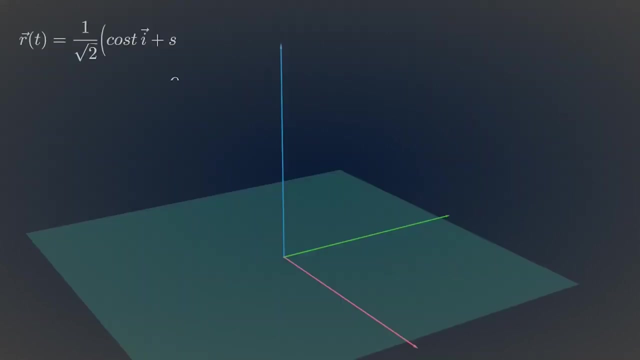 It just makes integral more easier to compute. It just makes integral more easier to compute Here. notice the negative area. Be sure to take it into account while calculating the area under this graph Line. integral of scalar function along a curve in space is just not clear. what such 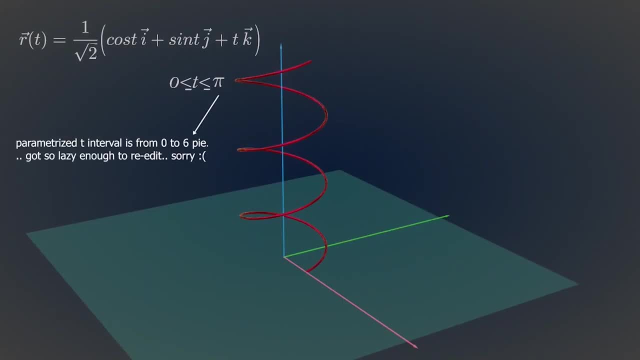 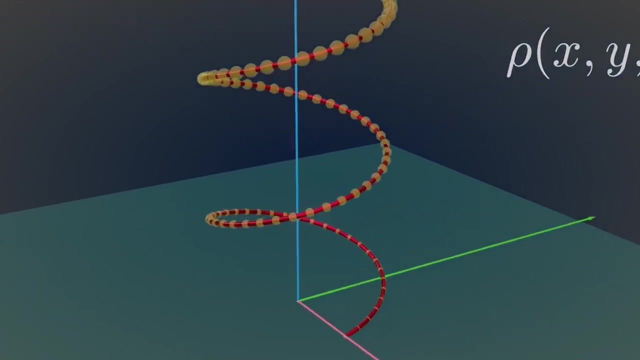 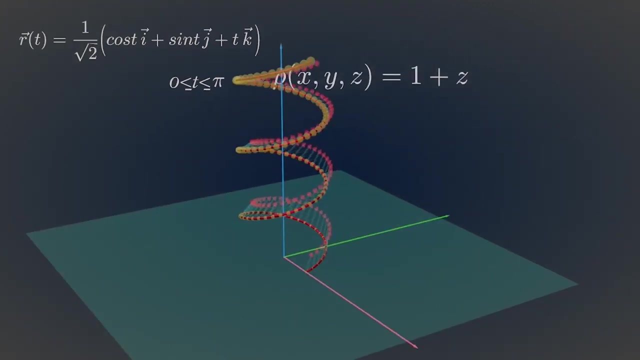 an integral mean, But they are good for more than just computing areas. Consider this spiral curve as a spring. Let's say the density of this spring varies in space according to this Scalar function. Just notice that the density of this spring increases as the spring spirals up the z-axis. 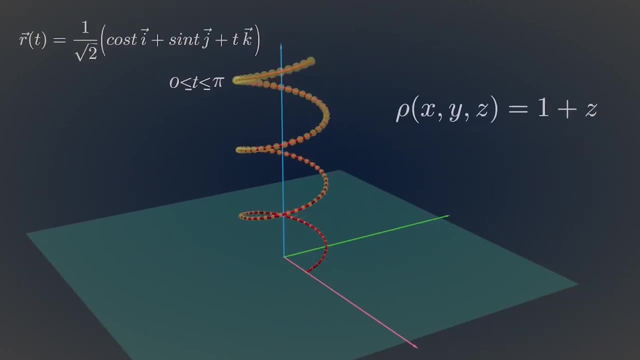 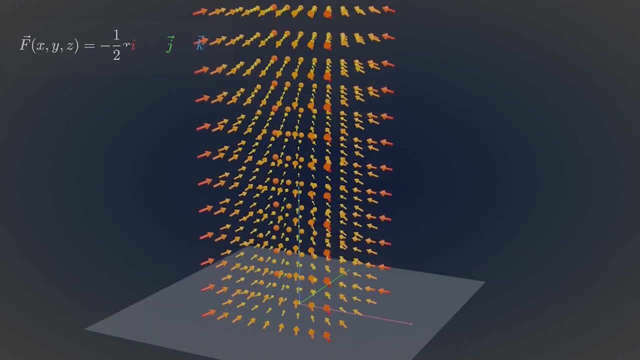 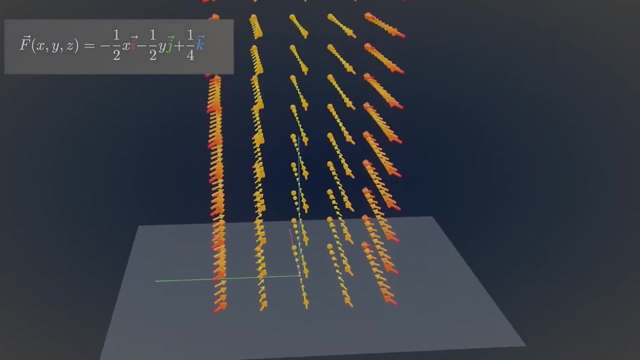 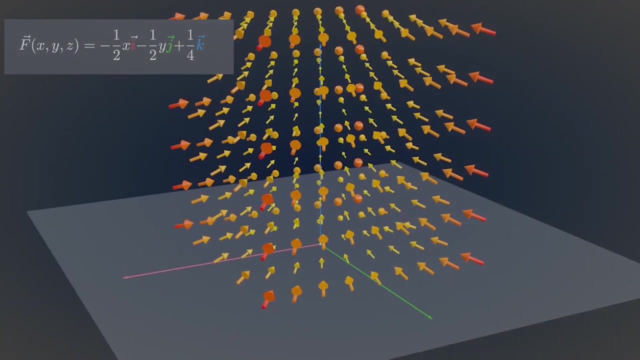 If this density function is mass per unit length, then the mass can be calculated by using this formula. Okay, that was some simple example of line integral of scalar fields. Let's get our attention back to the vector field. Throughout this course we would mostly focus on a vector fields. 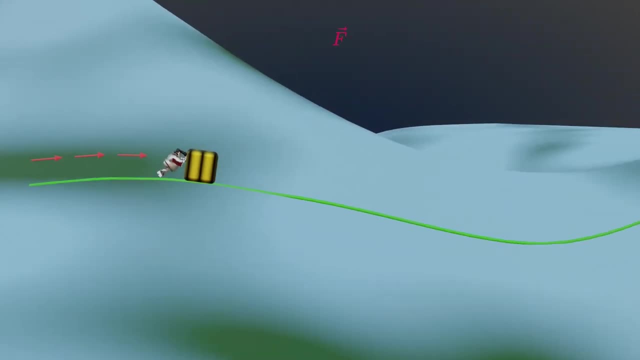 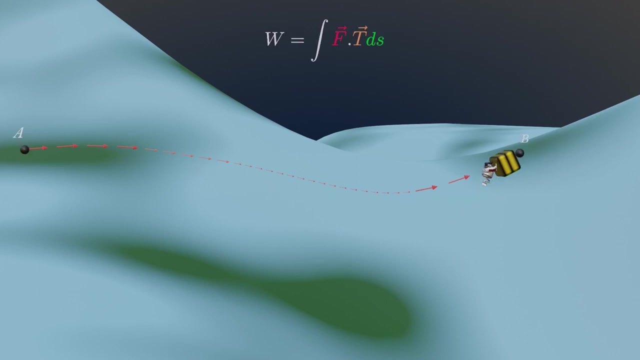 As you have seen, if you integrate the force vectors along the length of curve, you will obtain the total work done. But what if you integrate velocity vectors along the same curve? In the next section we will deal with line integral of velocity fields. 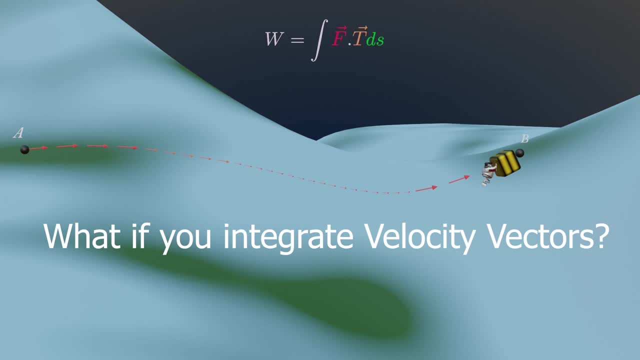 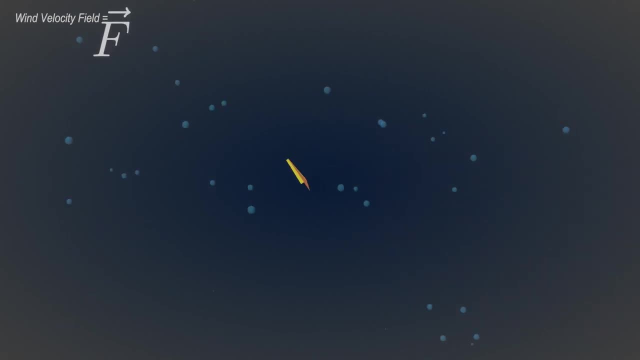 This brings the new concept of flow and circulation. Now consider a velocity field of vaned vectors. In this velocity field, a plane is flying up in the sky Let's its position in space is given by this position vector. 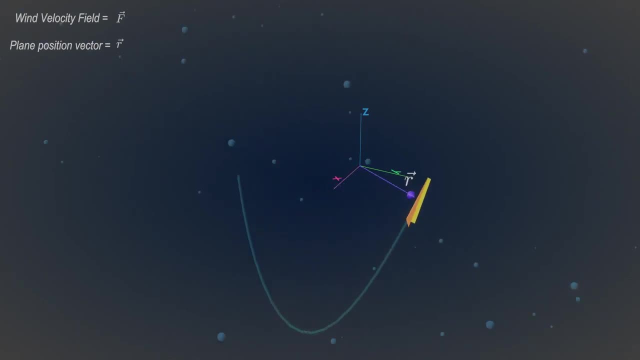 Let's consider a velocity field of vaned vectors. In this velocity field, a plane is flying up in the sky. Plotting it, you can see our plane is following a path of a closed curve in 3D space. You can calculate the velocity of this plane by differentiating this position vector. 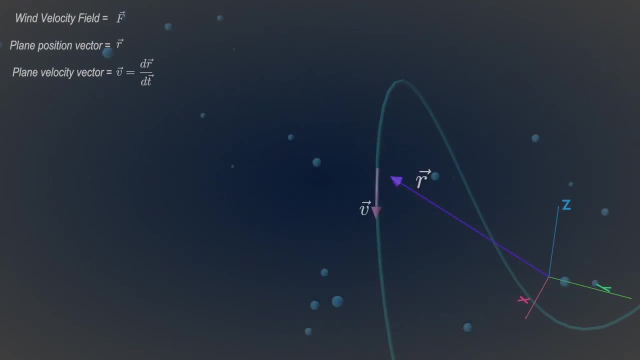 This velocity vector of plane would be tangent to curve. Notice, there are two velocity vectors. One, velocity vectors of vaned, Another, velocity of the plane. Let's consider a velocity field of vaned vectors. This velocity vector of plane would be tangent to curve. 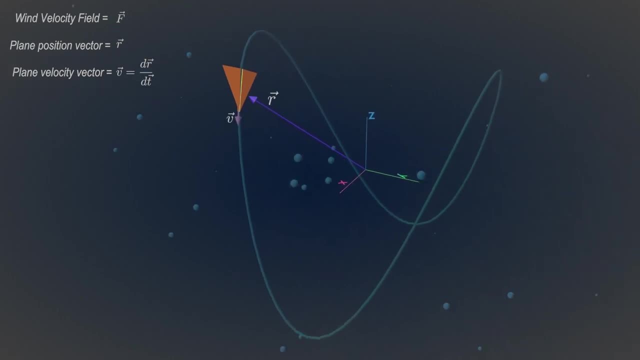 Notice there are two velocity vectors of vaned vectors. One velocity vector of plane would be tangent to curve. Notice there are two velocity vectors of vaned vectors. This velocity vector of plane would be tangent to curve. Notice there are two velocity vectors of vaned vectors. 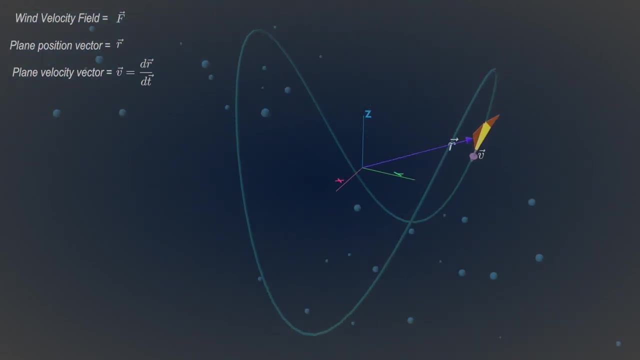 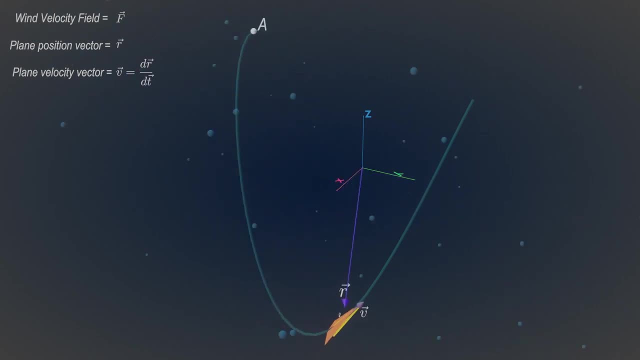 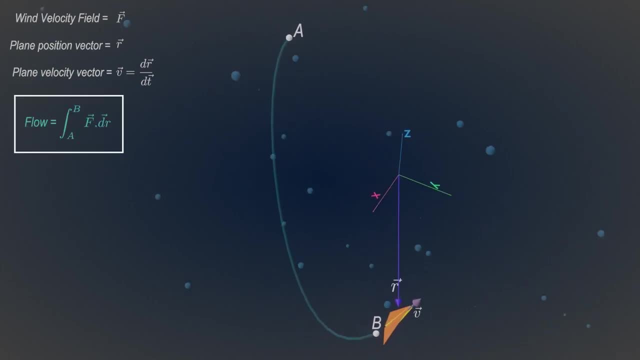 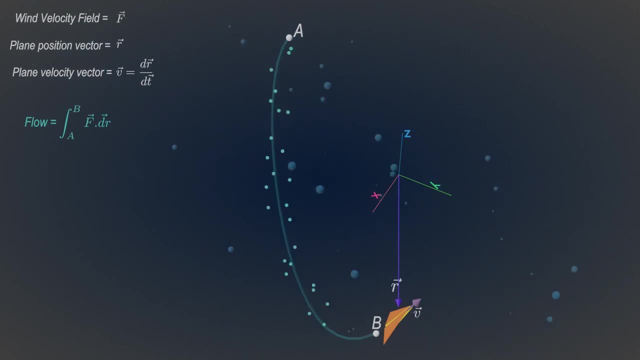 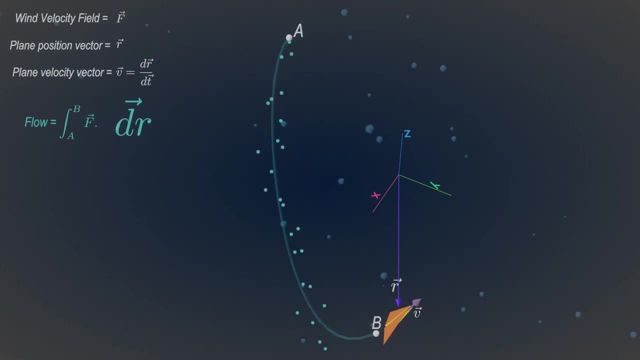 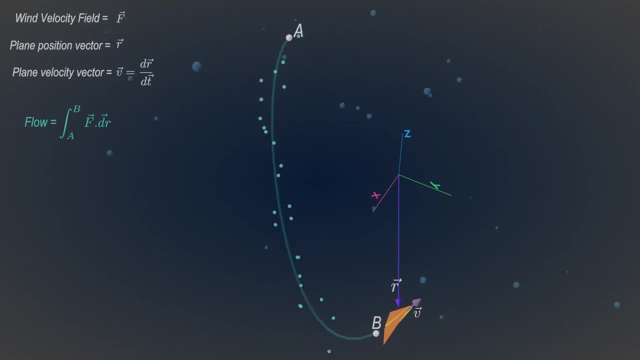 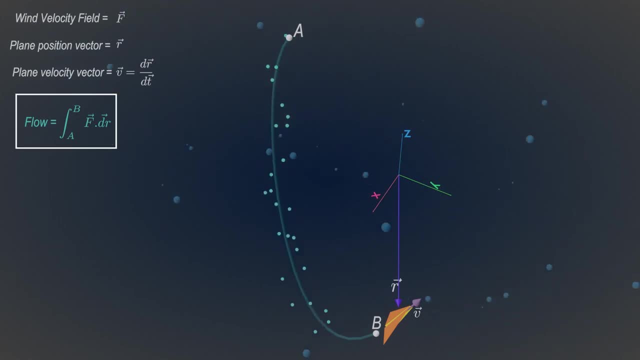 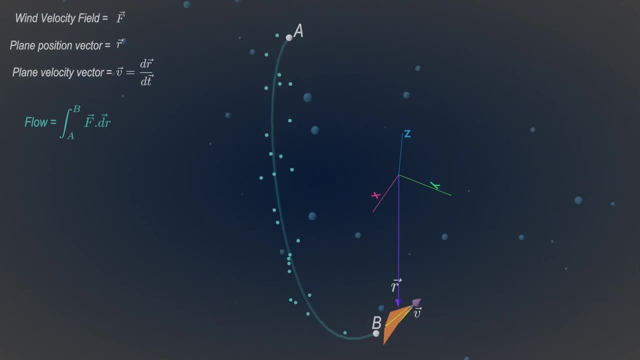 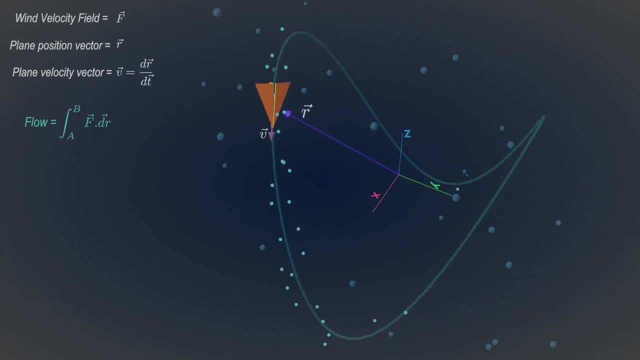 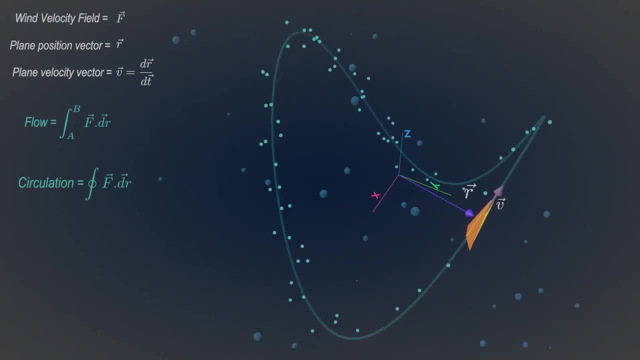 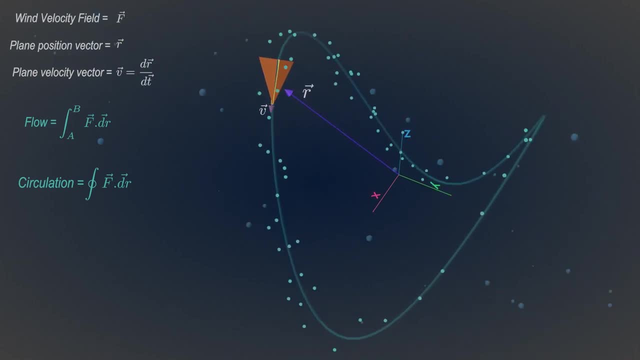 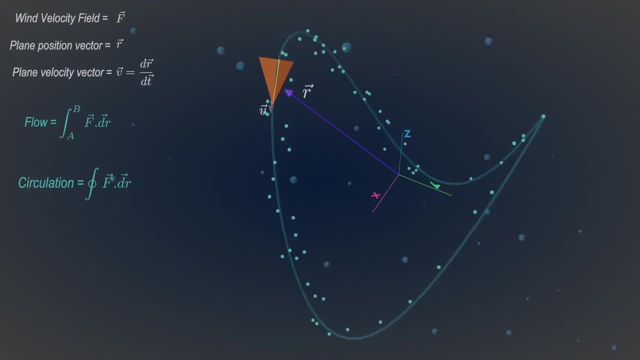 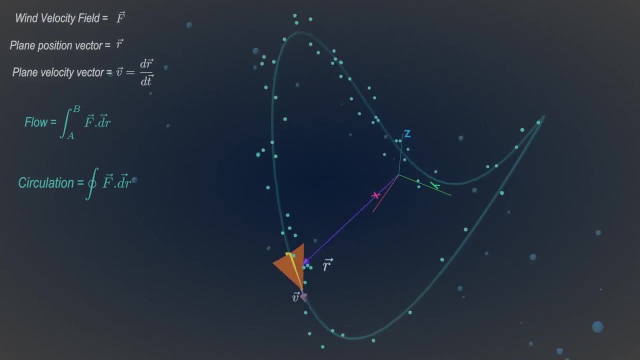 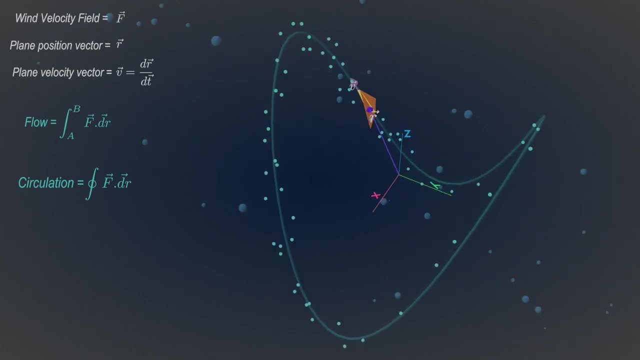 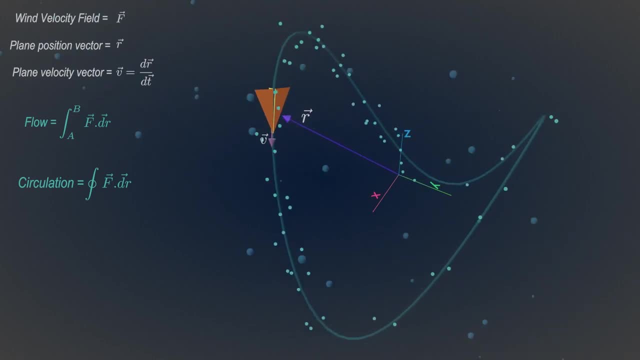 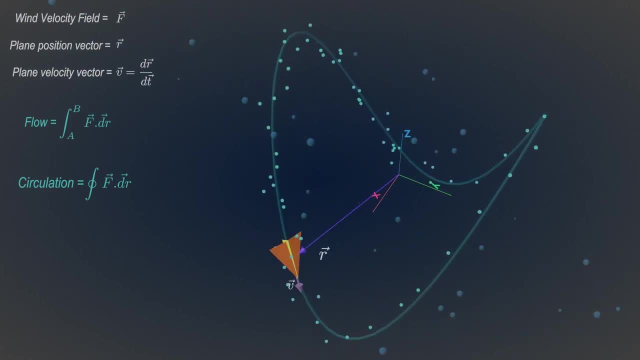 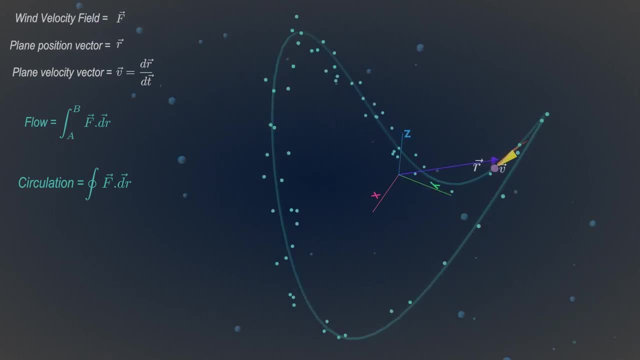 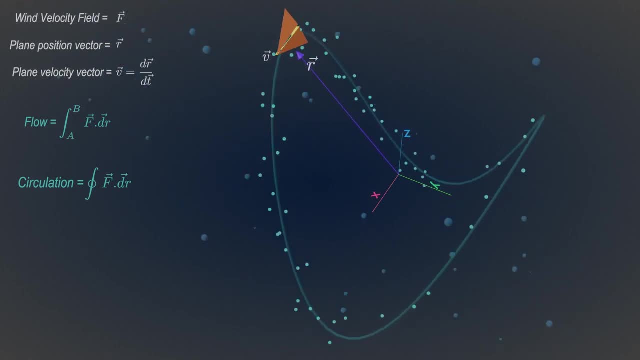 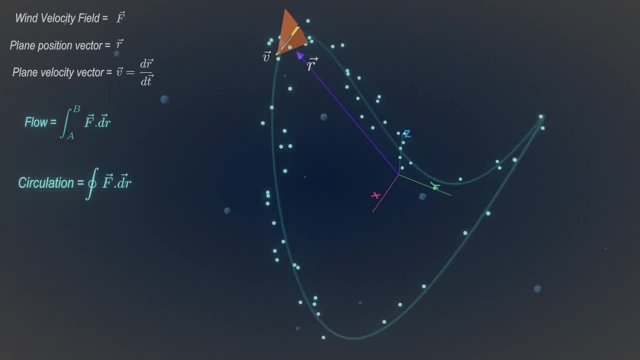 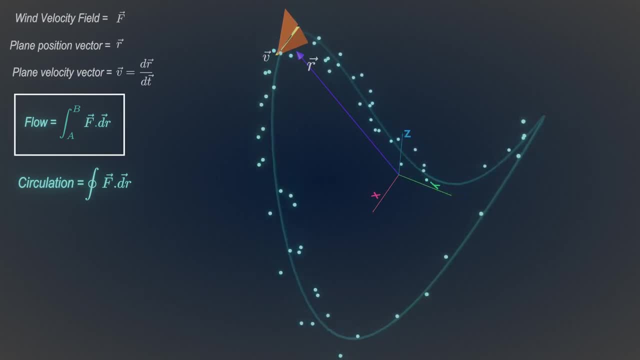 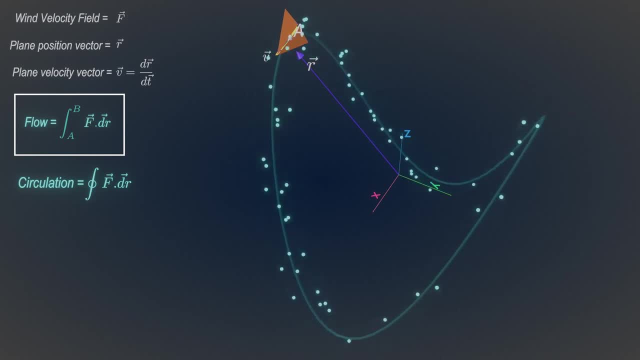 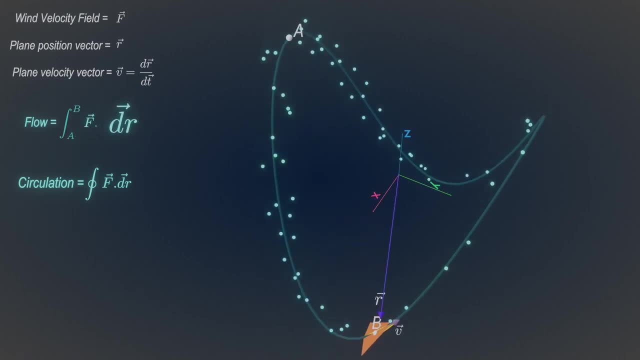 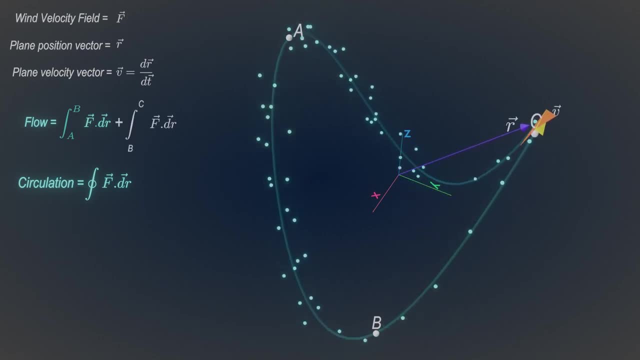 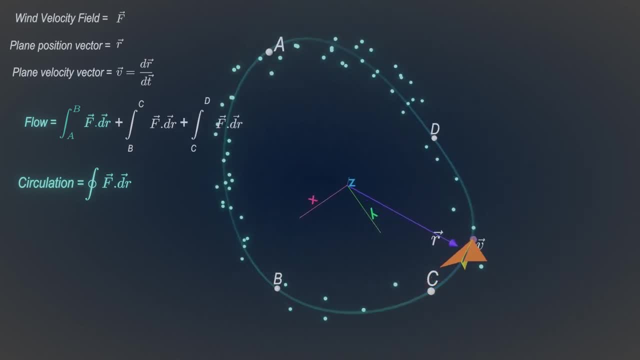 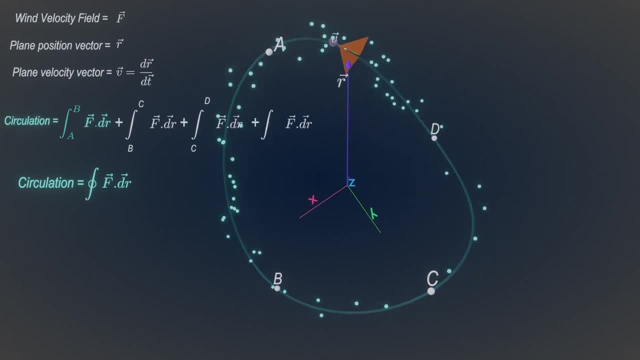 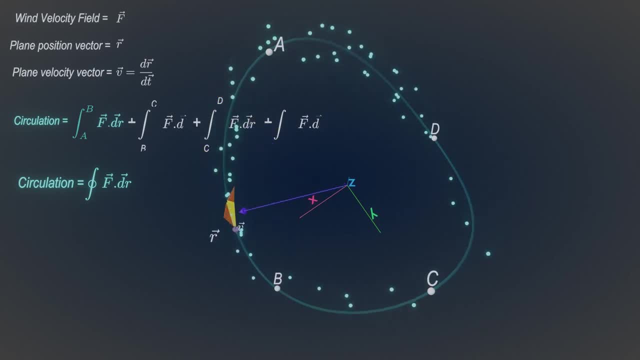 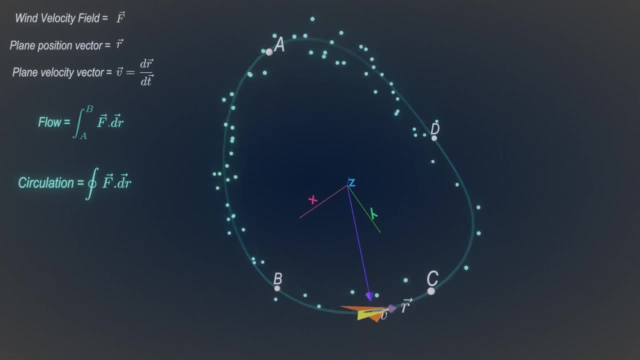 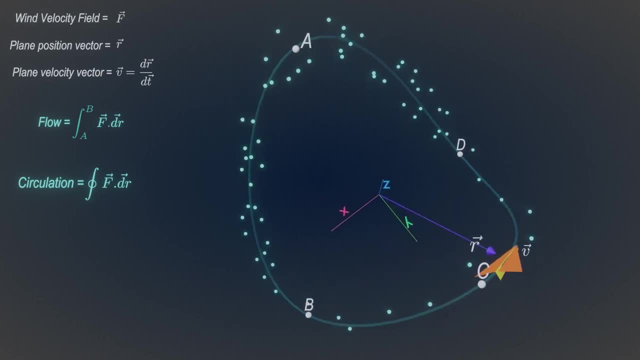 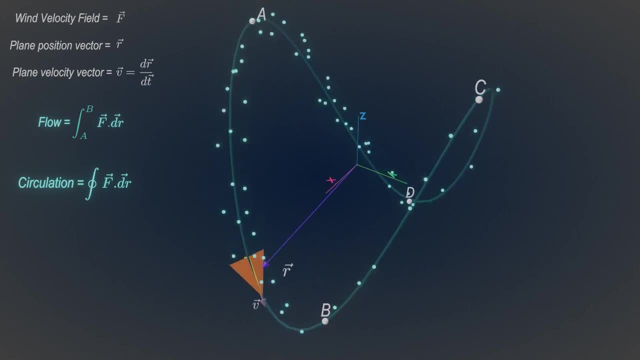 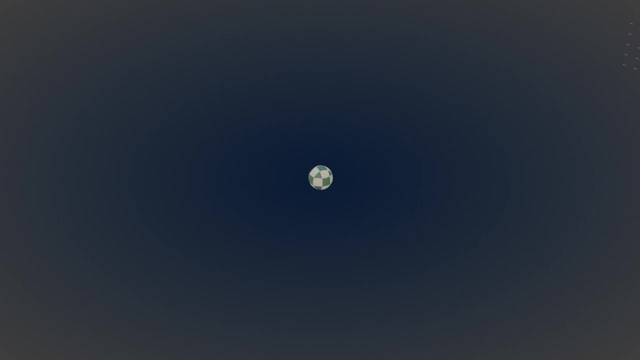 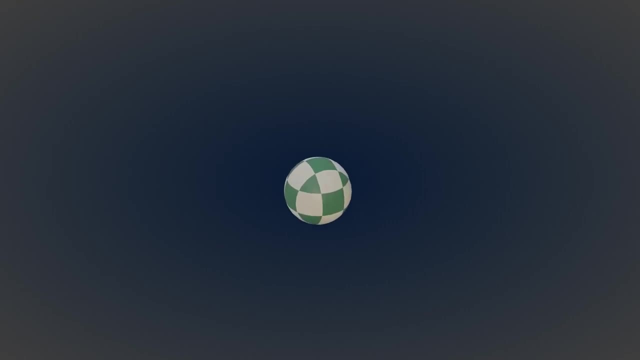 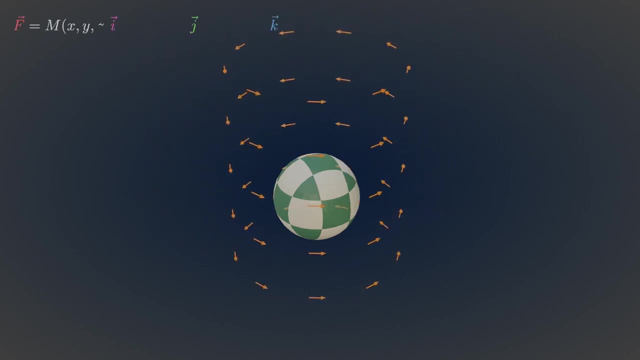 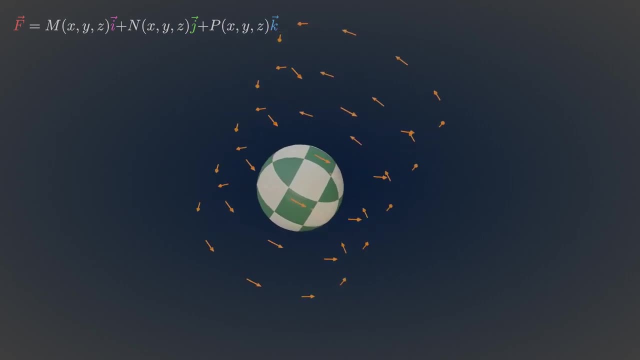 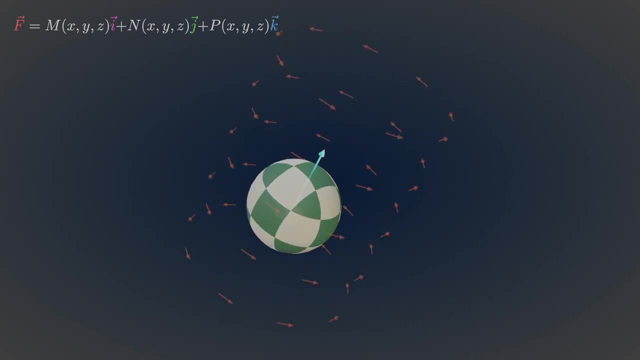 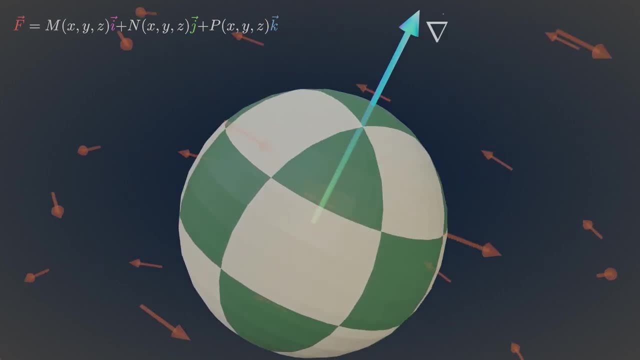 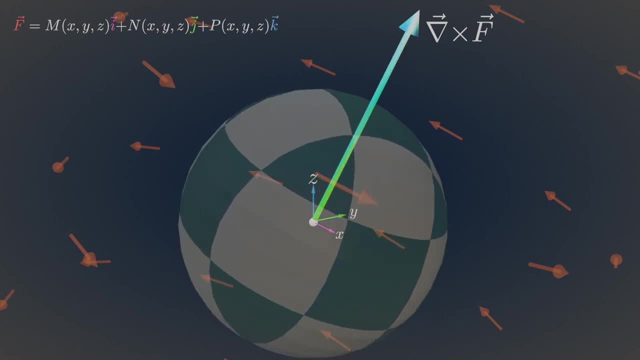 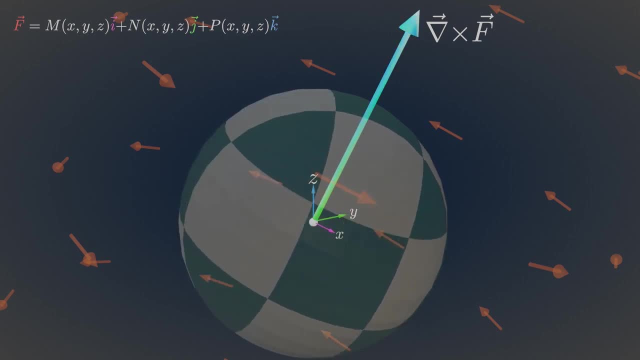 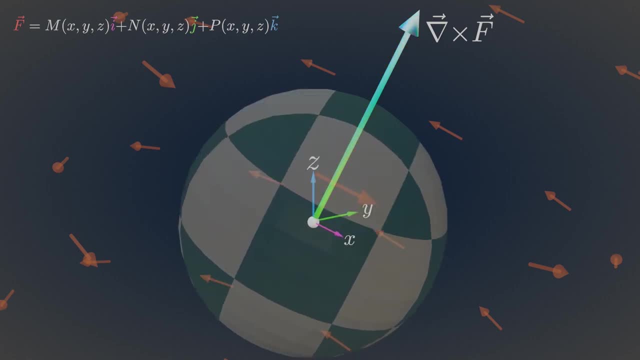 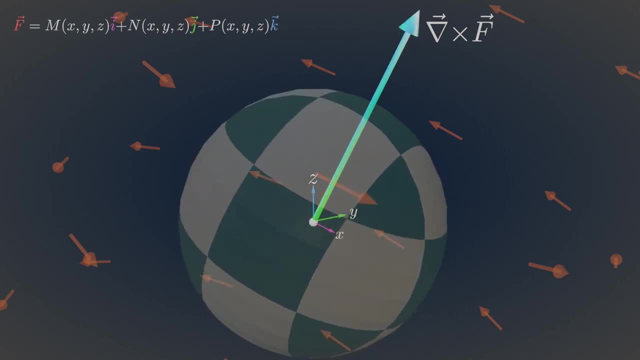 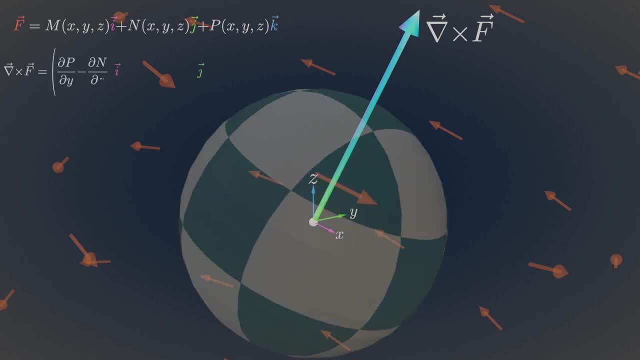 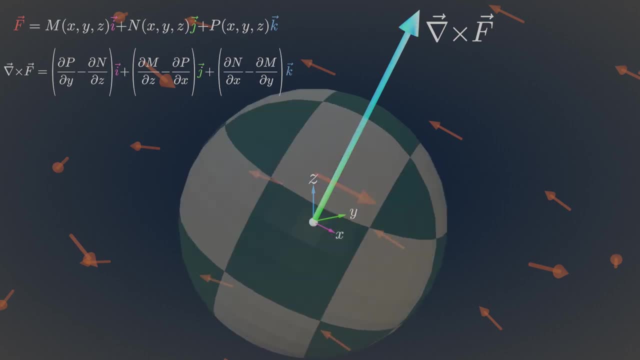 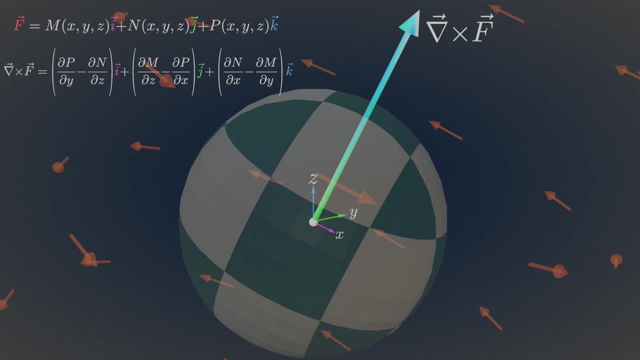 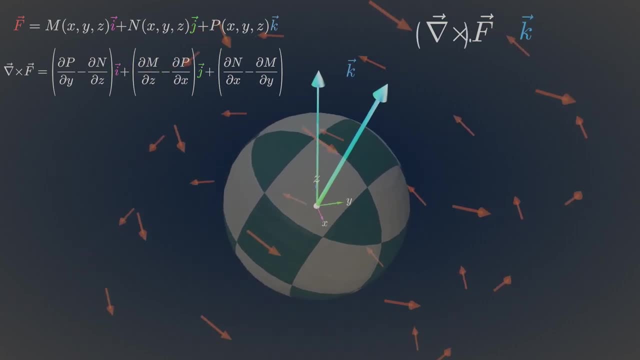 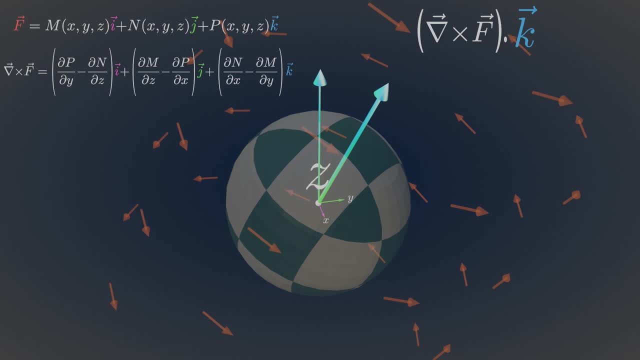 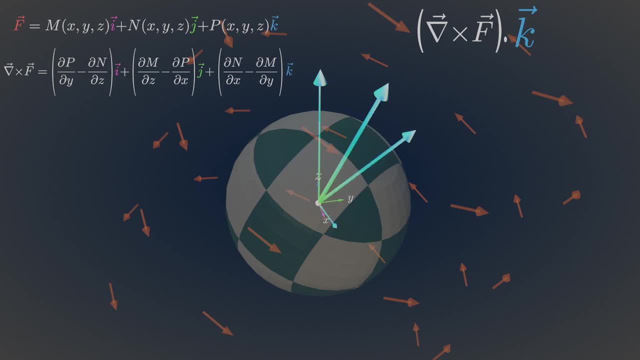 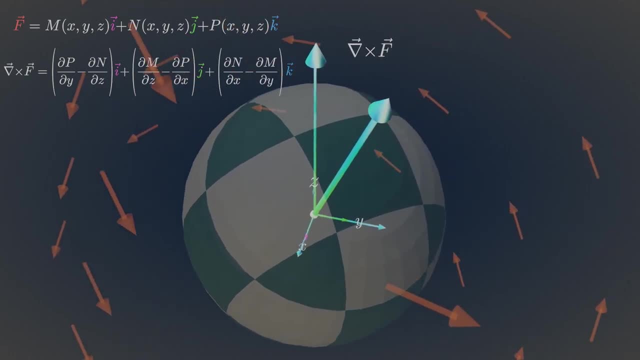 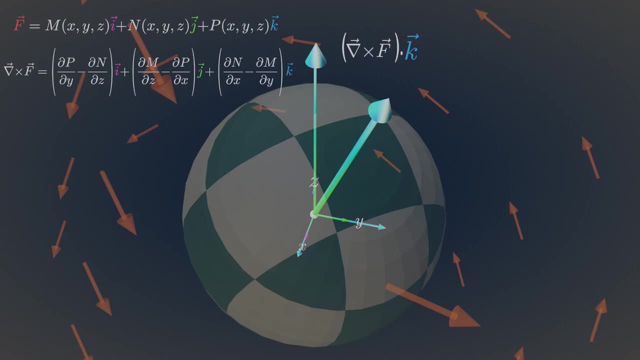 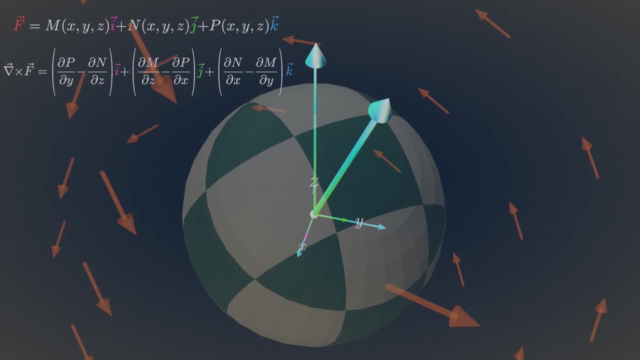 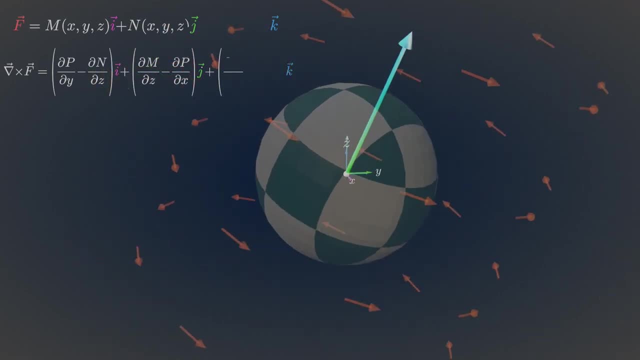 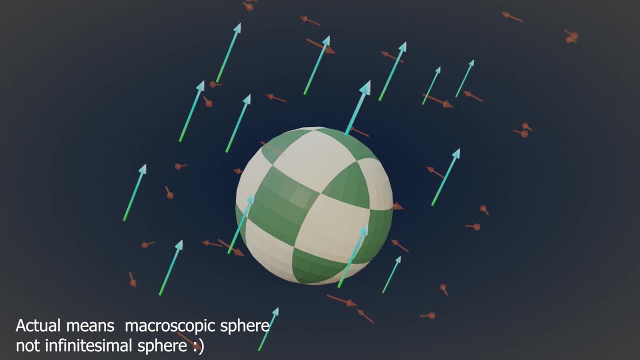 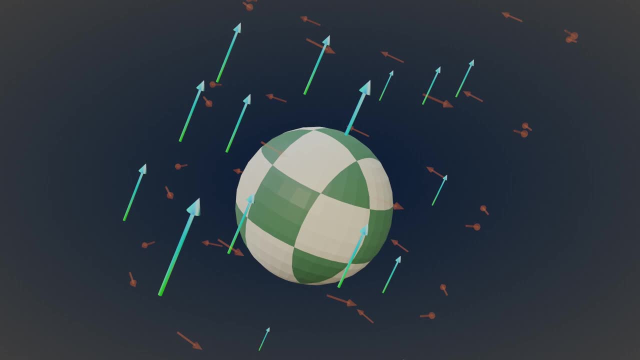 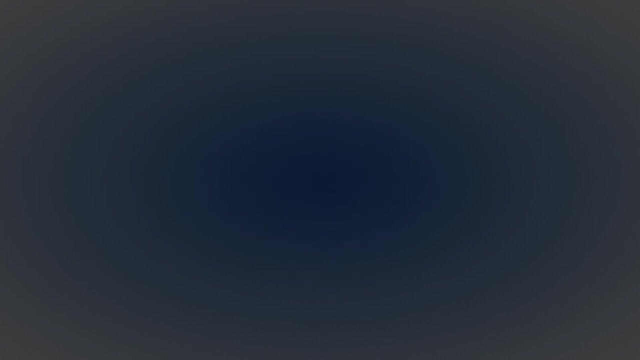 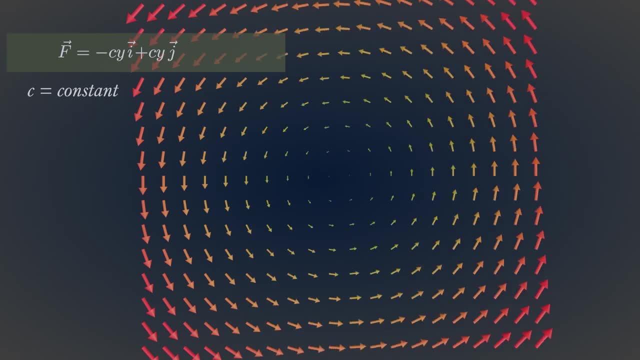 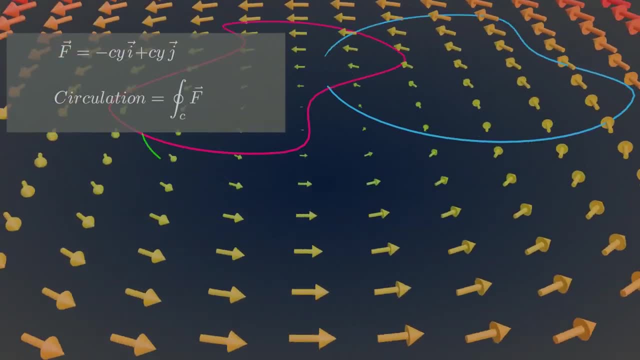 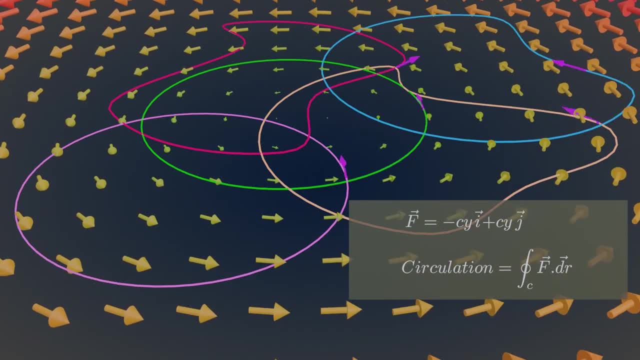 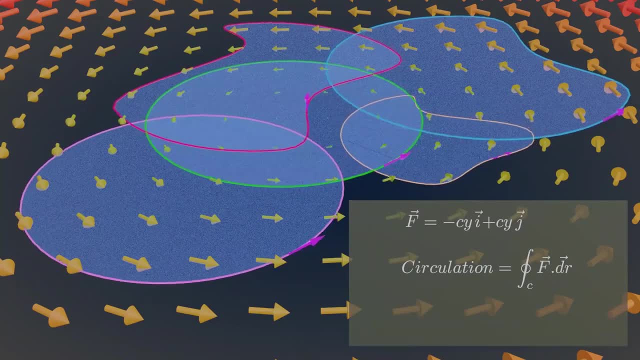 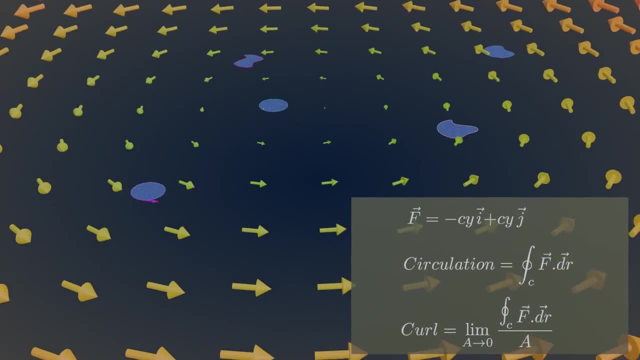 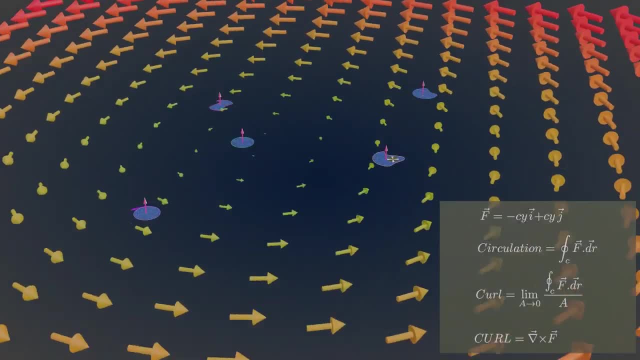 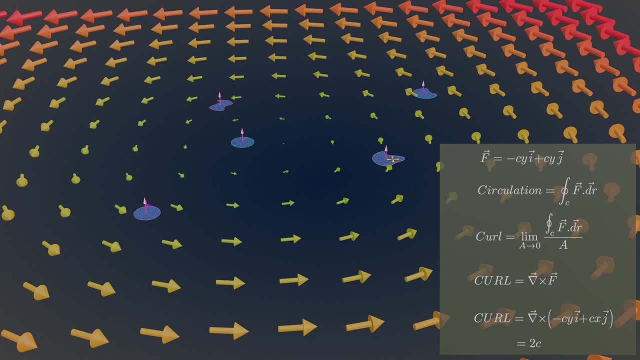 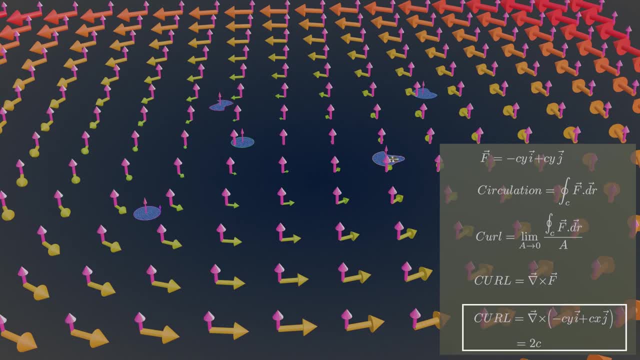 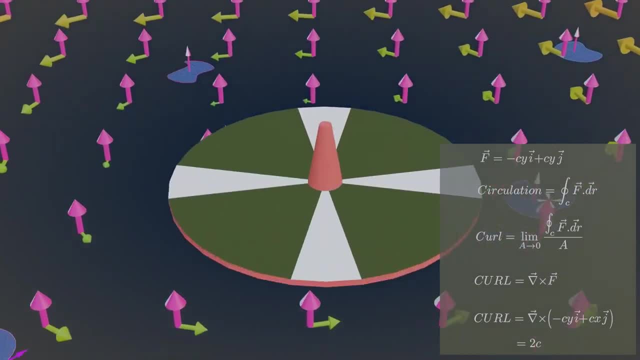 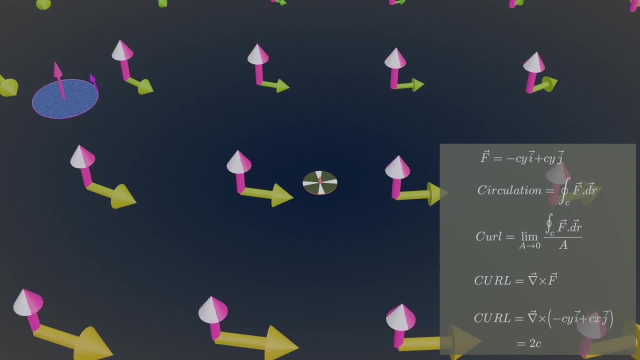 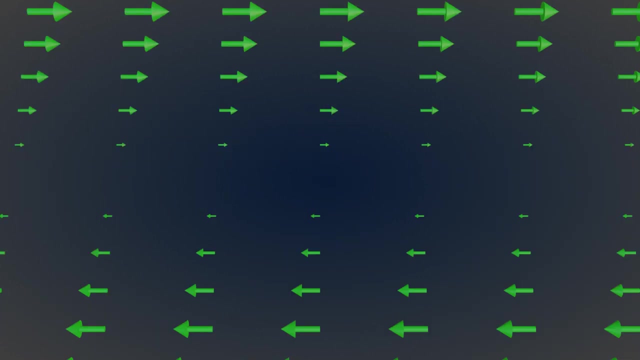 counterclockwise. If you put an infinitesimal small wheel or disc in this vector field and fix it at a point, then it will rotate due to curl. The magnitude of rotation in this case is 2.. Now consider this shear field of water. 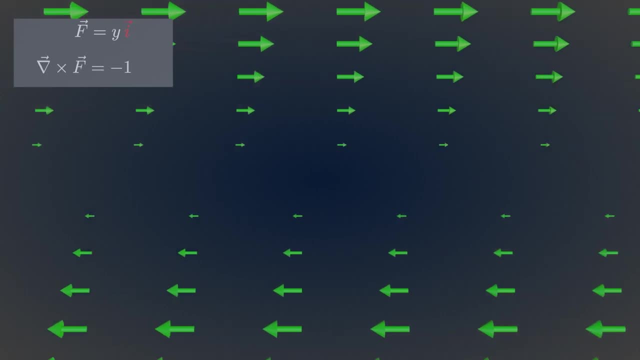 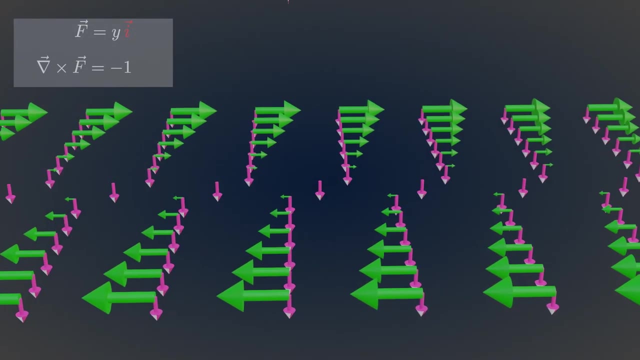 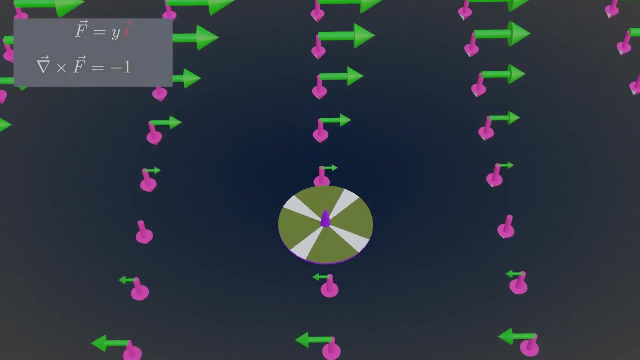 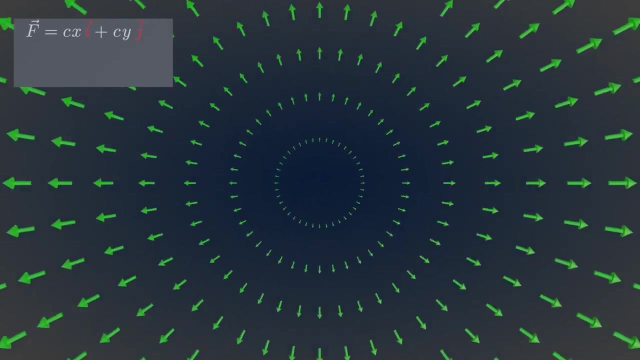 Let's calculate the curl at each point of this vector field. The curl is constant and negative here. So a wheel floating on water undergoing such a shearing flow spins clockwise. The rate of rotation is same at each point. Here is another vector field, A uniform expansion. The curl is zero here. 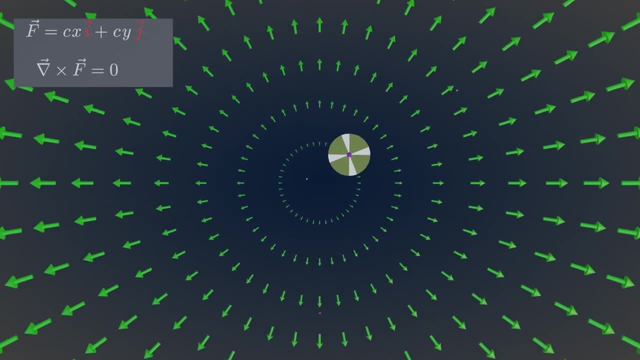 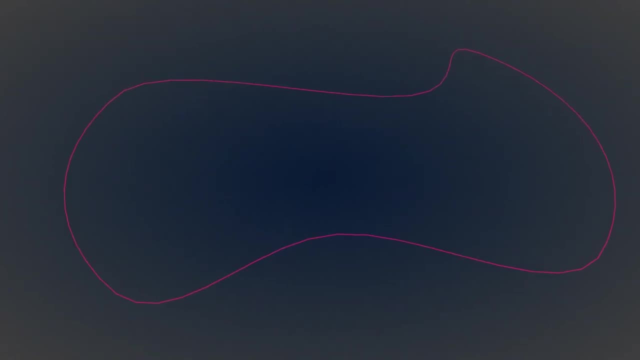 This means the gas is not circulating at very small scales. Let's calculate the curl at each point of this vector field and fix it at a point of this vector field. Okay, now we can compute circulation and curl. Now, if our line integral happens to be into: 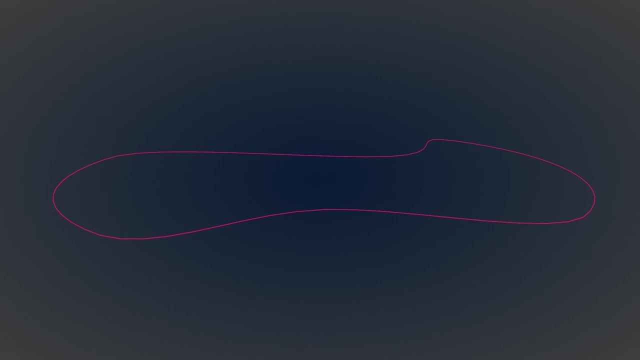 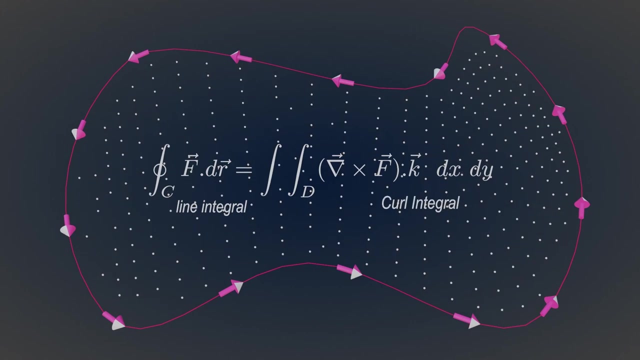 dimensions, then Green's theorem applies and we can use Green's theorem as an alternative way to calculate the line integral of this same curve. Green's theorem transforms the line integral around the closed curve into a double integral over the region inside our curve. First, think of this integral as the macroscopic circulation of the vector field around the path. 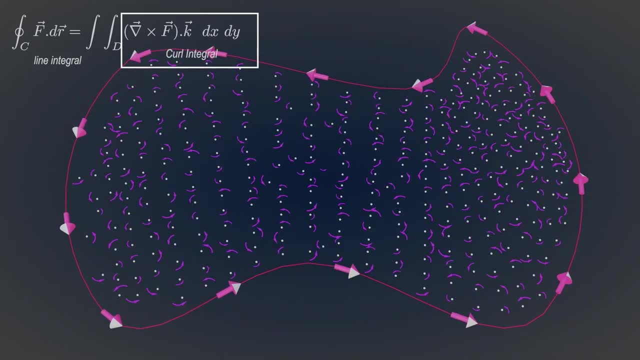 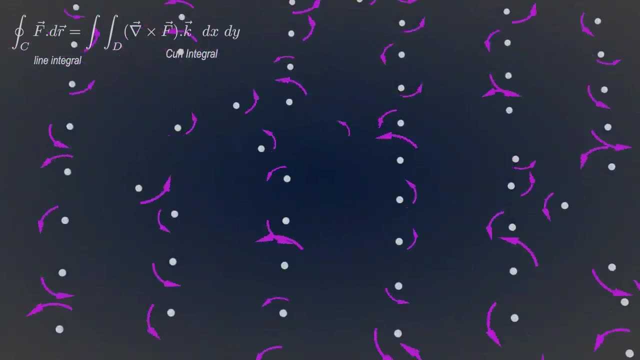 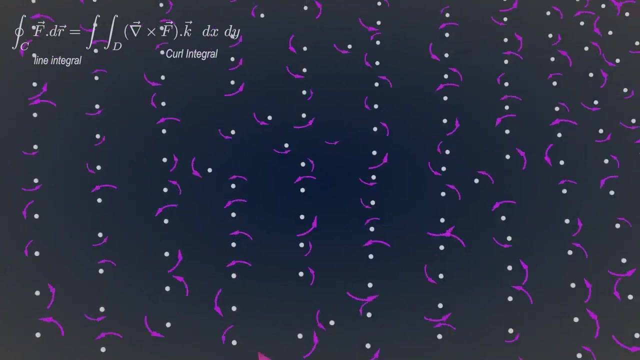 of our curve. Now imagine you came up with a microscopic version of circulation around a curve. In this case, this microscopic circulation is curl. We could picture this microscopic circulation or curl as a bunch of small, closed curves, where each curve represents the tendency for the vector field to circulate at that location. 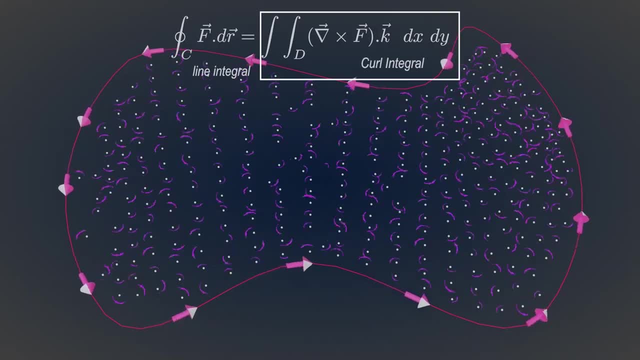 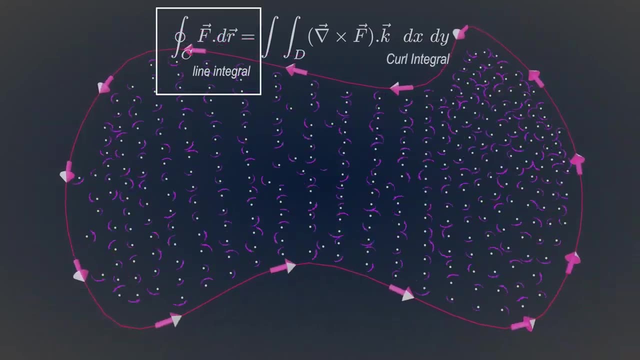 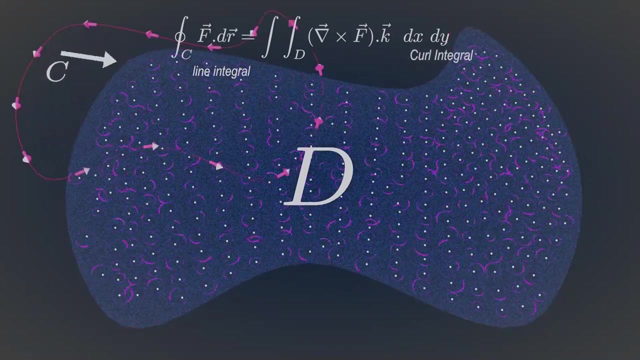 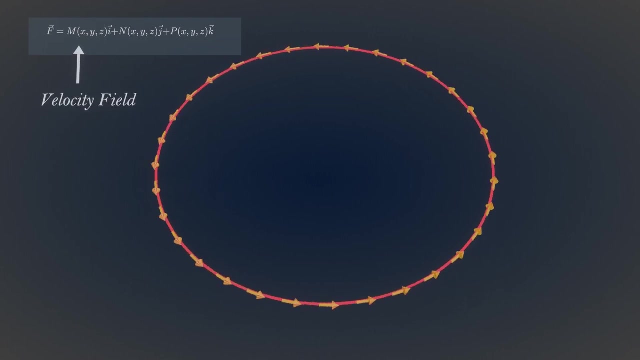 Green's theorem says that if you add up all the microscopic circulation inside our curve, then that total is exactly the same as the macroscopic circulation around the curve. Here D is the interior of the curve, C, Now in closed curve instead of tangential component. if you sum up every normal component of velocity field, 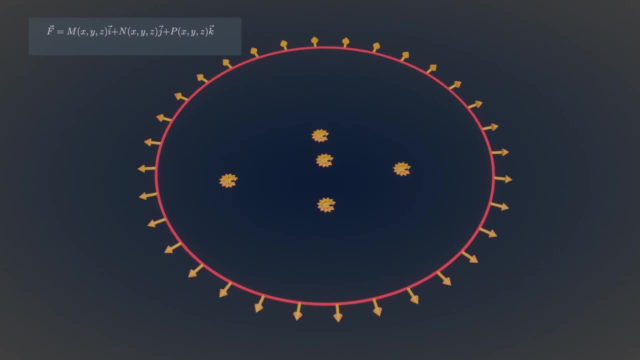 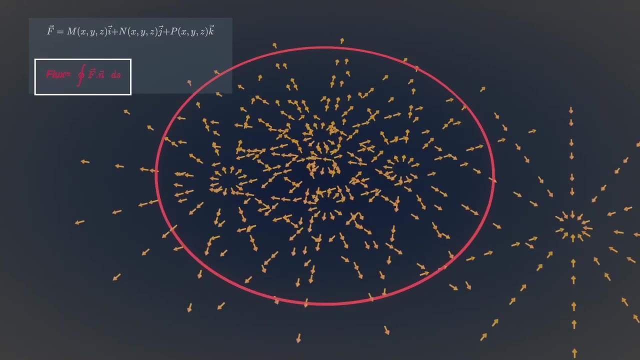 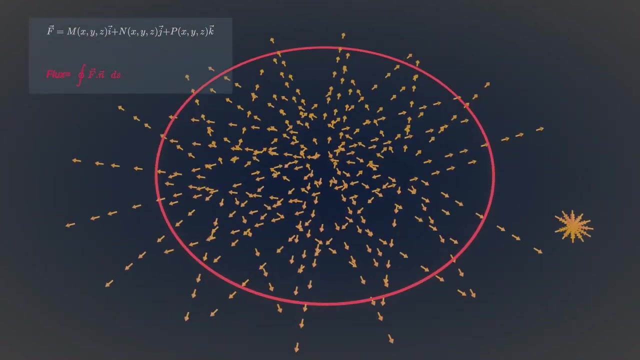 then what you get is flux. The flux calculates the rate at which a fluid is entering or leaving a region enclosed by a closed curve. By this flux formula we can get the flow across curve. Here you can see fluid particles just expands from certain point. 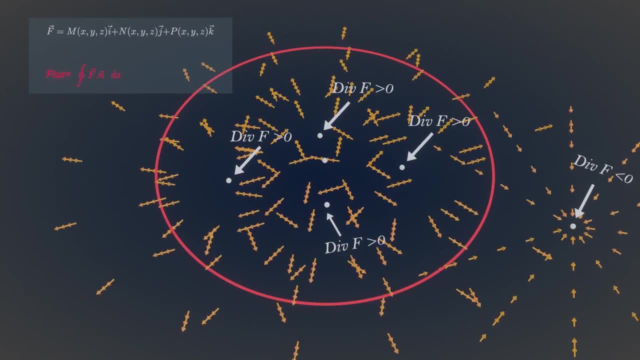 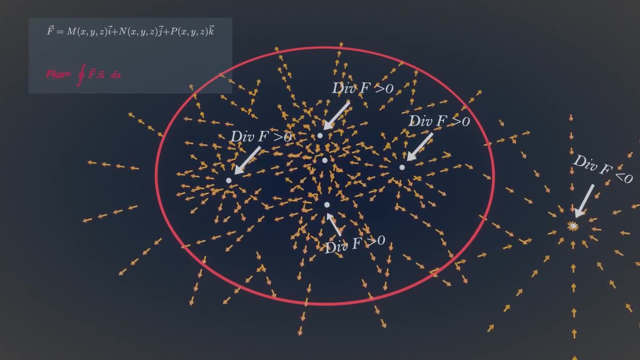 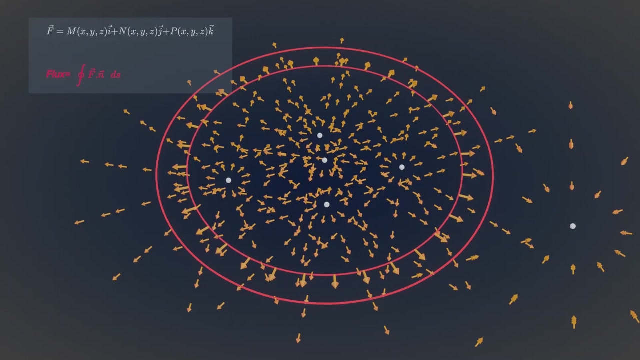 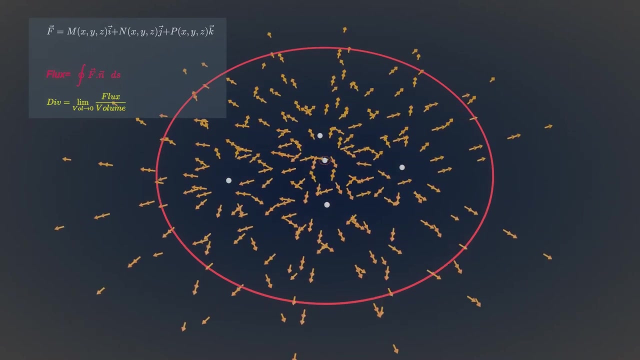 The point where fluid particles expands or compressed is the point of divergence. Divergence is microscopic, while flux is macroscopic. Divergence is occurred when flux is shrunk to zero or shrunk to a point. It can be also called as flux density. You can get divergence of any vector field. 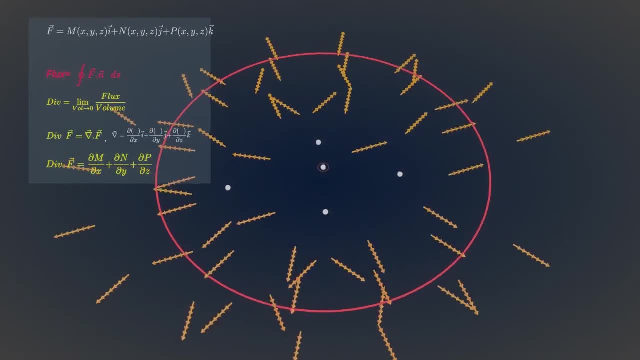 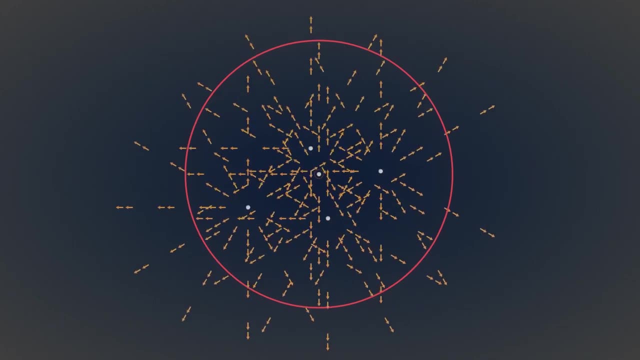 by using this formula. I hope you notice the difference between divergence and flux, density, Divergence and flux. they are closely related. So divergence occurs on point, whereas flux occurs across the curve. In Green's theorem there is a relation between divergence and flux. 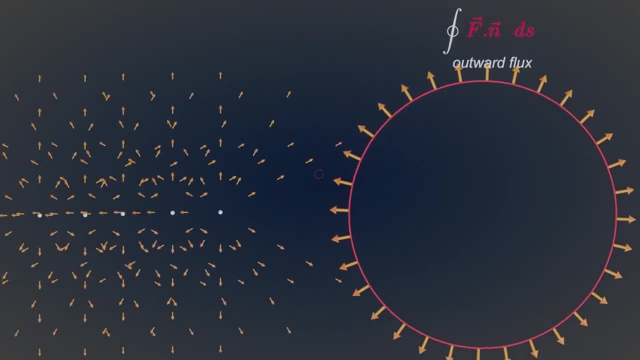 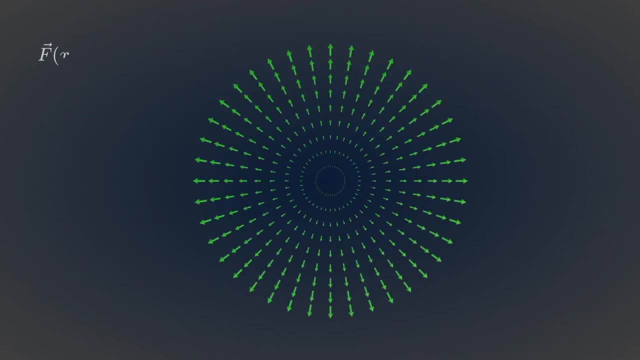 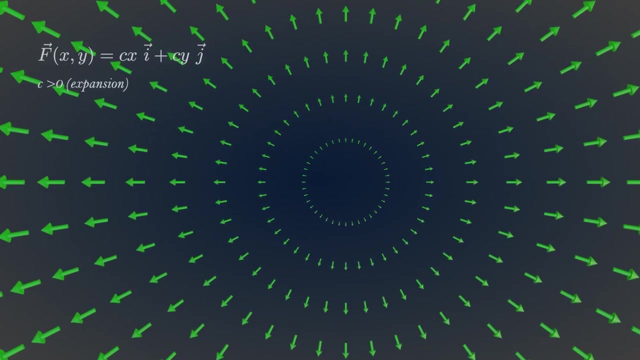 You can calculate total flux across a curve by summing up every divergence enclosed by that curve. Consider again This uniform expansion of velocity field of a gas or liquid. Now consider a point in this velocity field. If you measure divergence at this point, it would be positive. 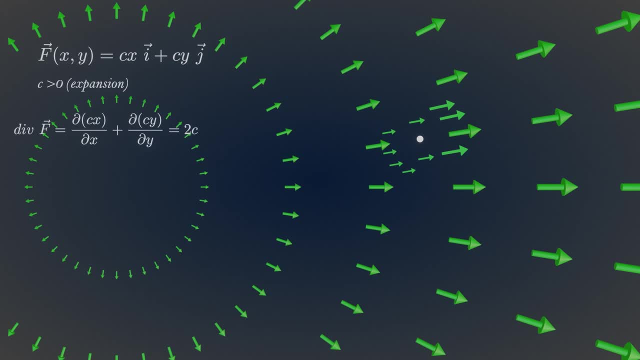 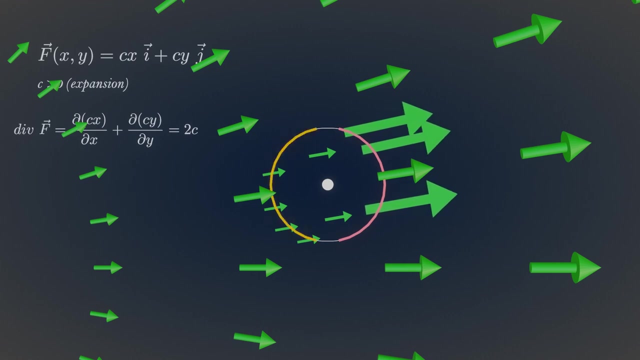 Let us draw more velocity field near its location. Okay, let's close this point by a circle. Now look at this vector diagram. the flow out of the circle is more than flow. Since flow out is more than flow in, the flux would be positive. 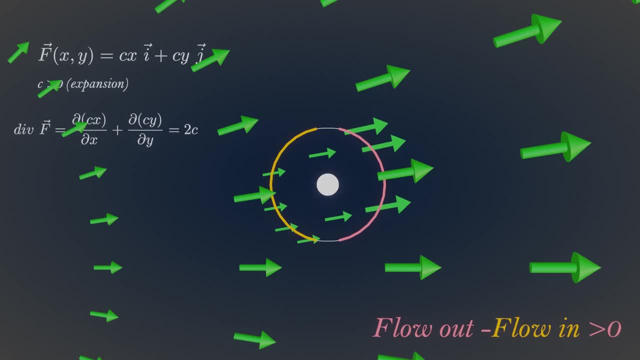 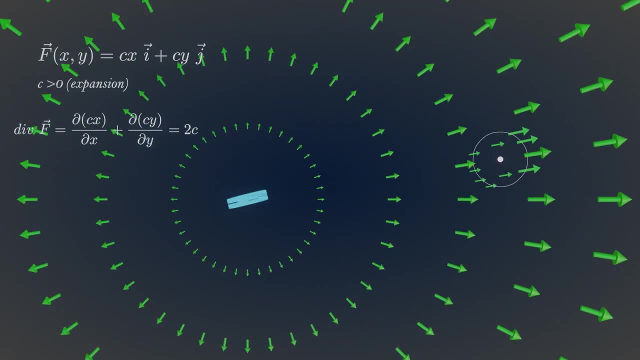 So in this case, both divergence at this point and flux out of this circle is positive. Now consider an infinite small fluid material In this velocity field. this fluid material will expand as it moves through this velocity field, so its volume increases. 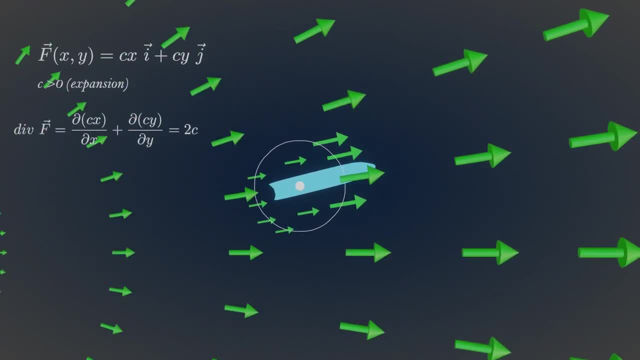 Do you know why it expands? Here the velocity out is greater, so this side of fluid element stretch more, But the flow in is smaller, so it would compress less. Overall the volume of this fluid element increases. But if this is an uniform compression velocity field, 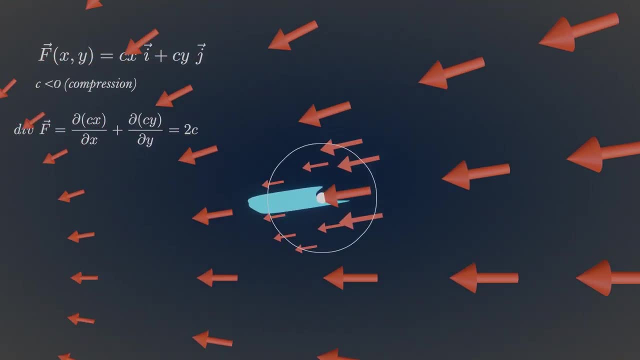 Then the fluid particle will be compressed and the volume decreases. This is because the volume of this fluid element is greater than the volume of this fluid element. So the volume of this fluid element is greater than the volume of this fluid element. 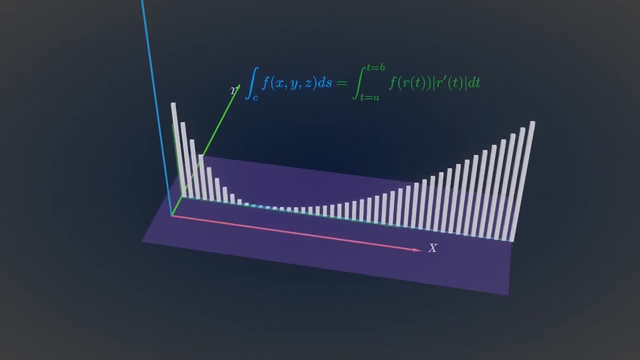 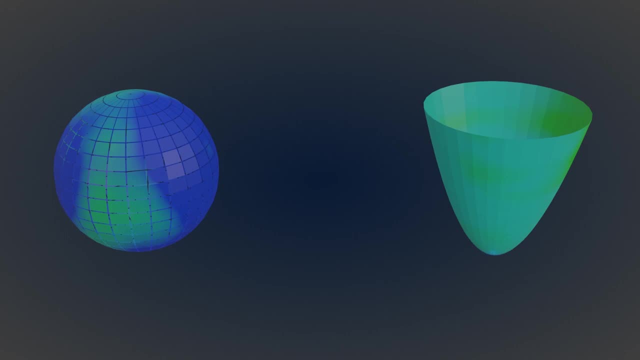 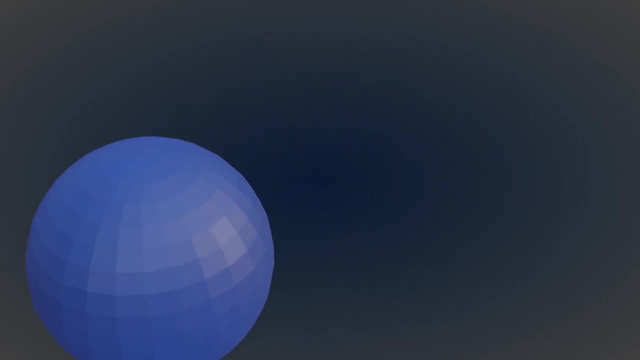 You have seen in line integral how a curve in space is parametrized to a single t-axis. Just like that, we will learn how to parametrize a 3D surface into a plane. Okay, our goal right now is to find a double integral formula for calculating the area of. 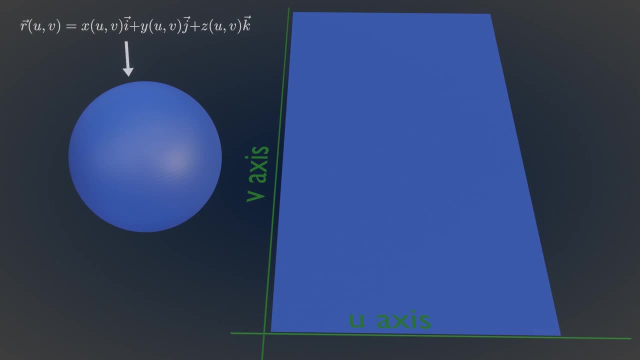 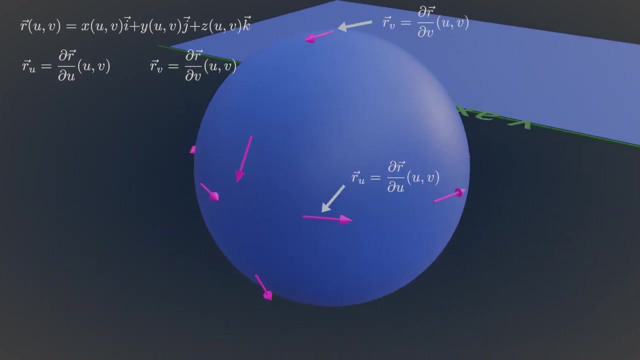 this sphere based on the parametrization. Okay, if you partially differentiate this parametrization with respect to U and V axes, Then geometrically it can be represented in terms of tangent vectors. For instance, if V is held constant, then this parametrization is a vector-valued function. 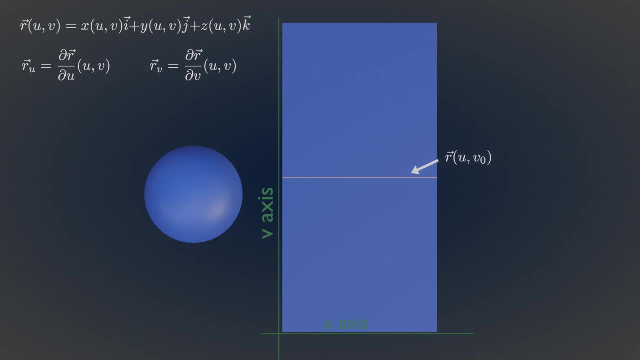 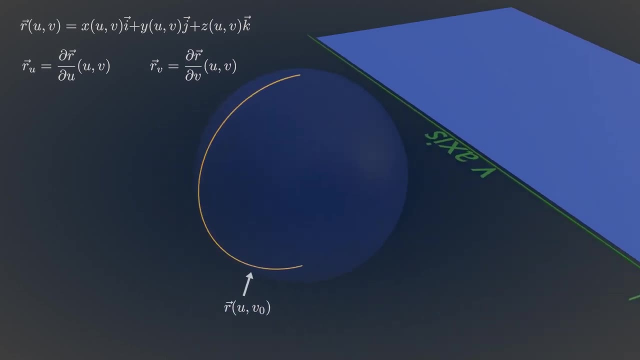 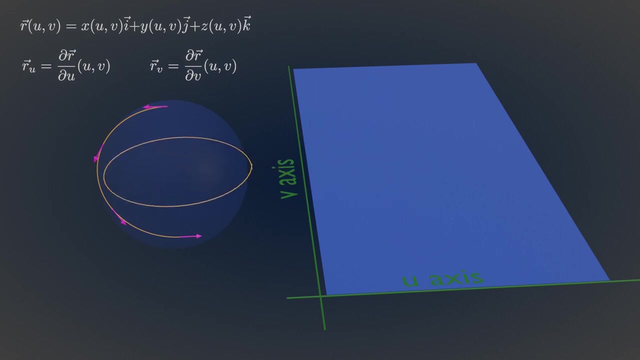 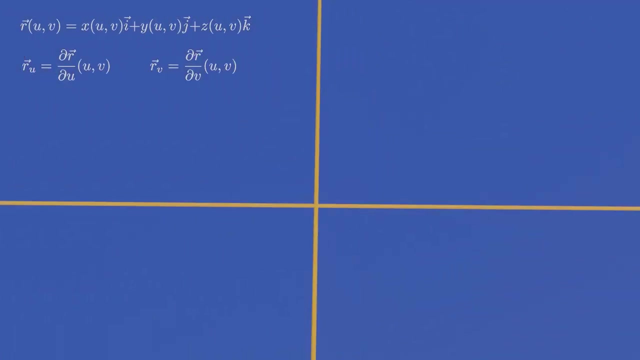 of a single parameter and defines a curve that lies on the surface of our sphere. Its partial direction is the same as the vector's direction. Its partial derivative is tangent to our surfaces. The same goes if U is held constant. Now take any point in the UV plane. 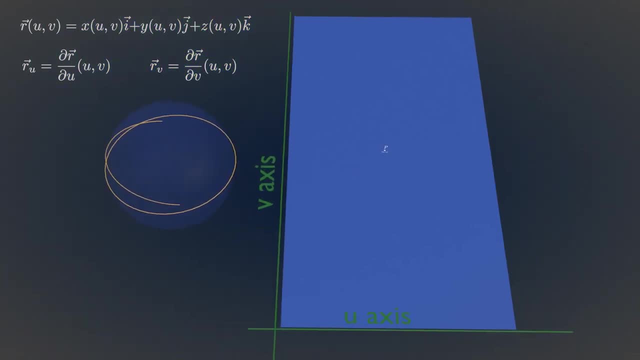 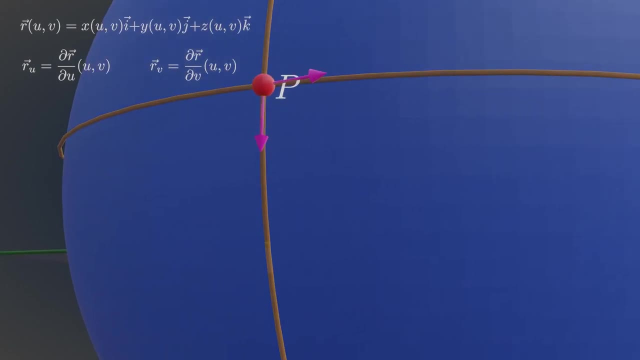 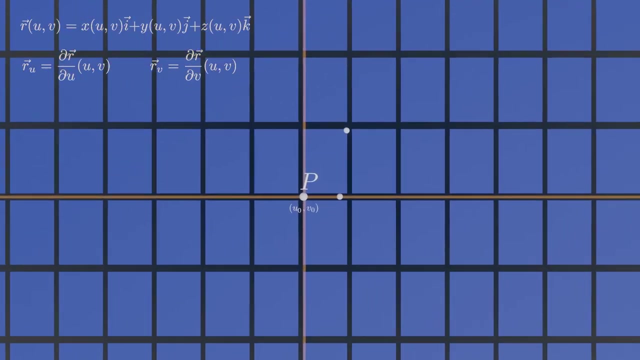 This point can be mapped to a point in surface in 3D space, The partial derivative at that point can be found, which is a vector. Notice, these two unit tangent vectors creates a plane which is tangent to our surface Now in UV plane. at that point, take a tiny, infinitesimal piece of rectangle. 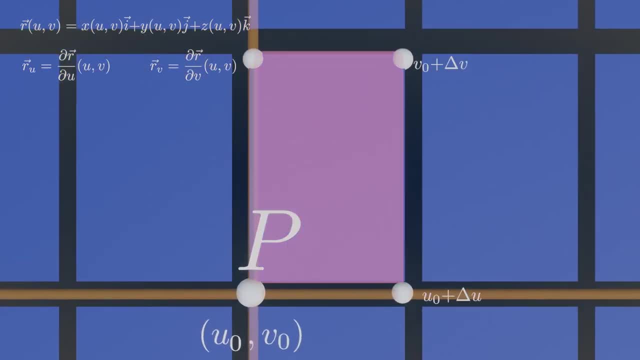 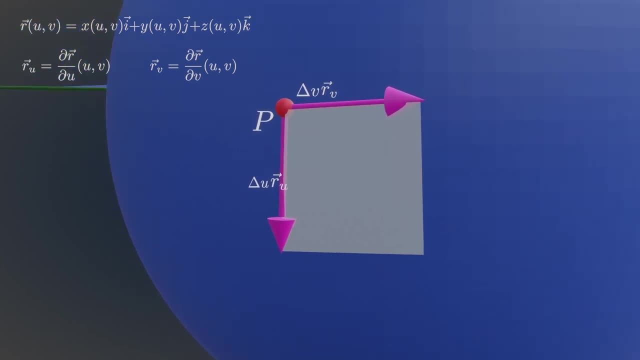 The length and width of this rectangle can be mapped to our unit tangent vector. Now take the cross product of these two vectors. What will you get? The cross product of these two vectors is another vector perpendicular to this plane. So this new vector is perpendicular to our surfaces. 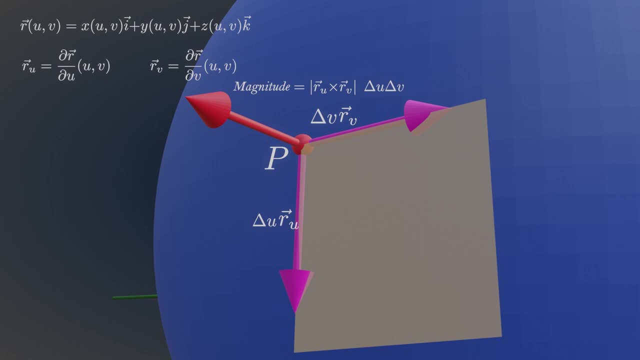 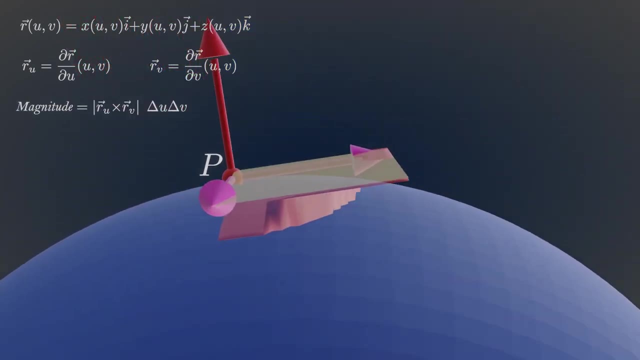 The magnitude of this new vector is area of this parallelogram And the area of this parallelogram can be nearly equal to the area of this plane And the area of this parallelogram can be nearly approximated with the area of this infinitesimal small surface. 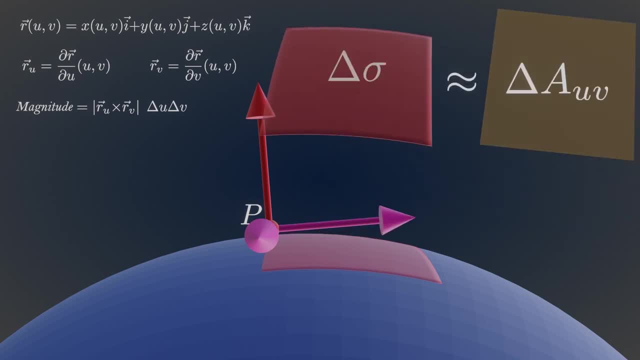 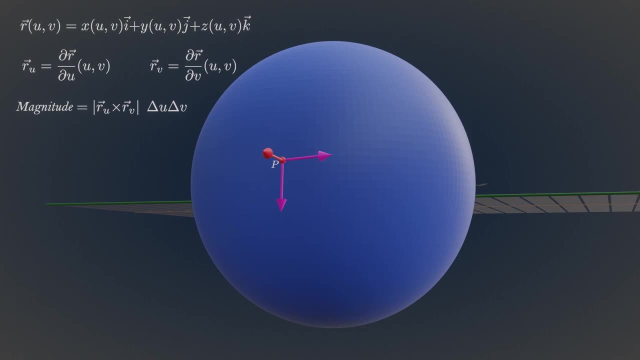 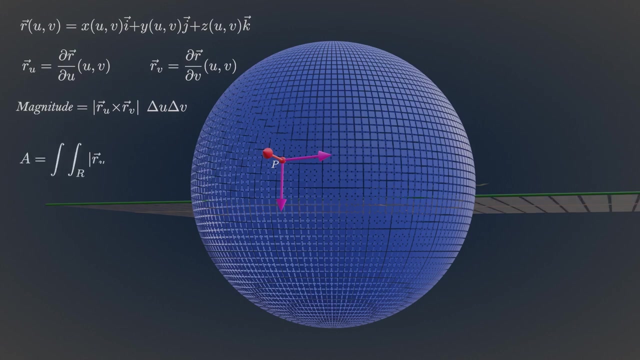 Or the area of this curved patch element. That's the area for one patch element. Now, in order to calculate the total area of this whole patch of sphere, we need to sum up every rectangle of this UV plane. This summation is done by double integral. 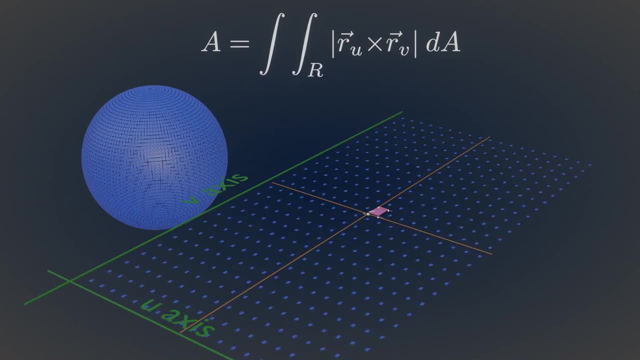 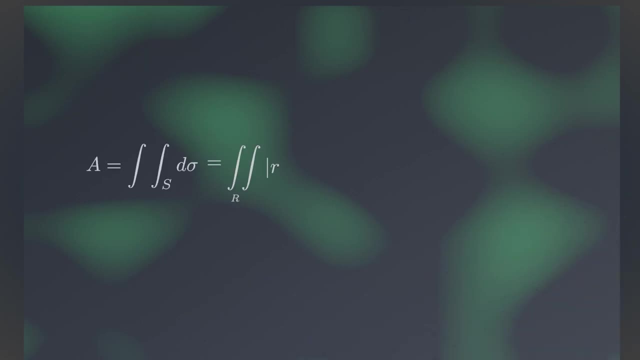 So if you integrate this integral, you will get this. So if you integrate the area of this rectangle, you get the area of this sphere. You can use this formula to calculate surface area of an parametrized 3D surface. 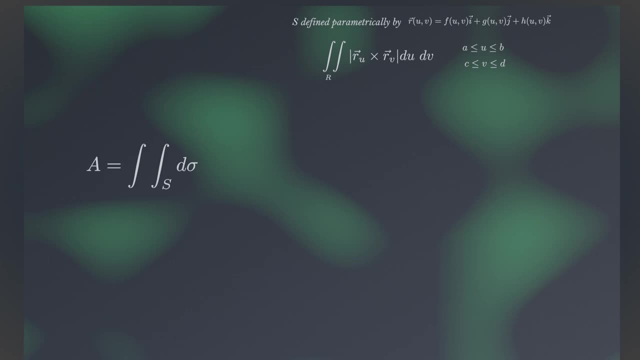 But many times you would encounter a surface which are not parametrized. The other surface you will encounter will either be an explicit or an implicit function. If a surface is an implicit form, you can use this formula. If a surface is an explicit form, then you can use this formula to calculate surface area. 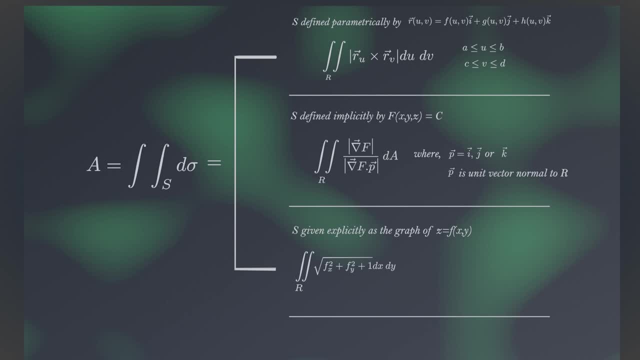 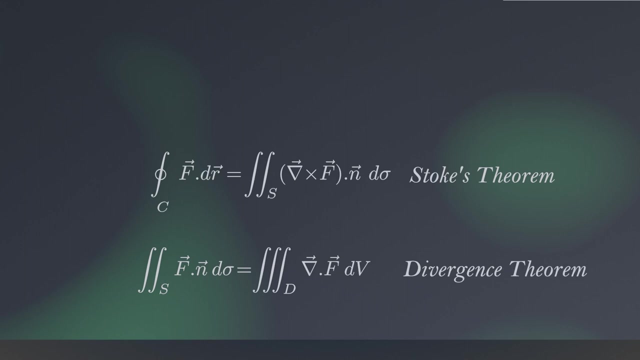 If you understand, really understand, how to use these three formulas, then one thing is for sure: You can easily master the vector calculus course In Stokes' theorem, divergence theorem and computing surface integrals. computing these differential patch element is very important. 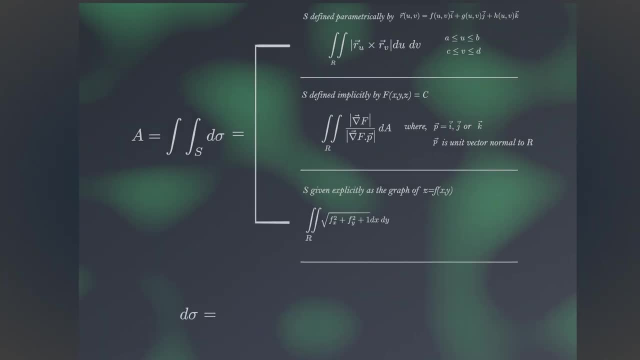 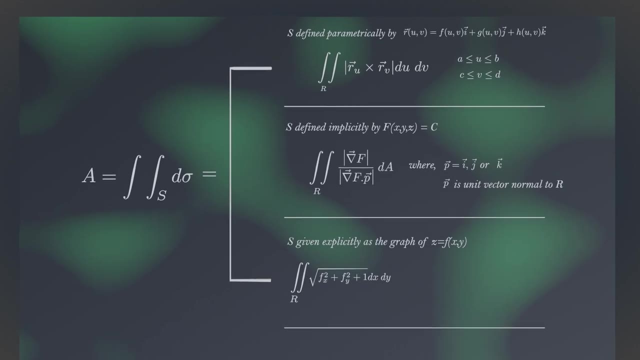 computing these differential patch element is very important. once you understand how it is obtained, calculation would be very easy. i have showed how this parameterized formula has arrived. now it's your homework to understand the derivation of these two formulas. if you understand the derivation of this parameterized surface area, then understanding. 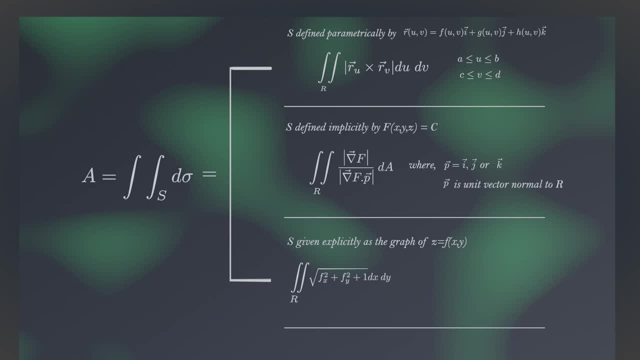 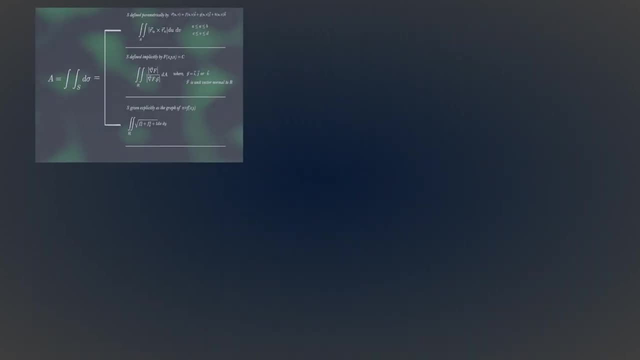 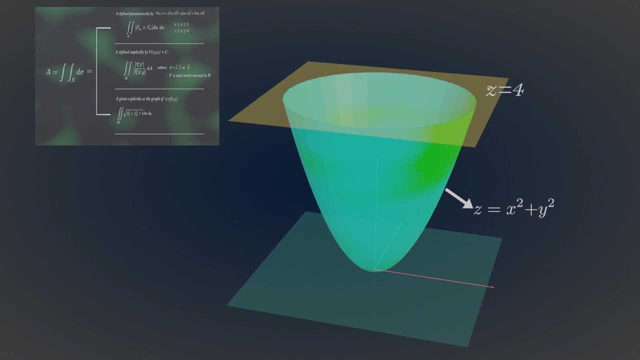 these two is quite easy. now let's understand how to use these three formulas. let's use these tools on finding the surface area of this paraboloid, which is cut by a plane. z is equal to 4 in space. first sketch the surface. this is an explicit function. looking at our formula sheet, we can: 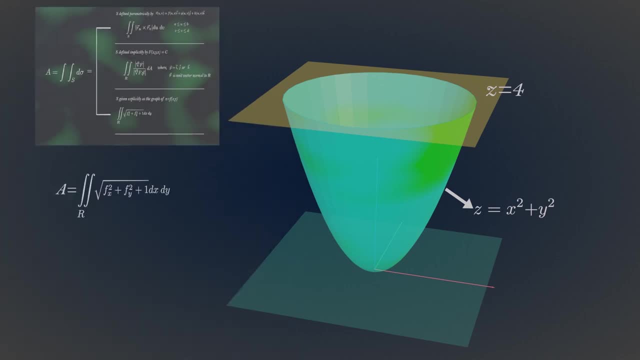 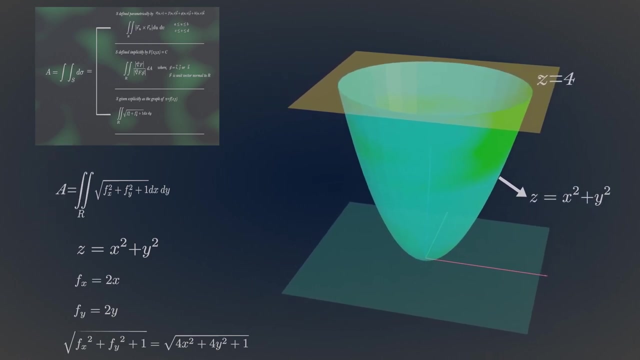 use this formula for calculating surface area. now partial differentiate this explicit function with respect to x and then with respect to y. then the surface area is given by this double integration. now, in order to find the region r project, this paraboloid in the x, y plane. 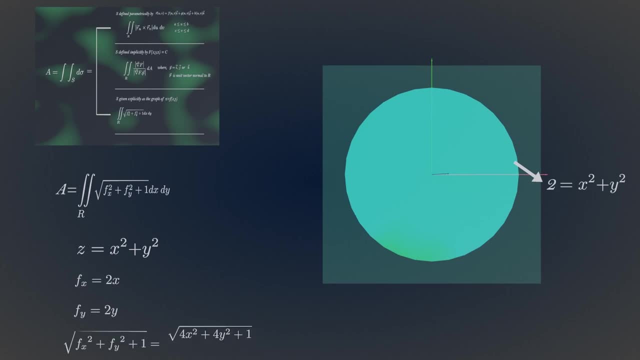 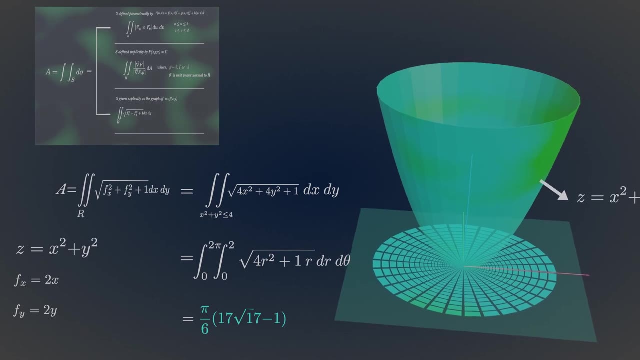 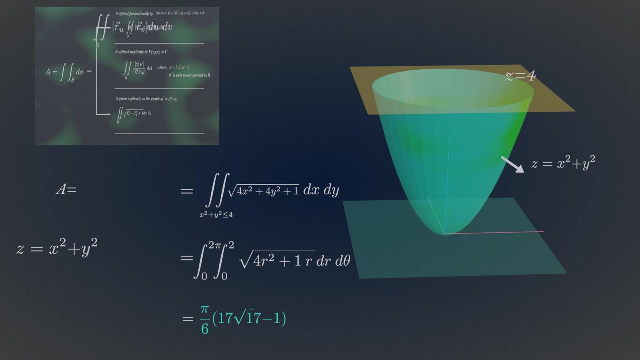 which is circle of radius 2. now just double integrate over the region of this circle, you will get the area of this paraboloid. now let's solve this same problem using parameterization method. you will soon see that the area would be same. first parameterize the parabola, now partial differentiate it, now calculate the cross product. 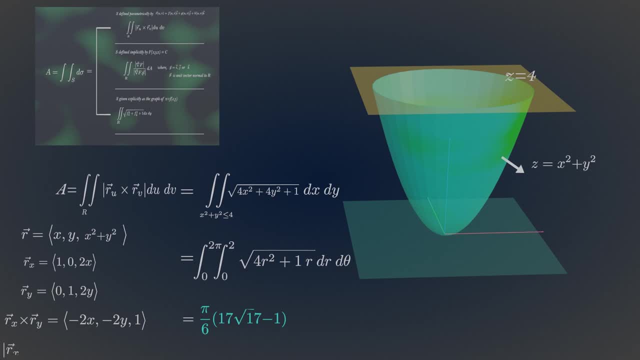 of these two vectors. now we require the magnitude of their cross product. finally, integrate this magnitude over the circle. the answer would be same. now let's solve this same problem using the implicit method. first, convert this explicit function to implicit function. now compute its gradient. therefore, we will be able to calculate the gradient of this function by using the implicit method. 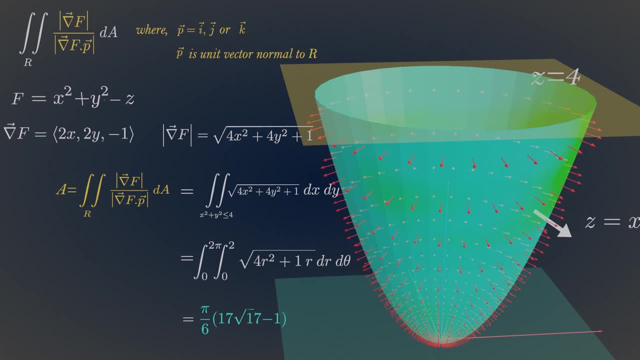 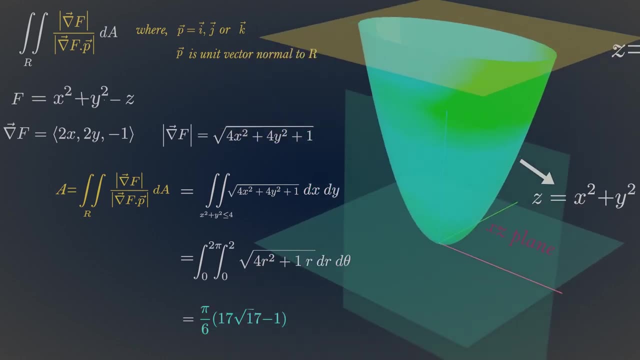 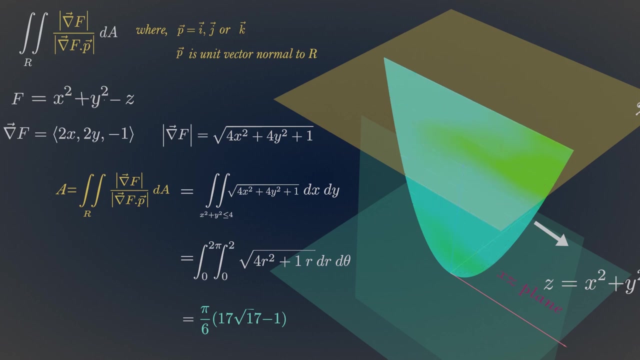 therefore the magnitude of gradient is. now you need to find the unit p vector. if you project this paraboloid into x- z plane, then unit p vector is equal to unit j vector, but the projection is not one to one and you can't double integrate over this region. there is another way: you can project it: on x- y plane. 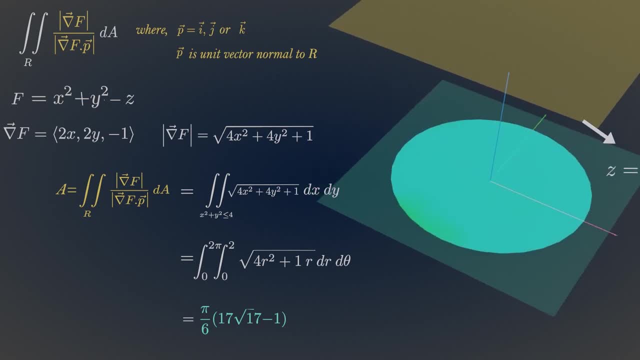 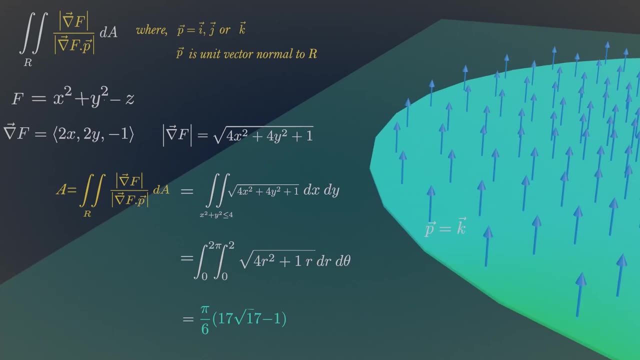 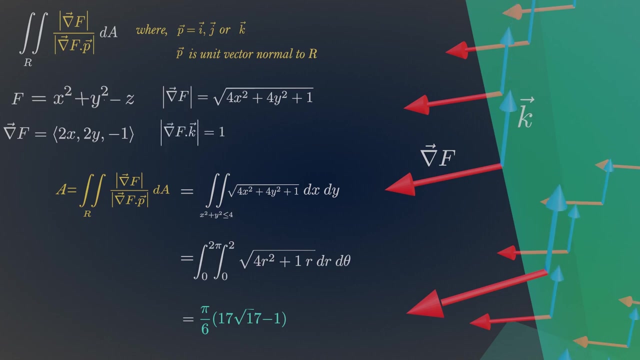 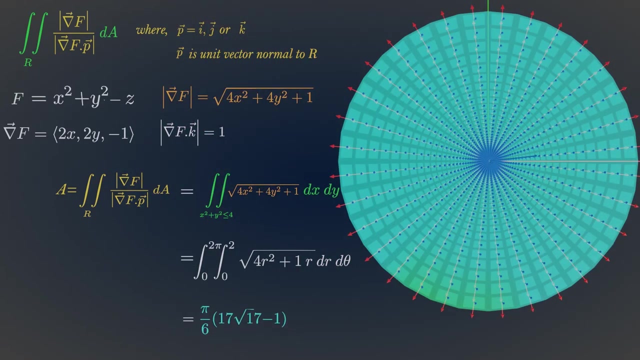 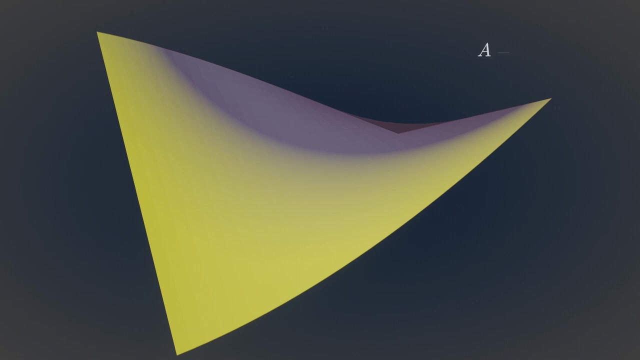 then the projection is one to one. in this case, unit p vector is equal to unit k vector, which is normal to our circle. now calculate the magnitude of gradient in the direction of unit k vector. finally, double integrate over the circle. the area would be same. now we can calculate the area of any surface by summing up each of these tiny patches of surfaces. 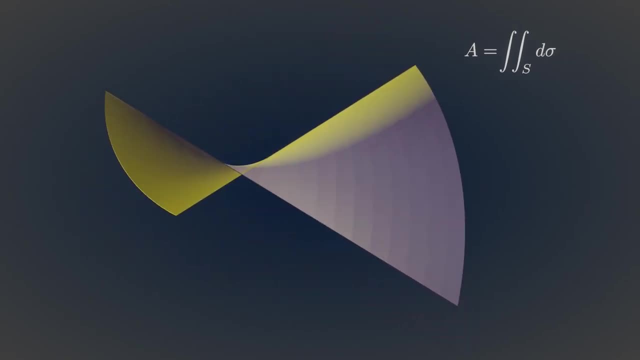 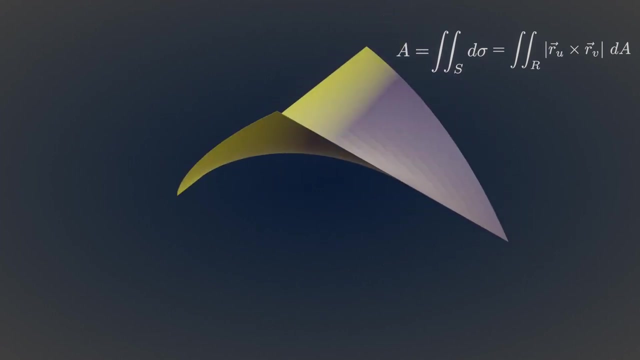 if the surface is parametrized, then we can unwrap the surface into a uv axis and double integrate the area of this plane. or if the surface is not parametrized, then we can convert it to an implicit function, project the function into the plane, capturing the built-in scenario. then, using the implicit method, we can 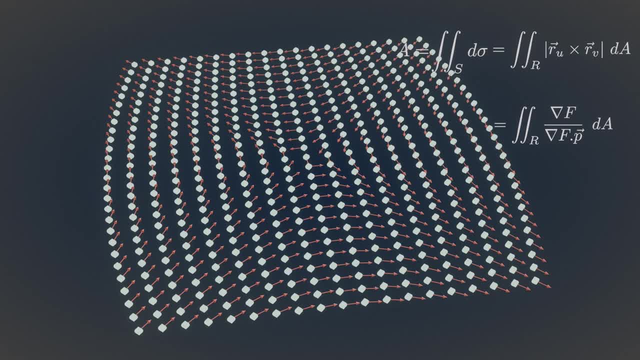 apply the boundary for each surface and then convert it to an implicit function, project the function into the plane capturing the area of the plane, so that you can see how this is its plot of the paraboloid plane. now we can its gradient vectors and compute the area by this formula. In both cases we evaluated the surface. 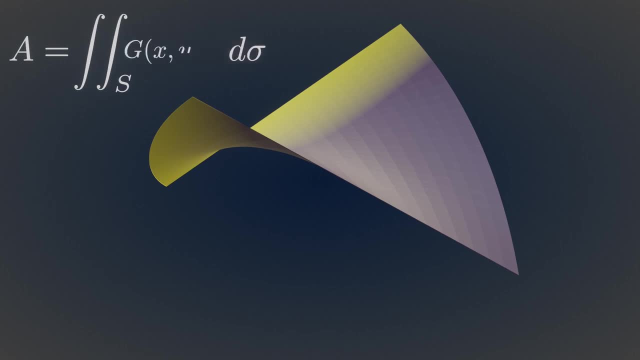 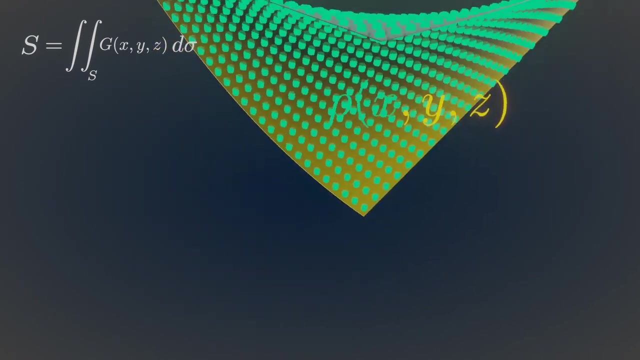 area. Now if you integrate a functions over the area of a surface, then what you are computing is surface integrals. For example, you might want to compute mass at each point on the surface. and if the mass per unit area on each point of a surface is given by this equation, 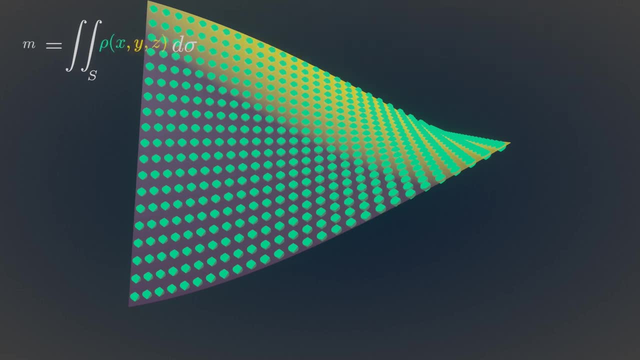 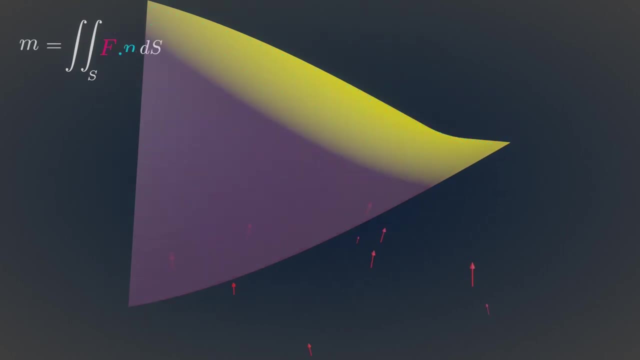 then evaluating this surface integral gives the total mass of this object. This is a scalar function. In this chapter we will focus mostly on surface integral of a vector field. Now imagine a fluid with velocity field flowing through a surface. Now think of this. 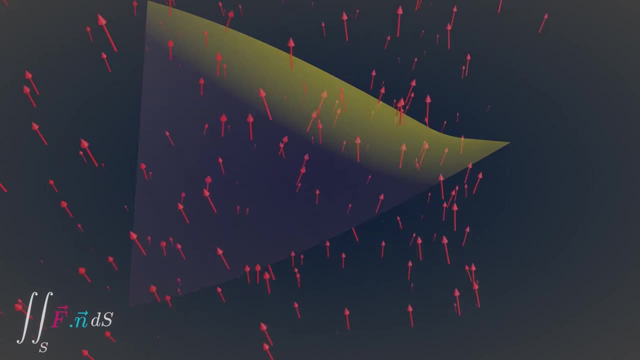 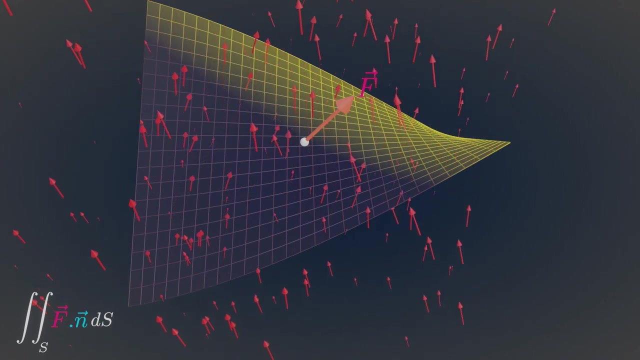 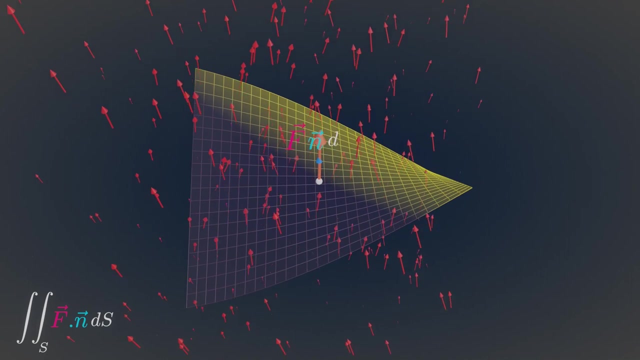 surface as imaginary surface which doesn't impede the fluid flow, like a fishing net across a stream. If f vector represents the velocity field and vector represents the unit normal, then the mass perpendicular to surface per unit time at an infinite small point is where rho is density. 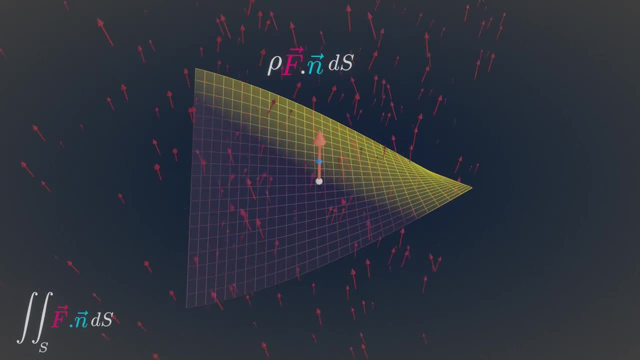 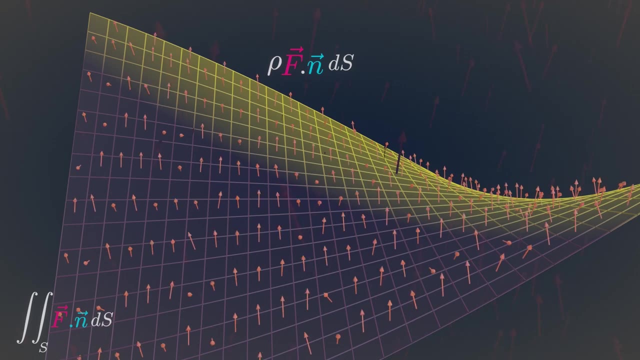 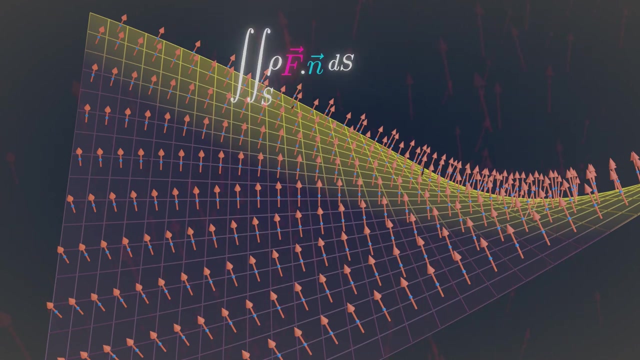 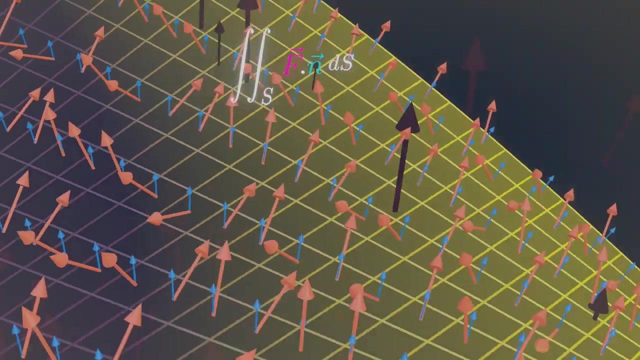 at that point This is interpreted physically as a rate of mass flow through an infinitesimal small surface. Now the flux of mass of the fluid flowing across the entire surface per unit of time is the surface integral of a vector field. The orientation of unit normal vectors is very important. If unit normal vectors 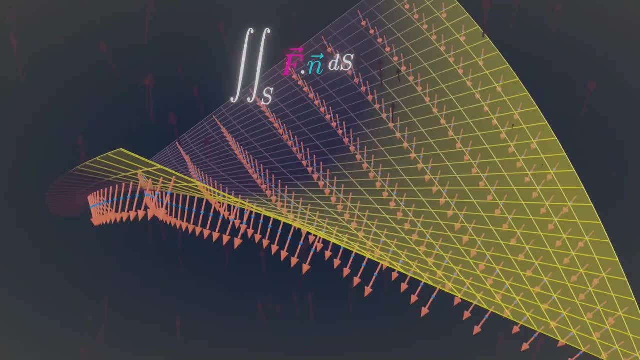 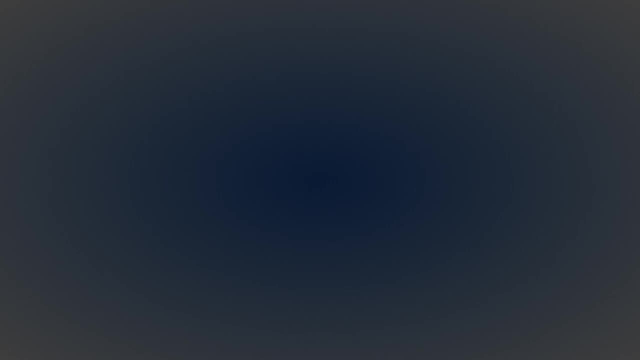 points in opposite direction, then we will be off by minus 1.. So we can calculate the surface integral of any vector field by using this formula. We already know how to calculate this differential patch element of a surface, But how do we calculate unit normal vector of a surface? 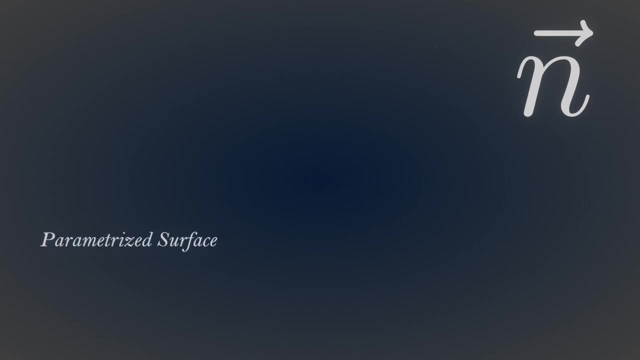 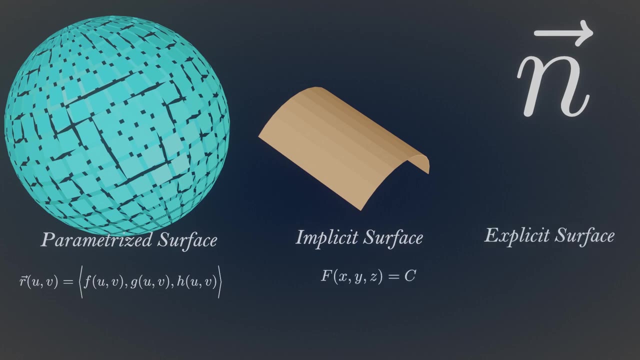 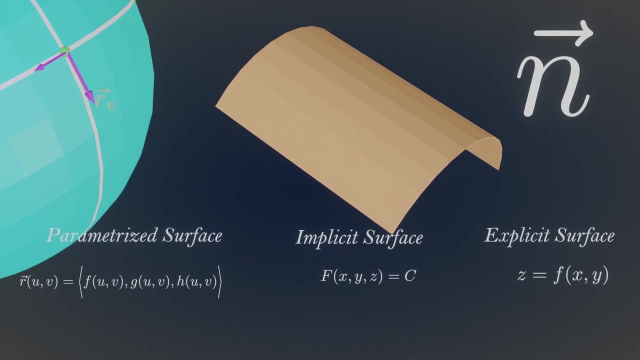 You might encounter three types of surface: a parametrized surface, an implicit surface or an explicit surface. For parametrized surface, the cross product of their partial derivatives gives a new vector perpendicular to the vector field. The cross product of their partial derivatives gives a new vector. 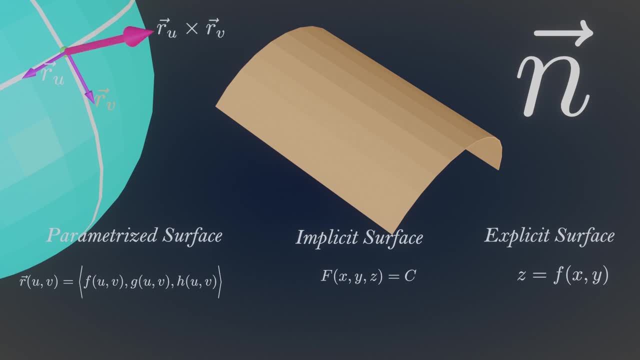 to their surface. so the unit normal vector for parametrized surface can be calculated by using this formula. Similarly, for an implicit function, their gradient vectors are perpendicular to surface, so the unit vector can be calculated using this formula. And finally, for an explicit surface, you can convert it to an implicit surface. 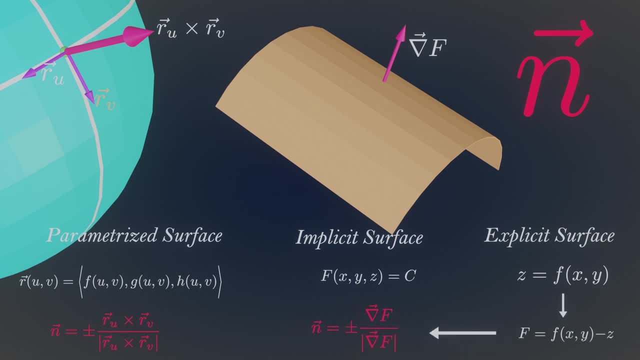 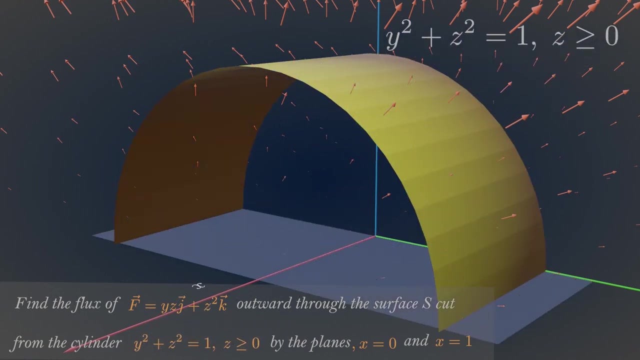 and calculate the unit normal. In the next episode we will evaluate the surface integral of a vector field. Let's calculate the outward flux of vector field through this surface which is cut from the cylinder by these planes. We can find the flux by this surface integral. 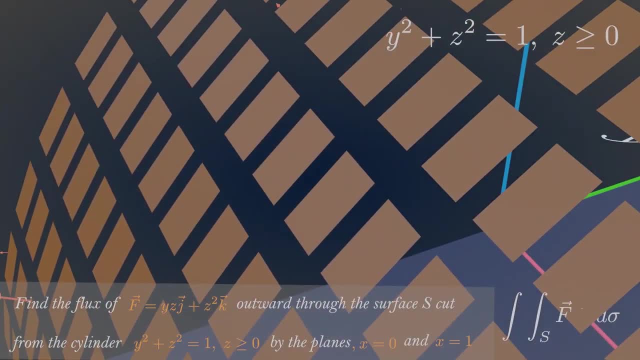 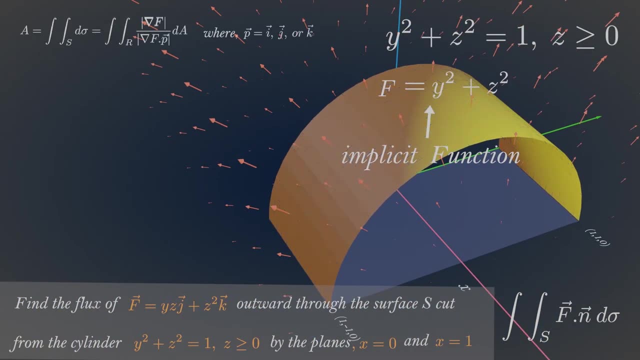 First, let's find the differential patch element of our surface. Since this is implicit function, we can calculate the flux by this surface integral. Let's calculate the area of this surface by using this formula. Comparing these two, we can see the differential patch element is It requires gradient of our implicit function. 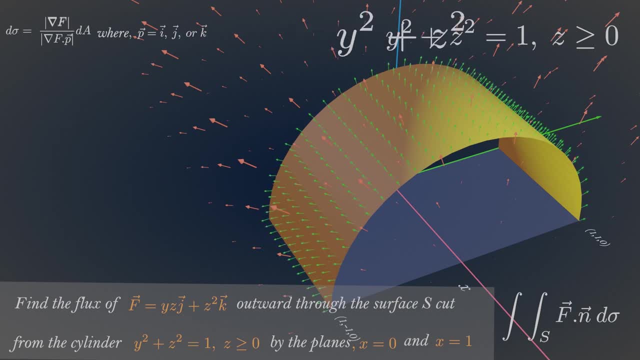 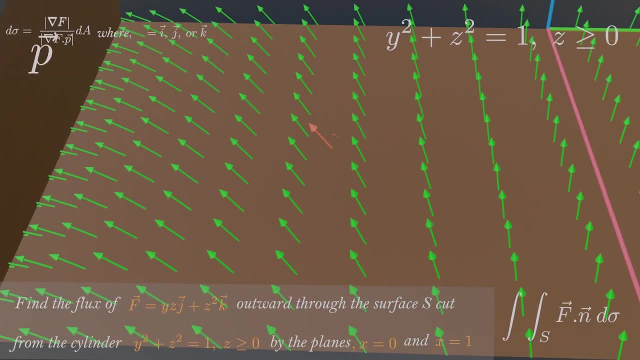 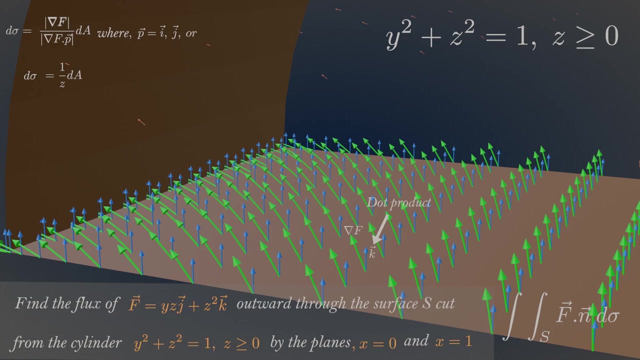 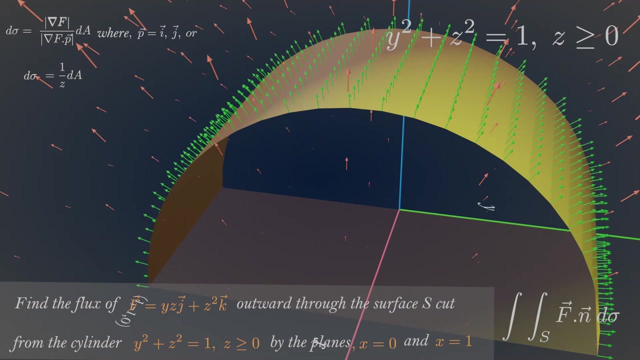 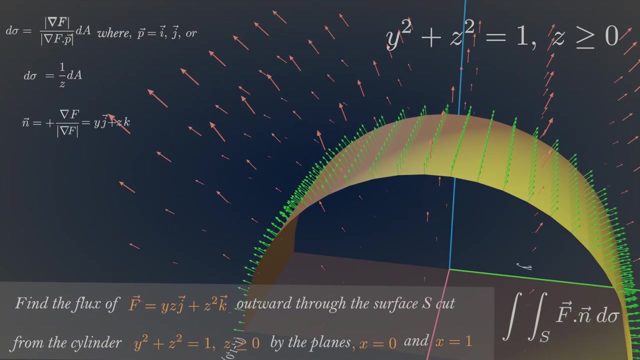 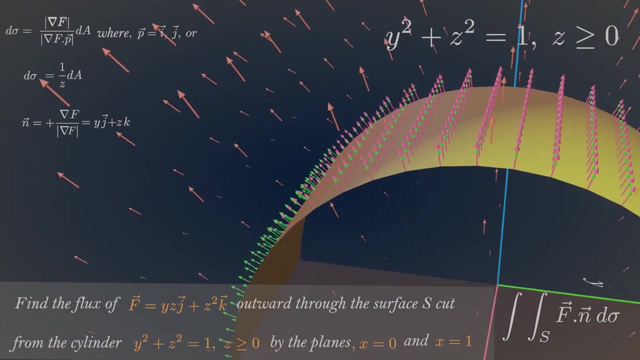 Okay, now calculate the gradient of this implicit surface. Now project the surface into the xy plane with its gradient vector. The unit p vector would be equal to k vector. Now calculate the differential patch element of our surface. Tell us the vector of this surface point on a pressure frequency: víinLife. 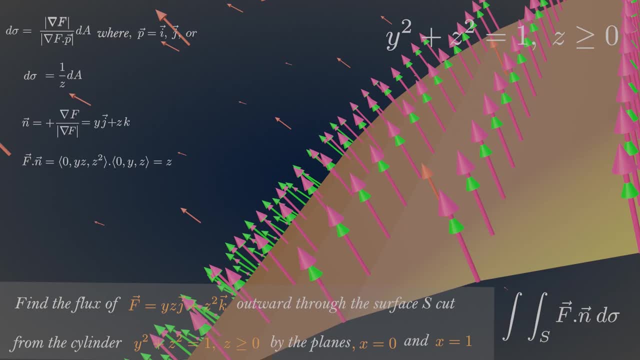 Now let's calculate the unit normal. Now the vector of the surface is direct outward. Now we need the vector field that acts on our surface. It seems the vectors are directed outward from the surface, so we want the normal that points in outward direction. Now we need the vector field that acts on our surface. It seems both unit normal and vector field points in the same direction, so the magnitude of flux in this case would be higher. 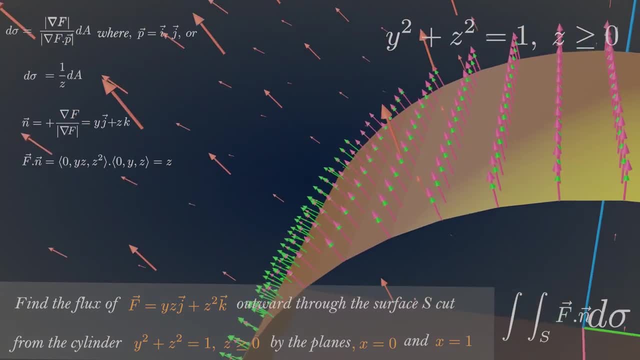 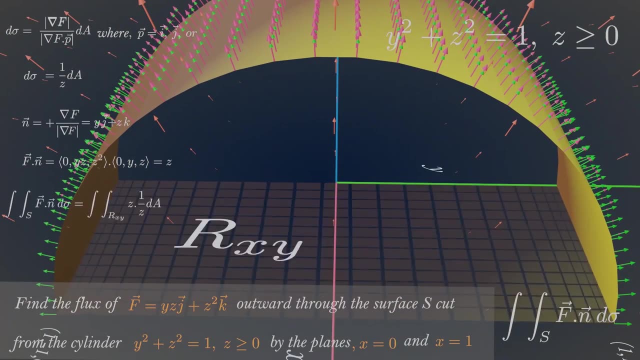 Okay, we captured that exterior andke chose to here. Will it work now? Okay, we captured surface patch elements and vectors in the direction of unit normal. Now evaluate the double integral over the region of this rectangle to get the total flux. 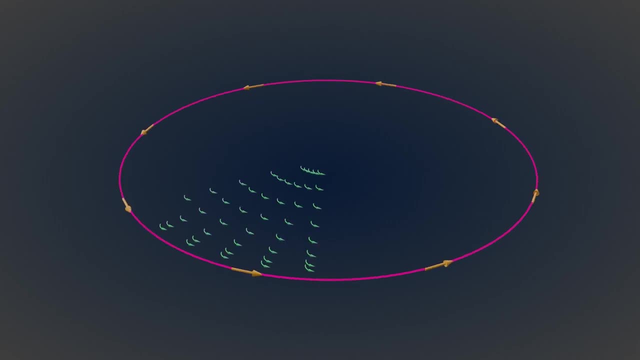 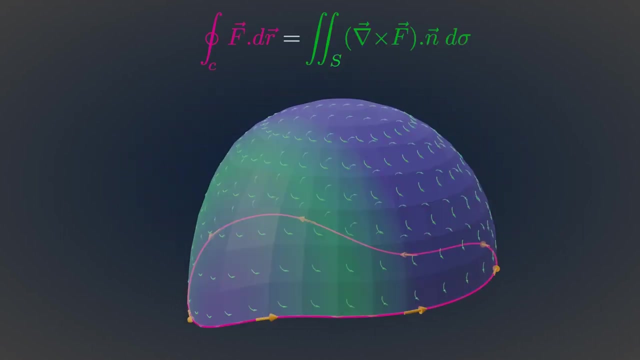 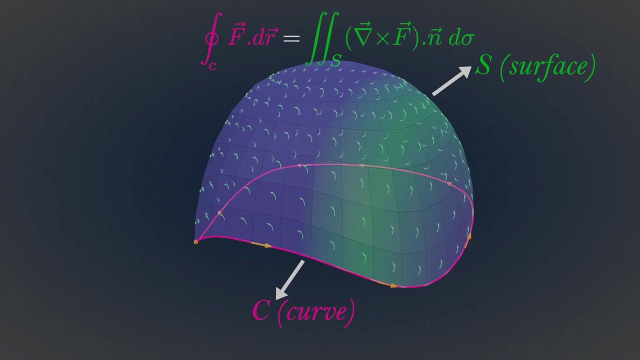 Now Stokes' theorem generalized the circulation curl form of Green's theorem to third dimensions. It relates the circulation of a vector field around the boundary C of an oriented surface S in space to a surface integral over the surface S. We also require that the surface 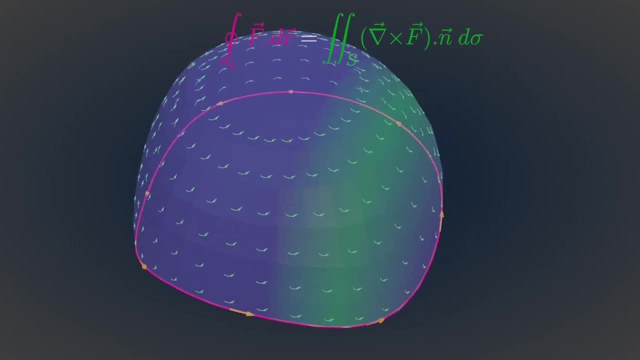 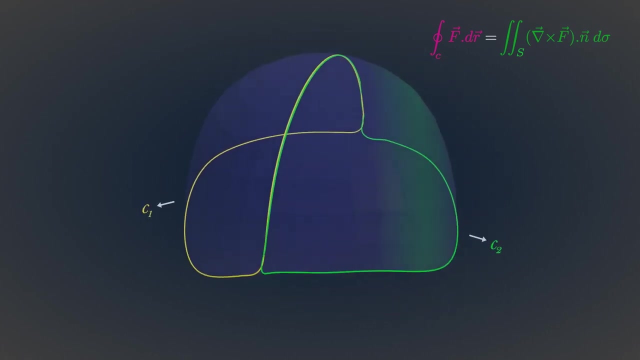 to be piecewise smooth. Now slice this surface in half And name the boundaries of the two resulting pieces. You can see these curves are oriented in counterclockwise direction. If they are each oriented the same way which our main curve was, then the line integrals. 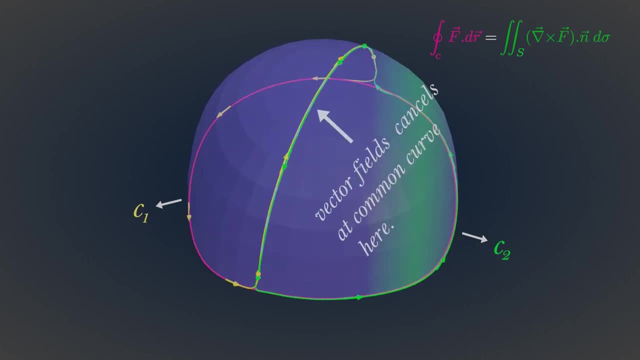 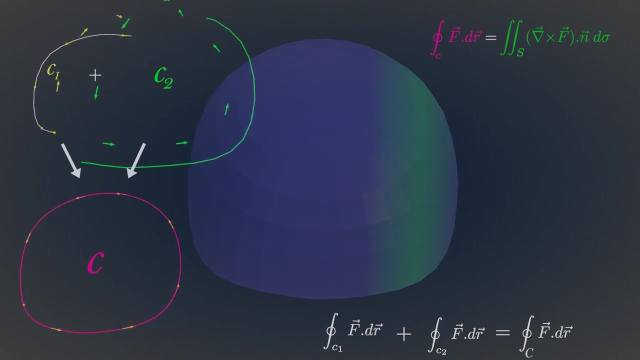 around each of these curves are the same. The smaller curves cancel out along the slice that you made. The portions of curve C1 and C2 which remains make up the original boundary C. So the sum of the line integrals around the smaller pieces equals the full line integral around our original. 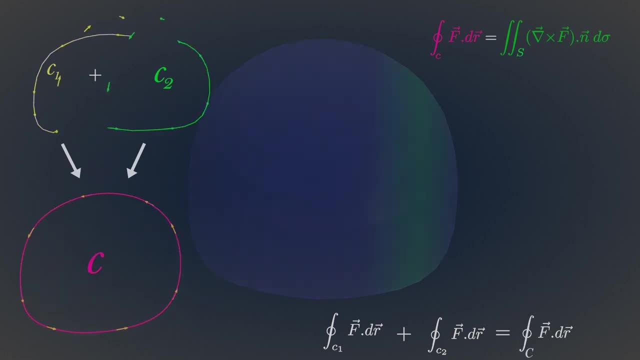 curve C. More generally, imagine slicing up these surface into many, many really small pieces. Now let's look at the curve C1 and C2.. We can see that these curves cancel out along the slice that you made And orient them all the same way. 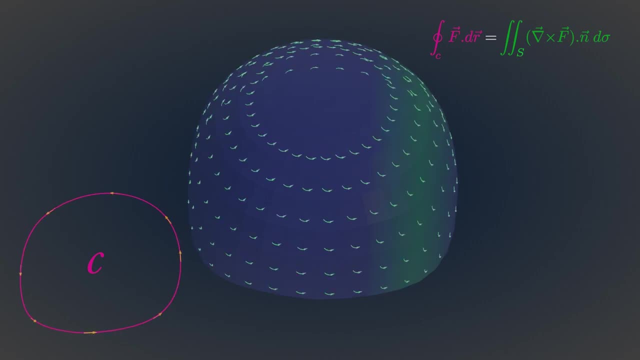 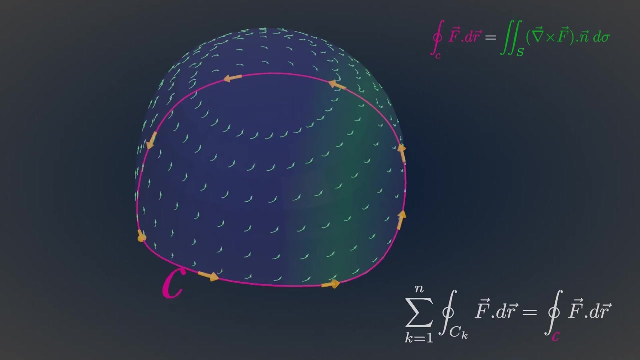 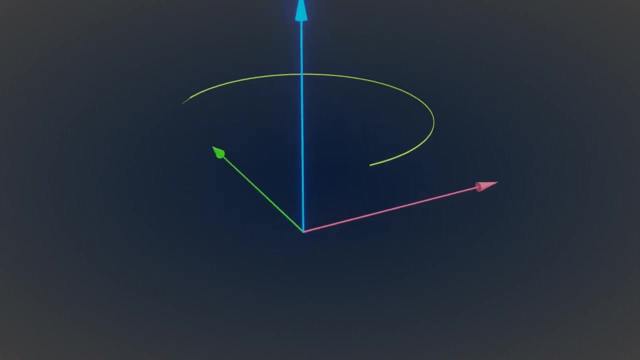 The line integrals around all of these little loops will cancel out along the slices within C, leaving only something equal to the line integral around C itself. Now consider a circle in space. Consider the orientation of this circle to be counterclockwise. Let the vector fields around the boundary of circle also rotates counterclockwise. 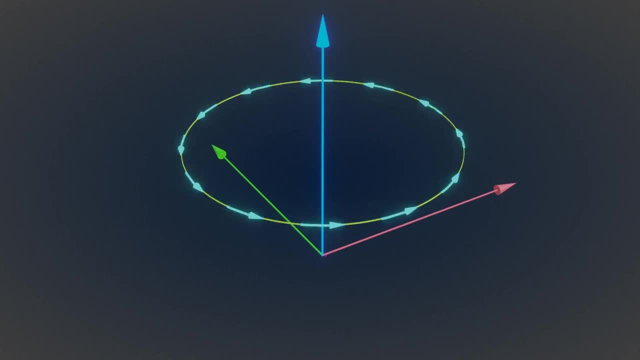 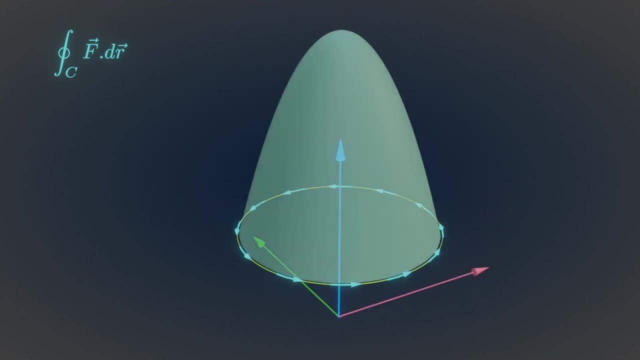 You can calculate the total circulation of vector fields around this circle by using this formula. If this circle is closed by a smooth paraboloid in 3D space, then according to Stokes theorem this circulation integral can be converted to curl integral In Stokes theorem. 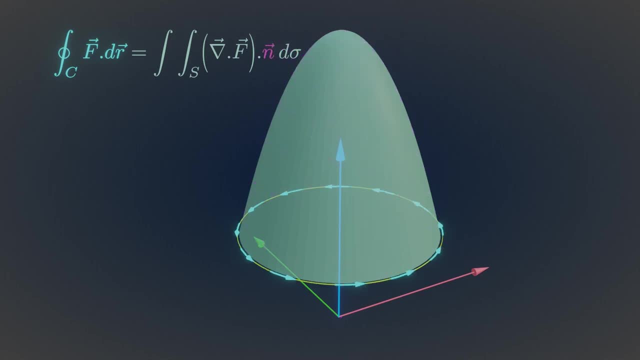 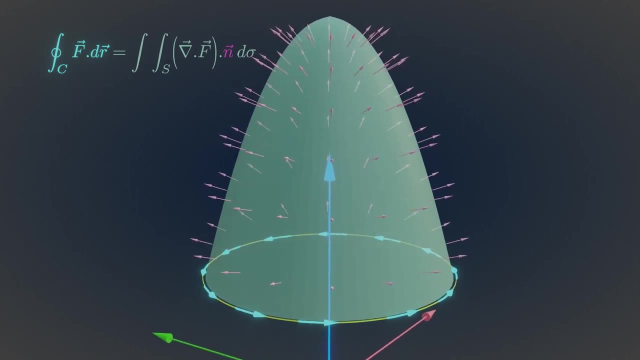 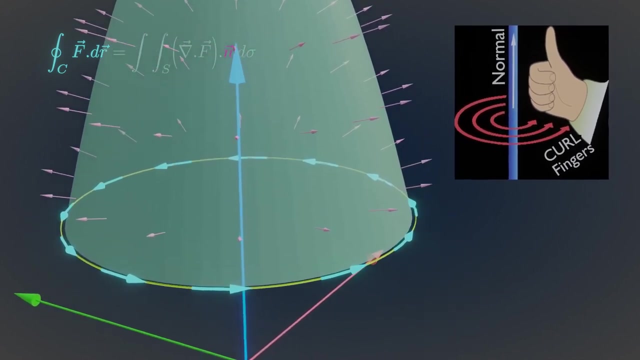 The orientation of surface is very important. You have two possible choices: either normal vectors points inward or it might point outward. The curve's orientation should follow the right hand rule, in the sense that if you stick the thumb of your right hand in the direction of a unit normal vector near the 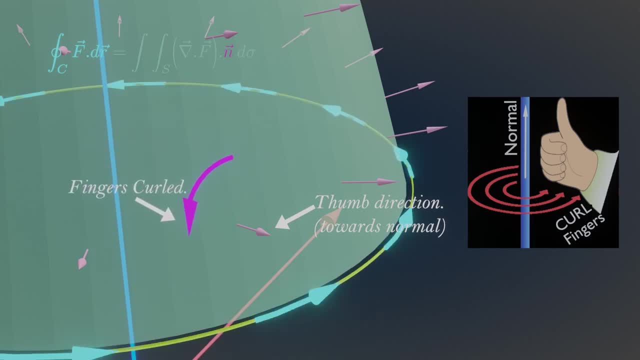 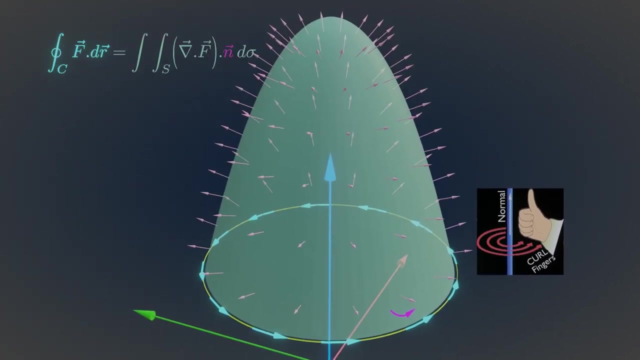 edge of the surface and curl your fingers. the direction they point on the curve should match its orientation. Here the orientation of curled fingers matches with the orientation of circle. so this is the right orientation of unit normal vectors. All of them must point outwards. 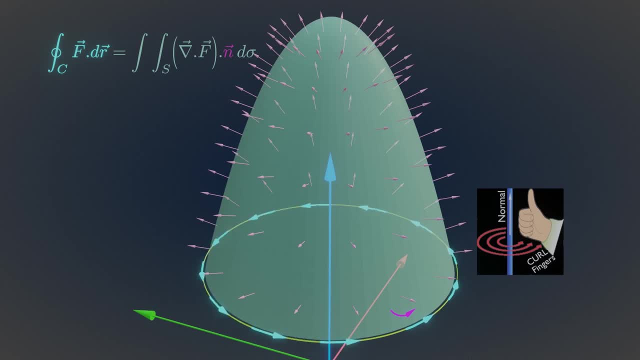 But if the circle is oriented counterclockwise in space and the unit normal vectors points outwards, then the direction of finger is in opposite with the direction of circle. Here the orientation of curved fingers matches with the orientation of circle. so this is: the right orientation of unit normal vectors, All of them must point outwards. But if the circle is oriented counterclockwise in space and the unit normal vectors points outwards, then the direction of finger is in opposite with the direction of circle. 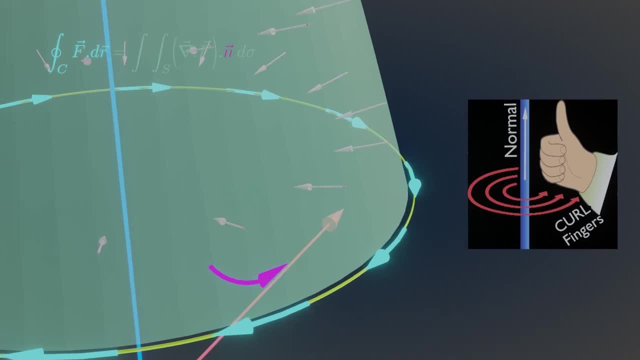 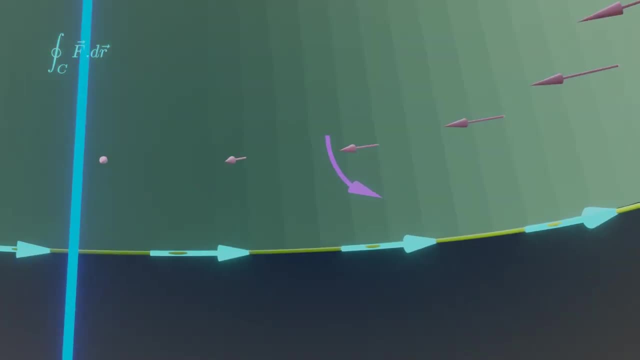 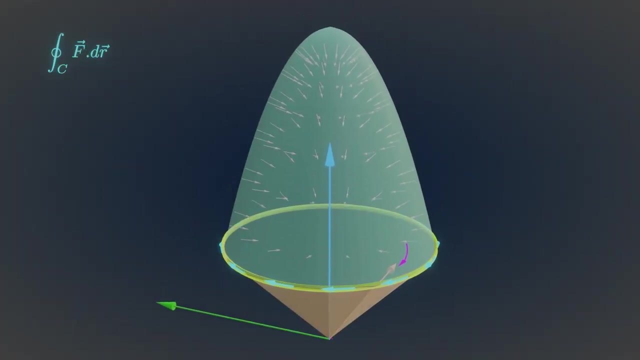 So in this case the normal vectors must points inward. So in this case the normal vectors must points inward. It is also possible that two different oriented surface can process the same boundary. Here the lower boundary is cone, whereas the upper boundary is paraboloid. 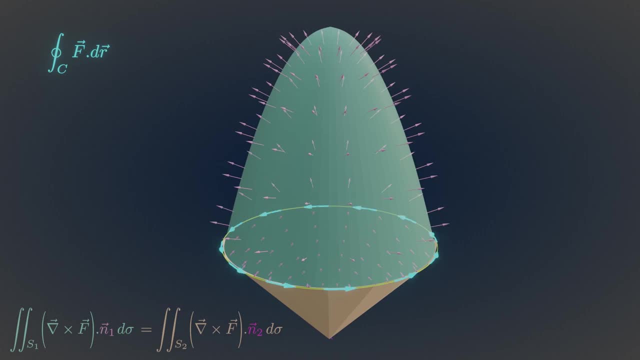 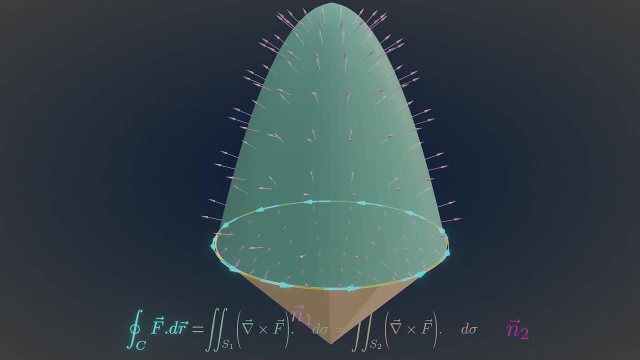 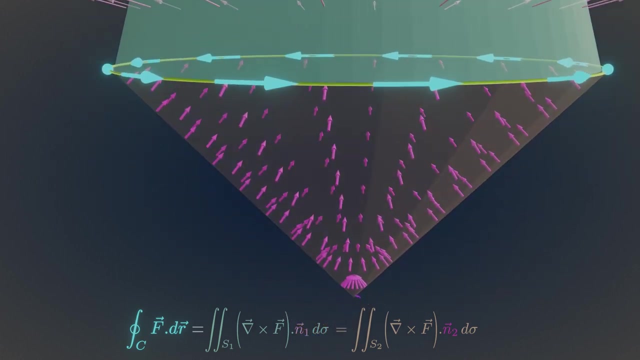 In both cases these integrals are same. In both cases these integrals are same. These both curl integrals are the same integrals equal the counterclockwise circulation integral on the left side of this equation, as long as the unit normal vectors correctly orient the surfaces. 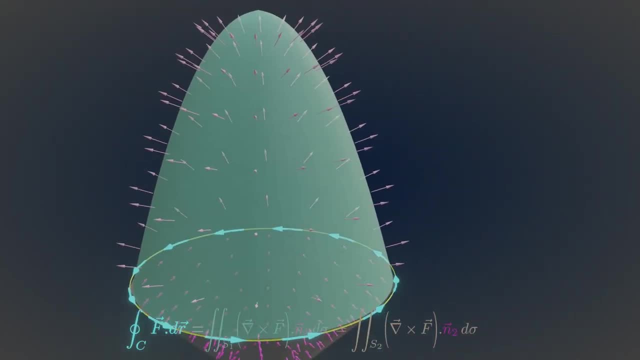 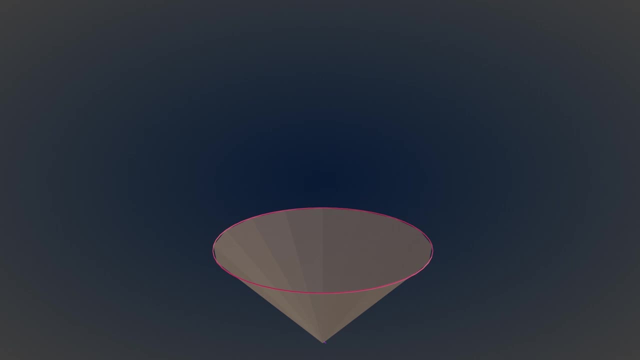 Just notice the correct orientation of unit normal vectors of cone and paraboloid. Now let's find out the circulation of this 3D vector field around this circle in space. This circle boundary is closed by a cone. having this parametrized equation, 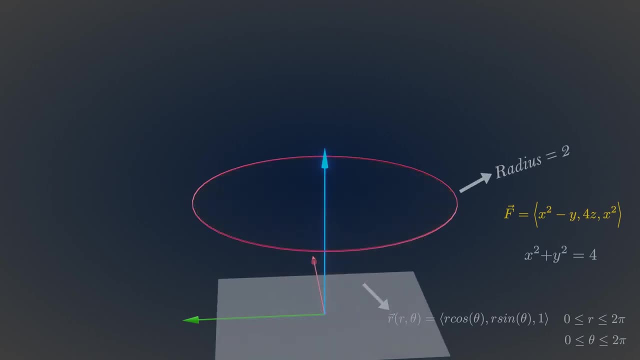 This circle has radius to unit and it lies above xy plane at z is equal to 2.. You can calculate circulation of this vector field around this curve by using this formula. Solving this integral requires a lot of work. Try solving it, you will get the answer of 4π. 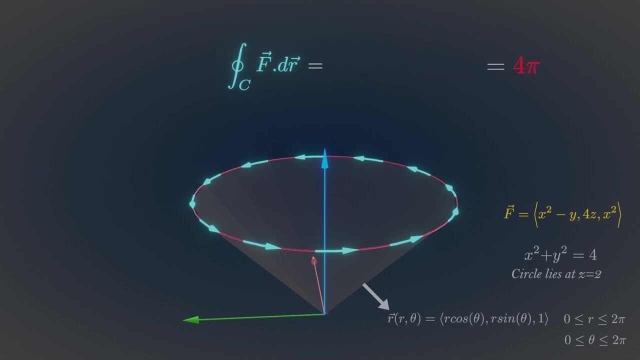 There is also another way You can convert this line integral to curl integral and integrate the curl field over the surface of this cone. Let's solve the surface integral for the cone, But for that first we need to get the normal vectors of cone. 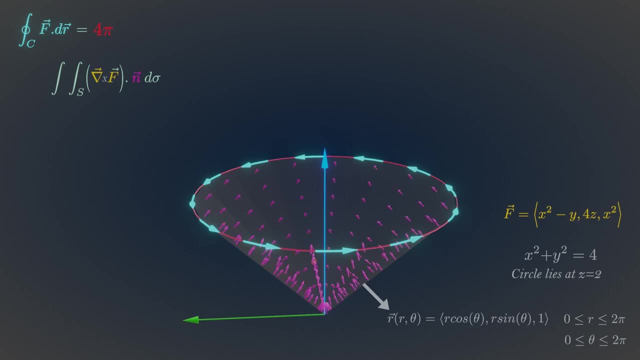 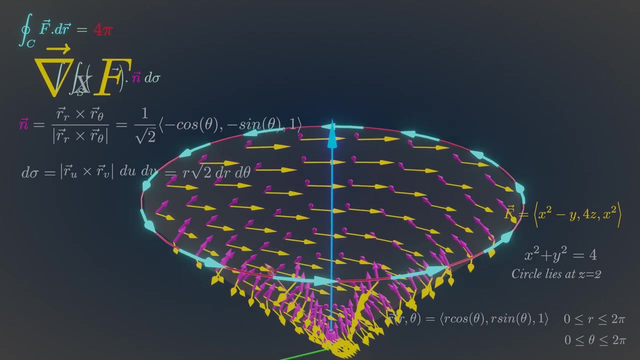 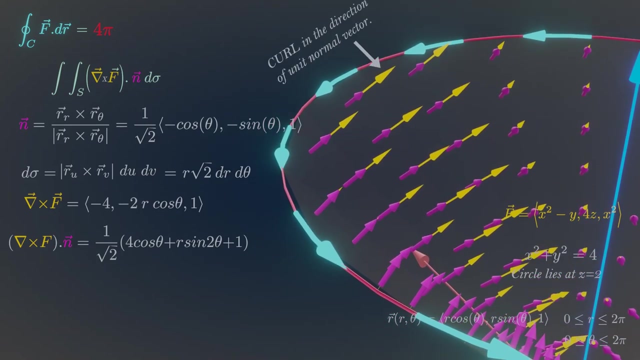 Since our circle is oriented counterclockwise. so according to our sign convention the unit vectors must be oriented in this way. Now get the surface patch element. Now get the differential equation of curl vector field. Now compute curl in the direction of unit normal vector, which is dot product. 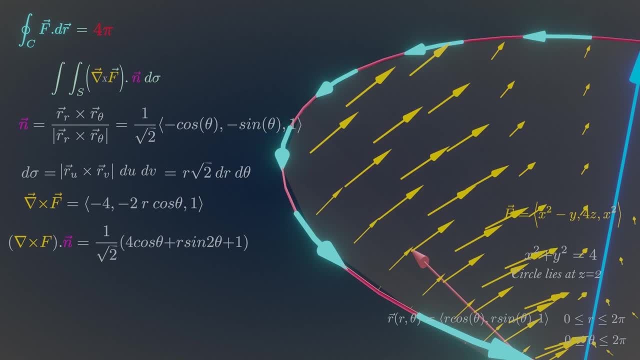 Finally integrate this magnitude of dot product over the surface of our cone? The answer would be 4π. The cone used in this example is not the integral. It is the integral of the surface of our cone. The answer would be 4π. 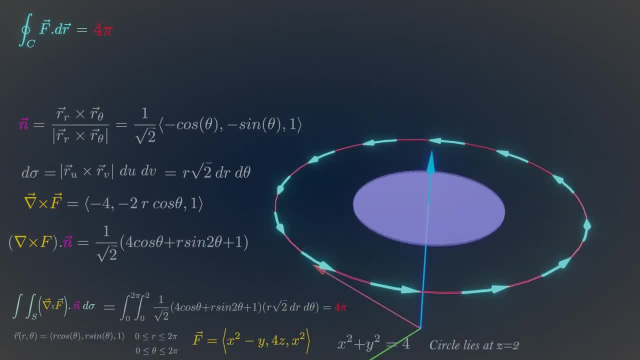 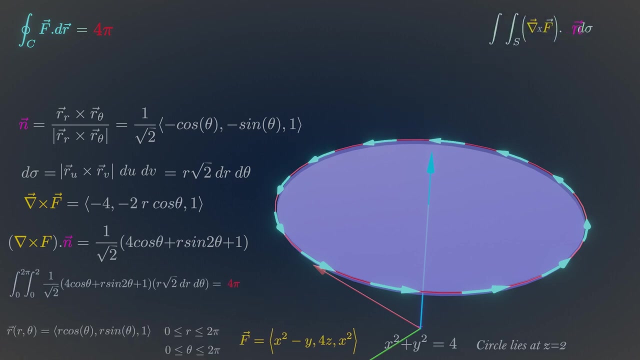 So we can use the flat disc of radius 2, centered on the z-axis. As the surface and circle lies in the plane, we can use Green's theorem To calculate this line integral. here the normal vector to the surface would be unit. 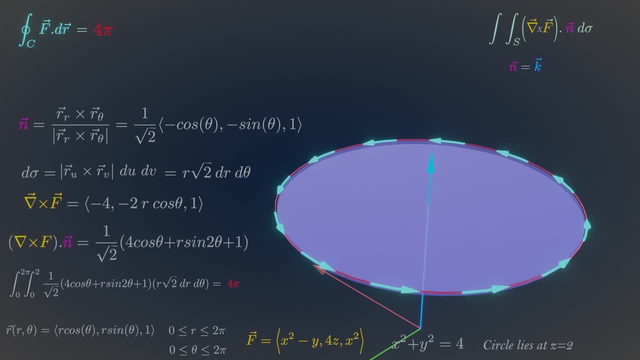 k vector. Now we still have the differential curl field. however, this component would be equal to 1.. So evaluating this surface integral would be equal to finding the area of this circle, which is 4π. This result agrees with the our previous circulation value. 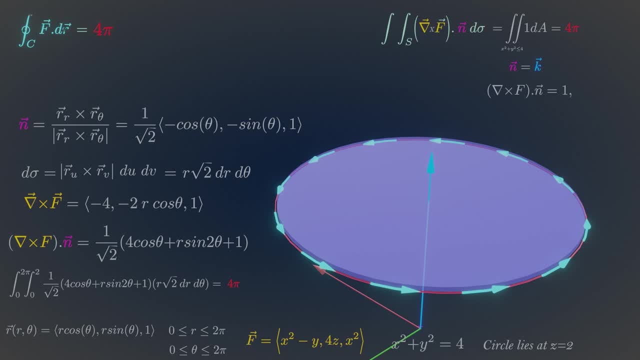 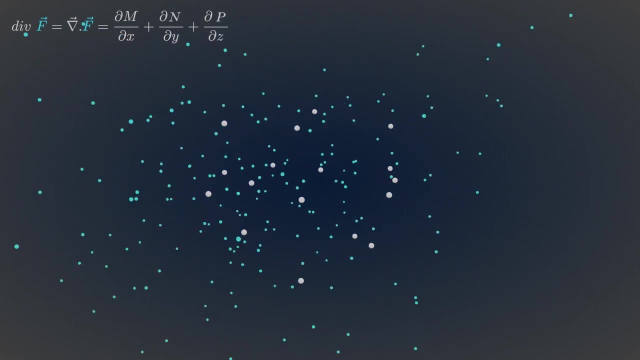 Similarly, the divergence of vector fields in third dimensions is written as: Now. if you integrate every of these divergence inside the domain of this circle, you will get the result. Now, if you integrate every of these divergence inside the domain of this circle, you will.